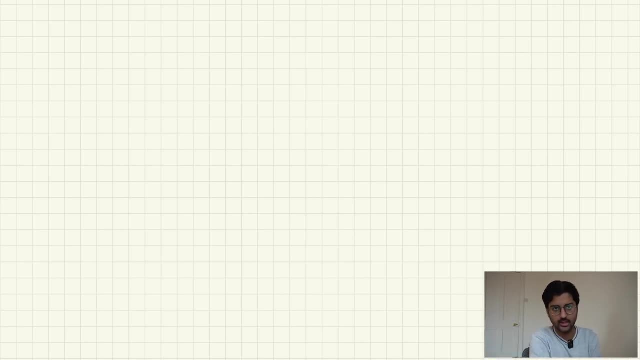 a very popular self-balancing binary tree. Obviously, we will look at other ones in the later on, but this is very important, Hence I am making a dedicated video on this. So we will look at AVL trees Full form. everything I will tell you later AVL trees- One thing: 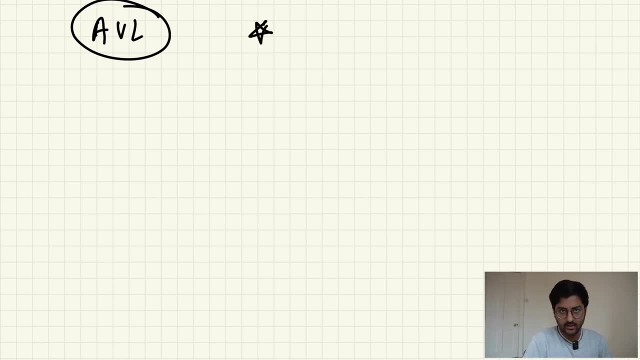 I want you to notice is sometimes people get intimidated by AVL trees. Oh, it's very difficult, you know, it's very confusing. It is not confusing. Not confusing, Then, what it is, Kunal It is actually. it has a lot of moving parts. 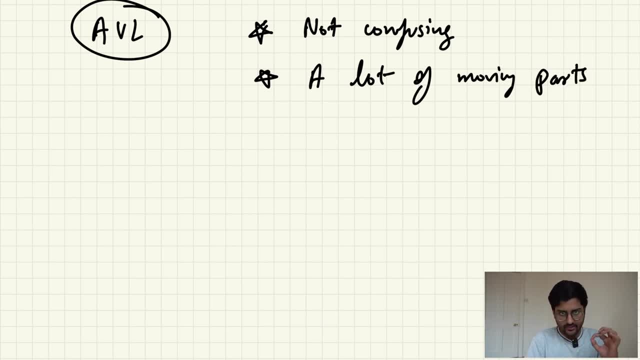 Lot of things are happening. So with AVL trees lot of things will happen. But all of those things are very simple. Just the quantity is a little bit. it's not that high. just four test cases. Okay, there are only four cases, but still some people feel like, okay, this. 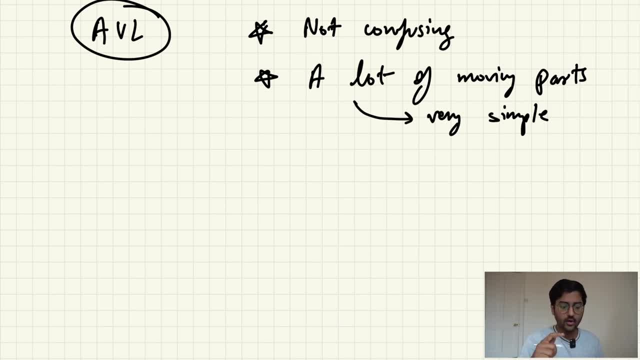 is too much, But I will actually teach you. So if you're looking at it for any topic, okay, not just tree. even when you do dynamic programming or when all the previous topics I've done in the past, when you take a concept and you try to memorize that concept in the 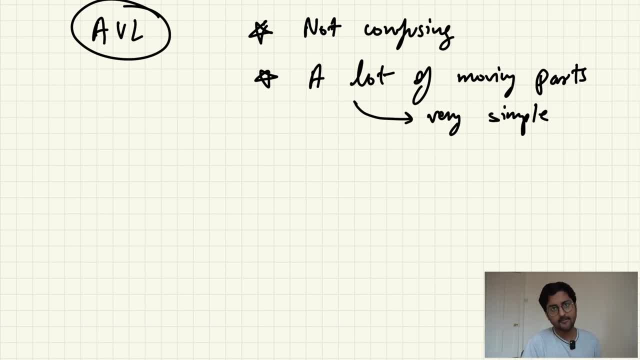 terms of: Oh, this concept has four cases, this concept has six cases, this concept has 10 cases. you try to memorize that without understanding what are these? Why are we having these many cases? Then it becomes overwhelming and difficult to you. Then you feel like it's difficult. 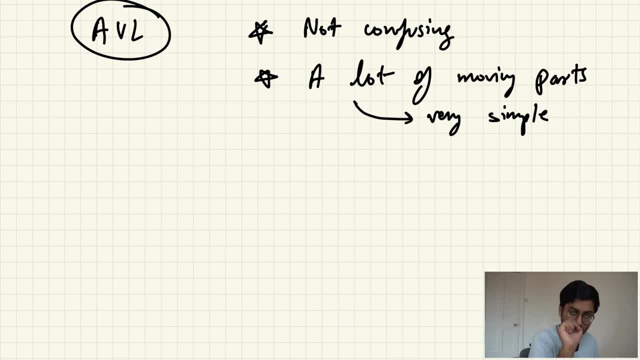 But I will make it clear to you why we only have four cases. What is the significance of each case, The thought process behind it? When they created AVL, why did they only make four cases, or whatever? Okay, let's get started. Forget about AVL right now. Let's just talk. 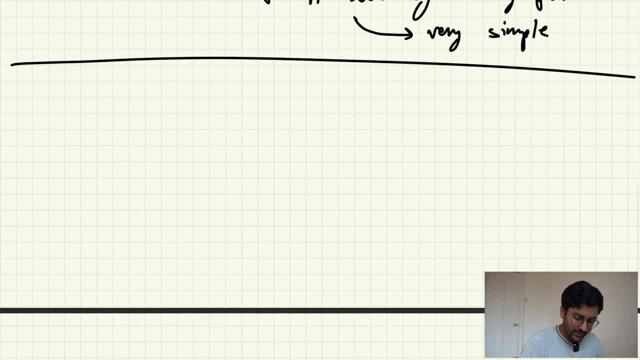 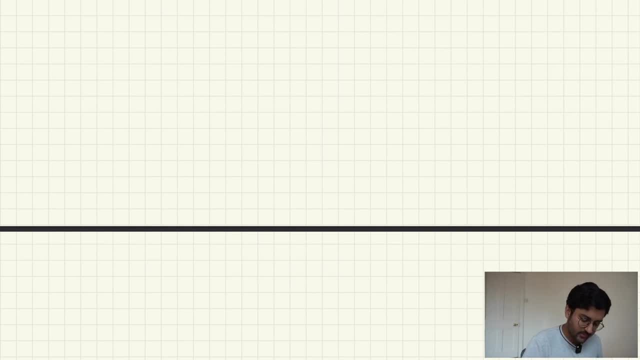 about binary trees, normal binary trees. So if I talk about a normal binary binary search tree, in the previous video we have already learned how normal binary trees functions. Okay, Let's say I have 10 over here And now I'm saying: Hey, Kunal, insert five into it. Okay, 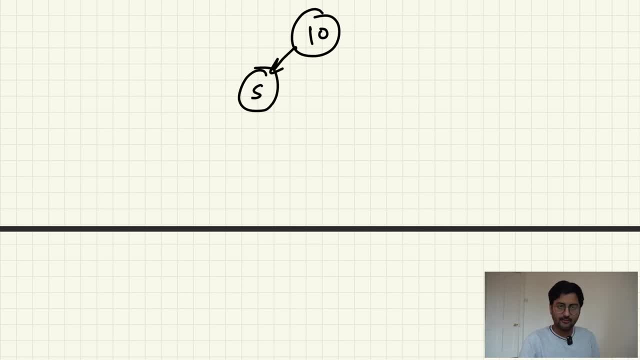 five is smaller than 10.. I will go over here. I've already covered this. Okay, how binary search tree functions. So if you're not understanding this, please watch tree tutorial number one. there's a there's a tree playlist on my channel. Now insert 15.. Okay, 15 will go over here. 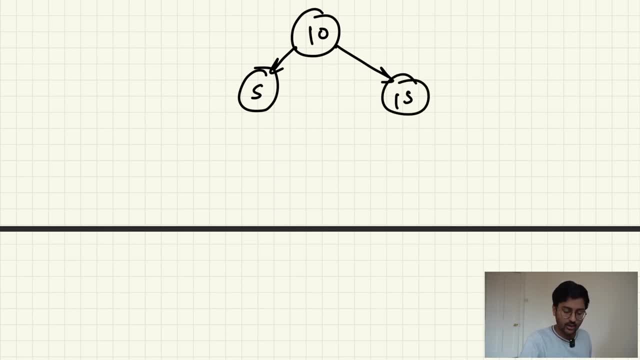 Now insert 10.. 10 is already there, now insert 12.. So 12 is greater than 10.. So right hand side 10, 15, left hand side, So on and so forth. you get the idea. So the idea is that the 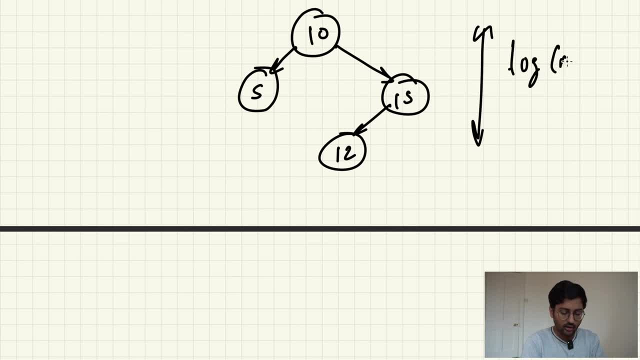 maximum height. let's say it's going to be log of n, which is n is the total number of nodes. So at any point of time. we have already covered in the past how the insertion and your delete and your, you know your when you delete, or one when you try to search an item. 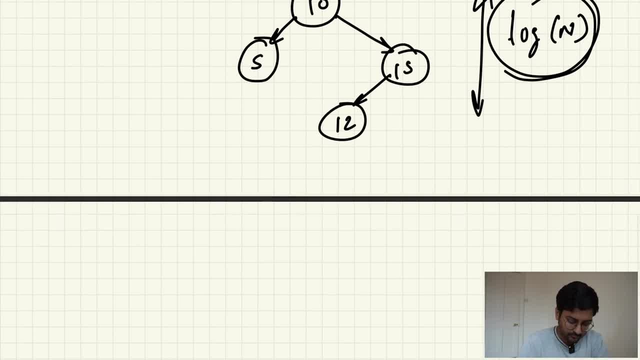 it will take log of n time. Very good, No problem, Okay. But the problem arises. let's say you're saying: Kunal, insert five in a binary search tree. Okay, no problem. So let's say you're saying: Kunal, insert five in a binary search tree. Okay, no problem, Okay, no problem. 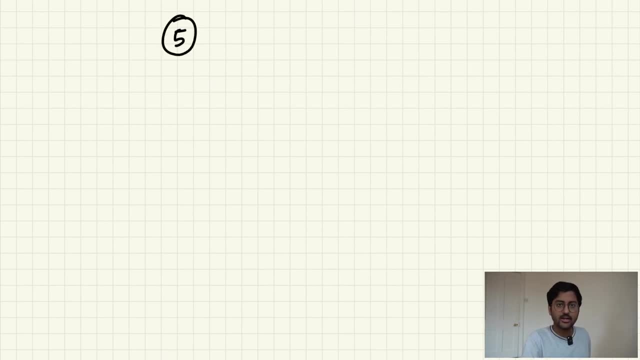 Okay. so let's say you're saying: Kunal insert five in a binary search tree, Okay, no problem, I've inserted five. Now Kunal insert seven into it. Okay, so five is seven is greater than five. it will go on the right hand side. No problem, Kunal insert nine into it. Okay. 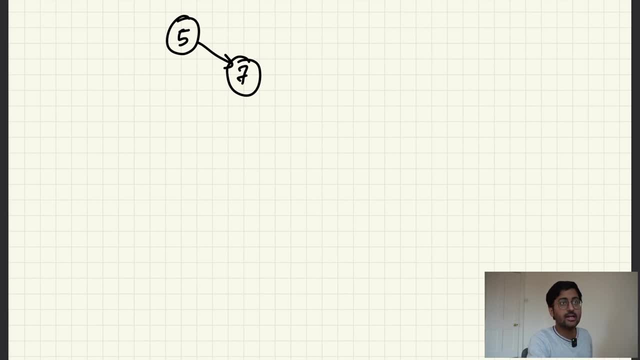 Nine is greater than five, So it will go on the right hand side. Nine is also greater than seven. It will again go on the right hand side. Kunal, please insert 11 into it. Okay, 11, I will insert over here. Kunal, please insert 13 into it, Okay. third, So can you. 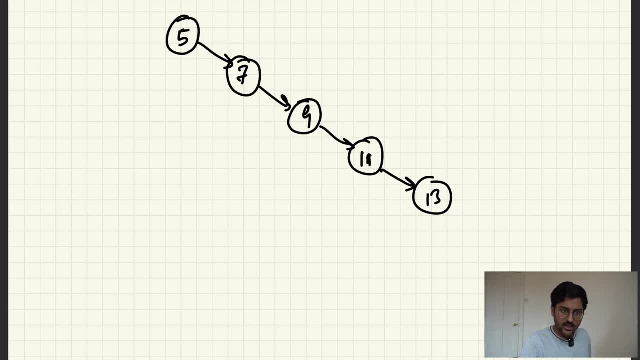 see what is happening. If I want to search 13,, it will have to insert 13 into it. Okay, 13,, it will have to traverse it n number of times. So instead of log n, it is now taking n complexity, which is wrong. Whole point of binary trees is now destroyed, Whole point. 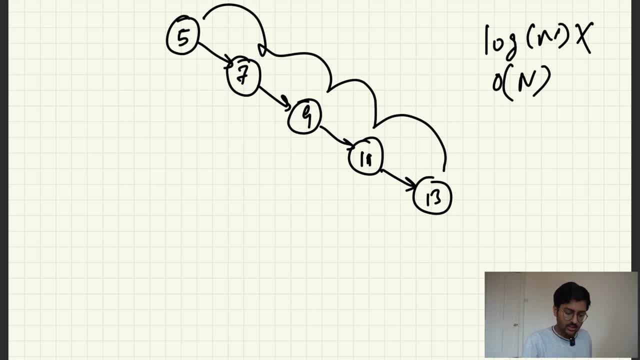 is destroyed. This is the problem with binary search trees, Because a chain can form like this. Even if you have something like this, still there is a chain right, Not perfect. log n is the answer. Make sense. That is the problem, and 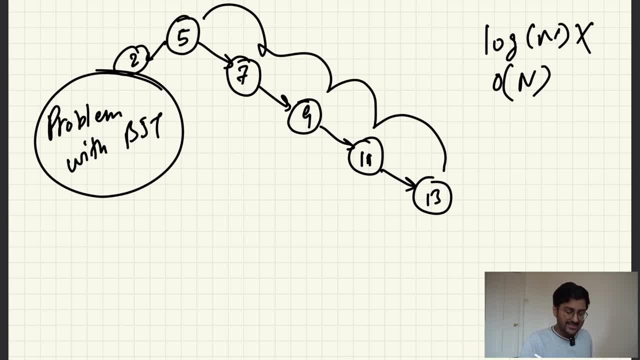 that is what we're trying to solve. So how do we define this problem? Okay, now defining the problem Kunal. it looks like a problem when I'm looking at it from my eyes, But how do you define it in a definition? 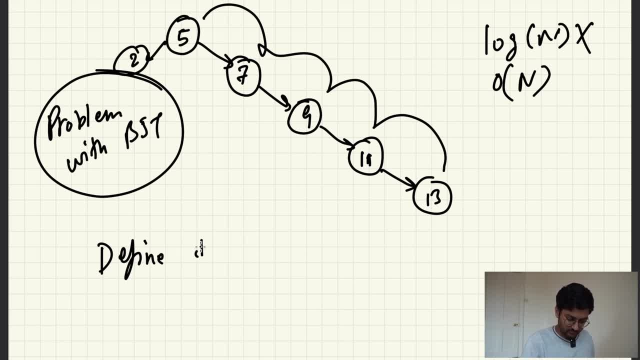 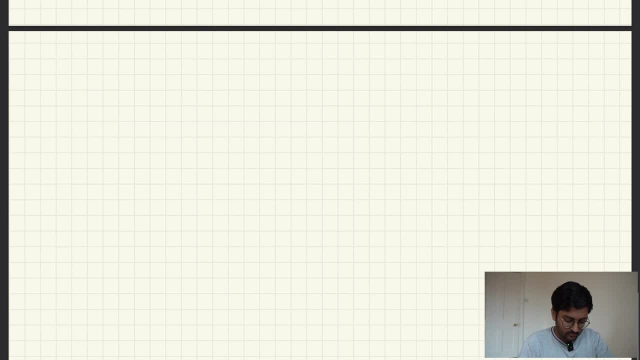 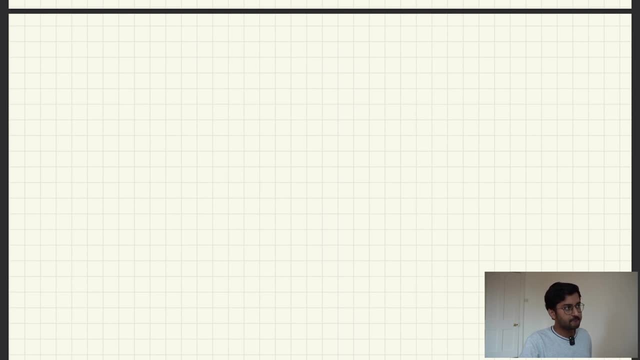 Define the problem. No problem, we can define it. So the problem is this: that for any tree, for any tree that you have, let's say we have this tree, Something like that. Okay, Let's say we have this tree. Now here you can see that the difference. 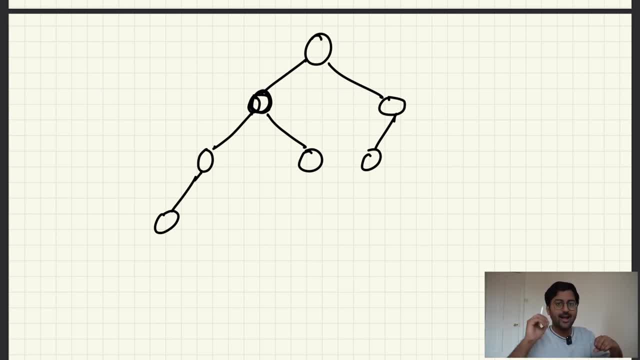 of height of left subtree and right subtree, for every single node is going to be either plus one or minus one, like less than equal to one, for example. So here you can see what is the height. Height is the number of edges from the node to the 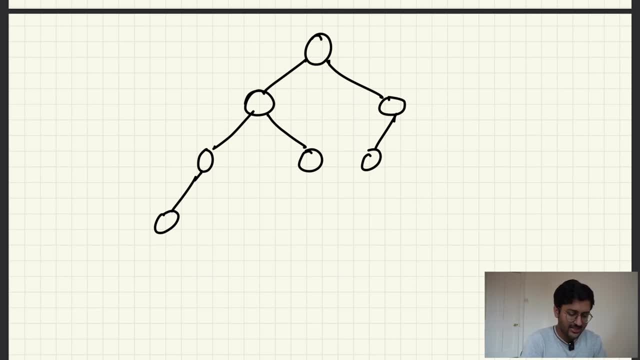 bottom leaf. So for every single node, let's say we're talking about this node first. for every single node, Think about the definition. For every single node. the height of the left and the right tree should not have a difference of more than one. Okay, what is the height? 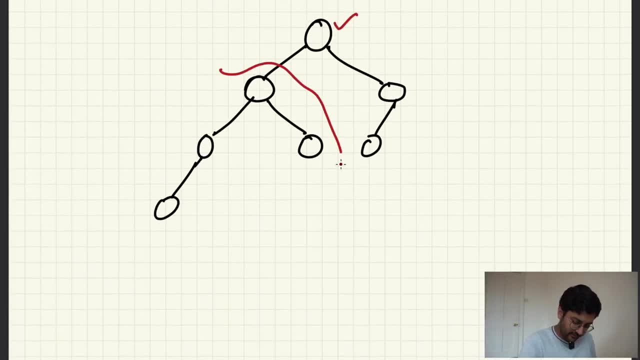 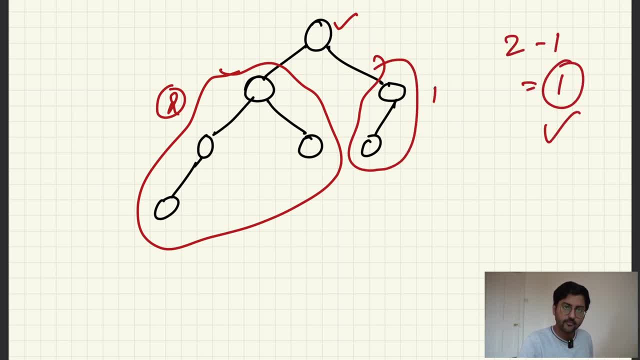 this one: 1.. 2 minus 1 is equal to 1.. Correct, So this difference should only be less than or equal to 1.. So 1 or 0. And if you do, let's say, for example, if I say for every: 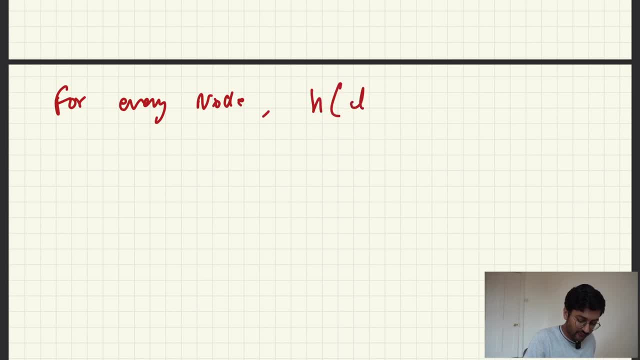 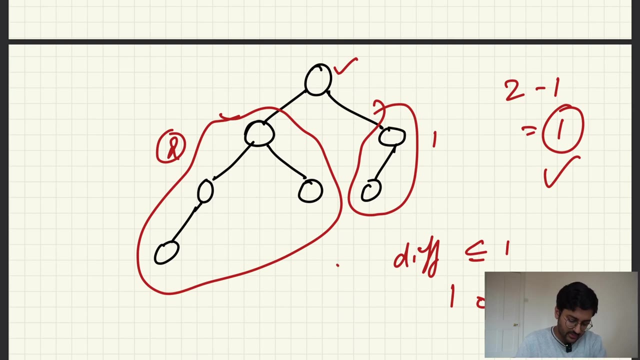 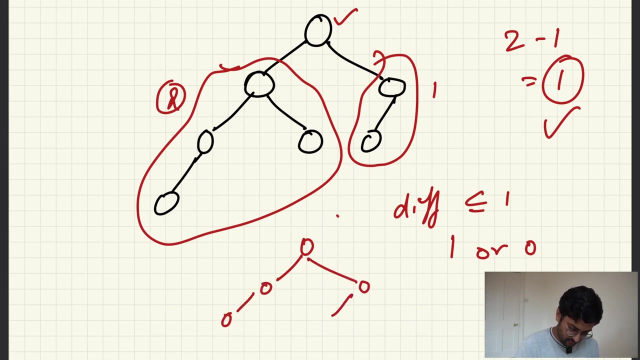 node. height of left minus height of right can be equal to minus 1,, plus 1, or 0. only In this case it is 1.. But if you have something like this, in this case this height is 1,, height is 2, for this tree or this tree. 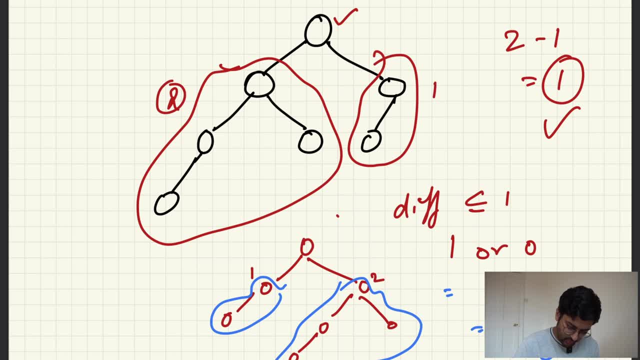 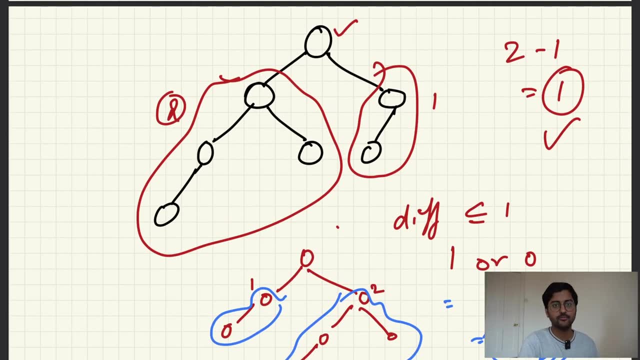 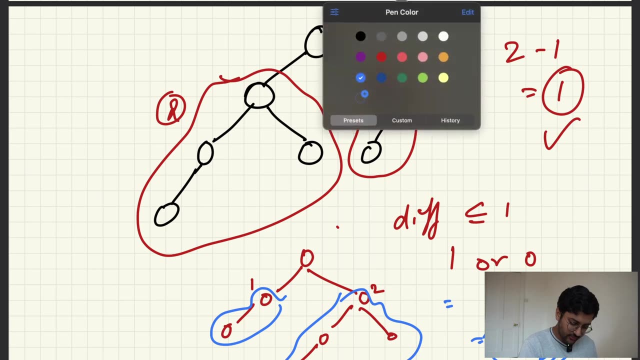 1 minus 2, minus 1.. That's fine, No problem. Okay, And this you have to do for every single node. For every single node, you have to do this. So now, let's see, I did it for this node. right Now, I will do the same for this node. 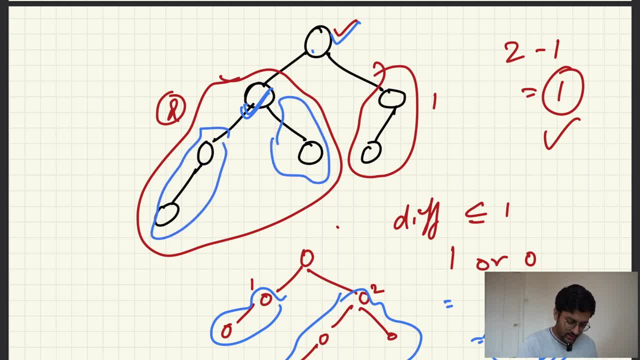 So again, take this tree and this tree. Here the height is 1.. Here the height is 0.. Difference is 1 minus 0, 1.. Yeah, sure, This is also balanced. Now again, do for this node. 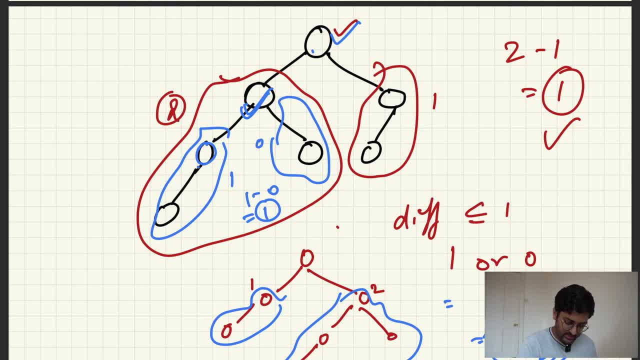 For this node: 0. And so this is just 1.. So I will just leave it For this node. this is itself. it has no left or right children, So I'll leave it. And for this one it's again just 1,, as you can see over here, 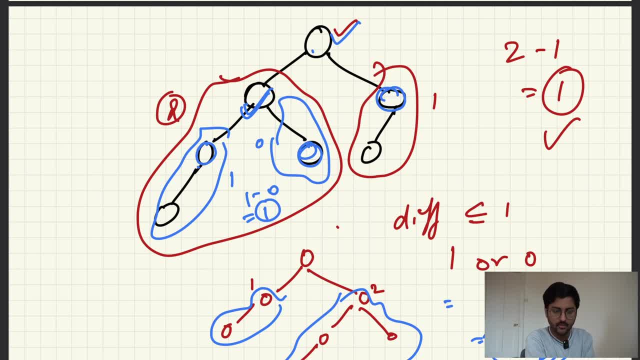 So pretty simple stuff, Okay. So, as you can see, for every single node- I'm repeating it again and again- For every single node- the left and right tree height can only be minus 1,, plus 1, or 0. 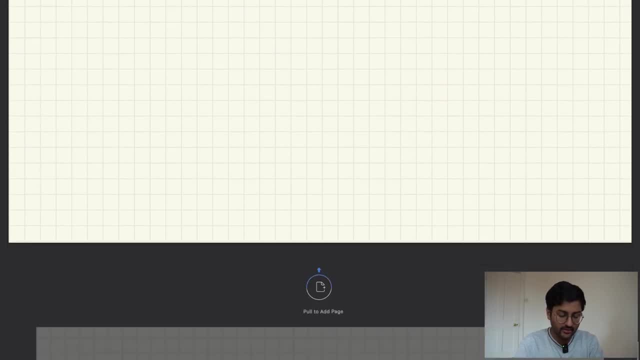 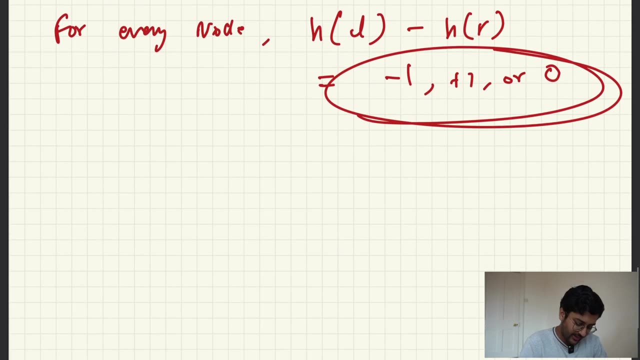 Let me take an example of a tree which is not balanced. This is known as a balanced tree. By the way, Okay, If I write the definition down for every node, did my pen run out of ink Not working, So actually this is the definition only. 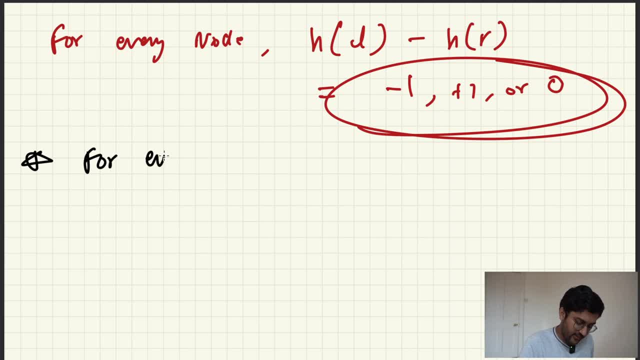 What formula I have just written above. For every node in the in the tree, the difference in height of left and right subtree of that node for every node should be less than equal to 1.. Or, yeah, should be less than equal to 1.. 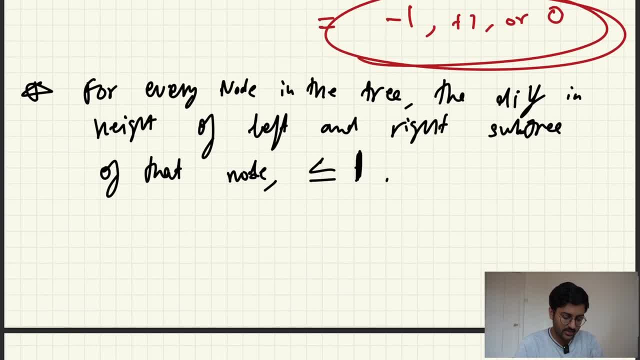 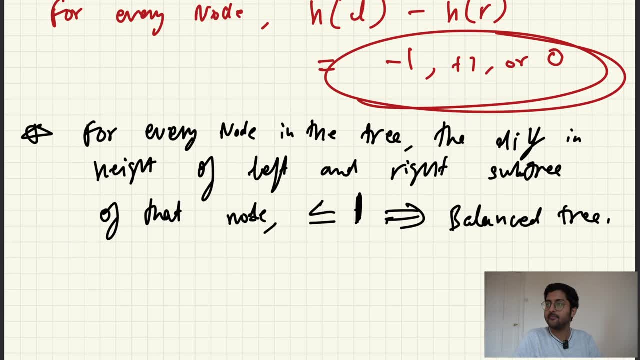 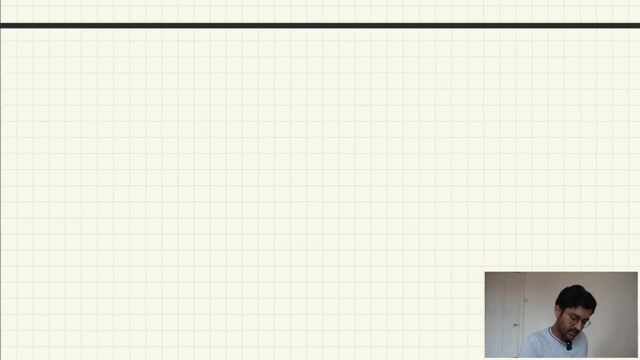 Cool, So either 1 or 0.. Now let's take a look at an example and that is a balanced tree. That is called a balanced tree. Let's take a look at a tree which is not balanced. So if I have this tree right here, okay. 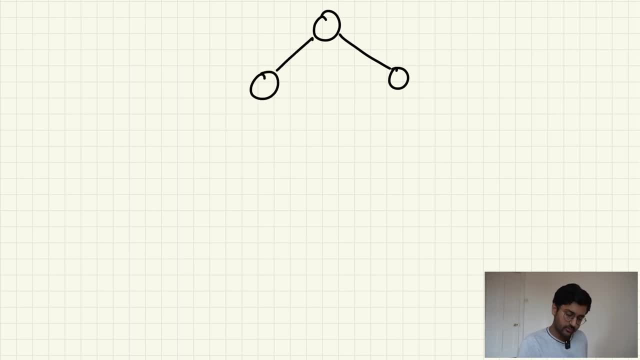 Like this: This is okay for now. Something like this: Fine for now. Okay, Let's add in one more. Okay Now, how do we determine, Kunal, whether this is a balanced tree or not? Look at the definition. 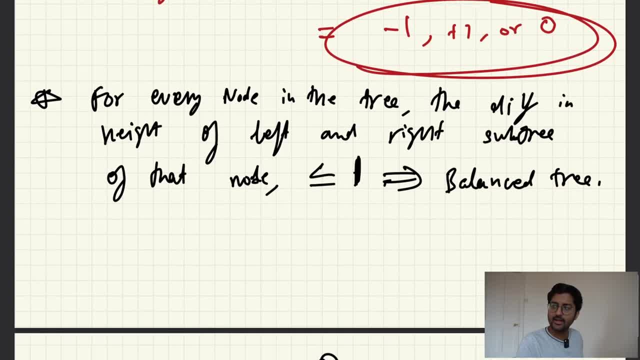 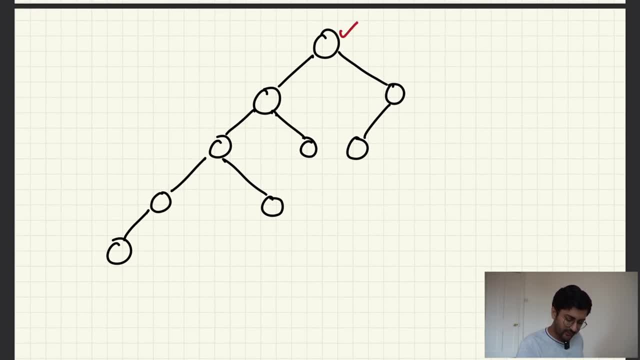 The definition says, for every node in the tree, the difference of the left and right subtree height should be less than equal to 1.. Okay, Then I will start checking from here. What is the height of left and right? So height of this is 1,, 2,, 3, and height of this is 1.. 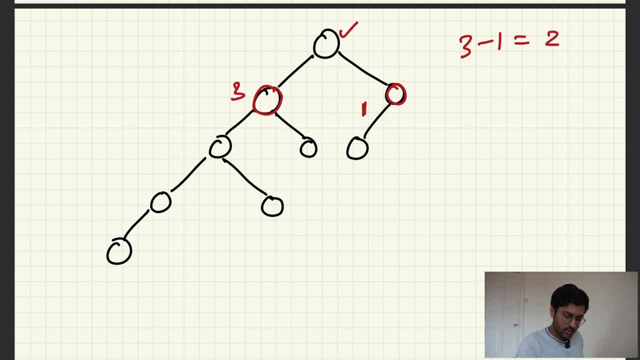 So 3 minus 1 is equal to 2.. Not balanced, Not balanced Simple. That is basically balanced tree and unbalanced tree. I hope that is clear, Okay, In the previous example also, this is also unbalanced tree. 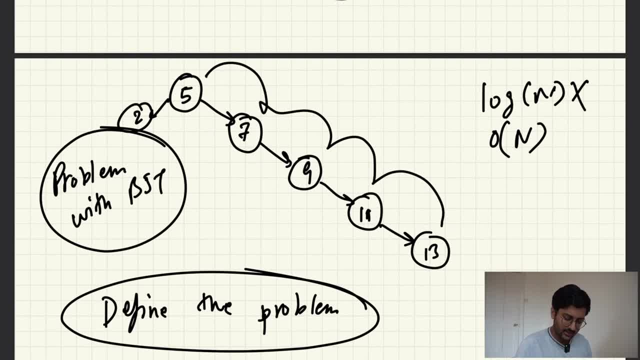 You know this one Why? Because the height of the left tree is 1.. Right tree, left tree is 0.. Right tree is 1, 2, 3.. So 0 minus 3, minus 3.. 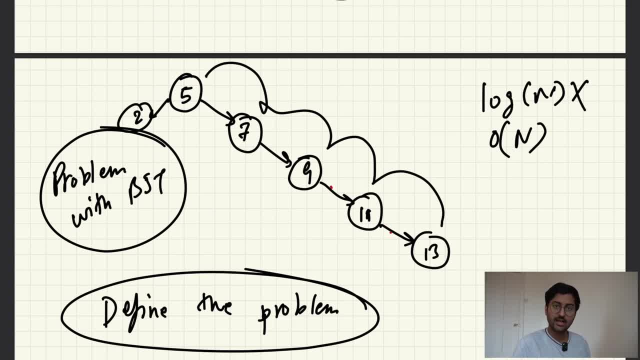 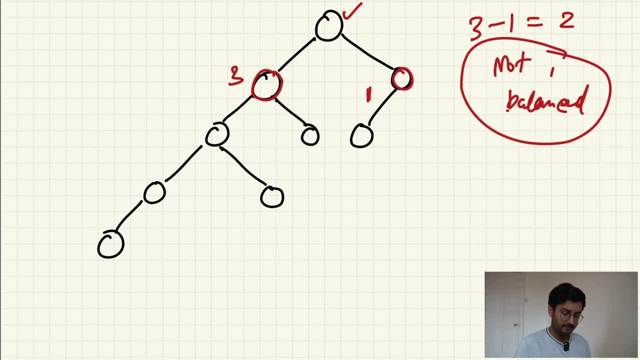 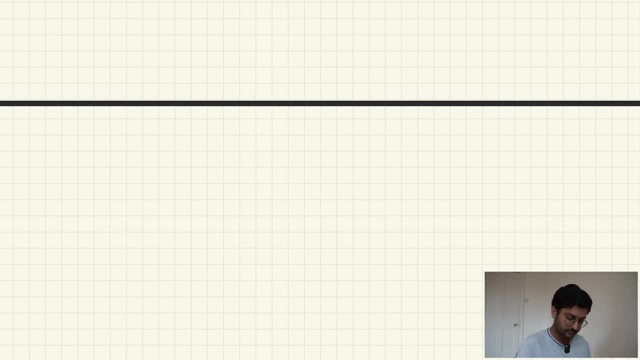 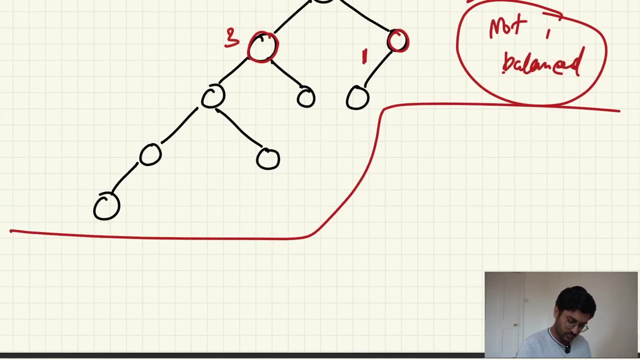 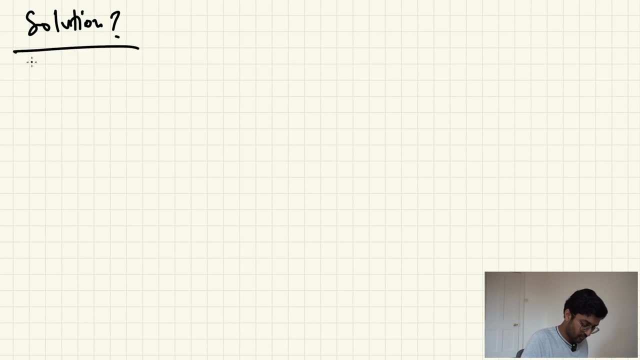 Not cool, Not good. Difference in height is 3, here It's minus 3.. Okay, Very simple stuff, Cool Now. Now moving forward. how to solve this problem? Solution Solution is self-balancing binary tree. 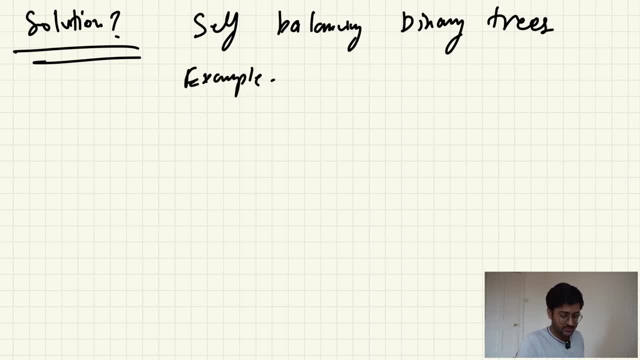 For example, one of those is AVL- Self-balancing binary tree- Self-balancing binary tree. Now you understand what was the problem and what problem self-balancing binary tree is trying to solve. So when you have a tree that is unbalanced, 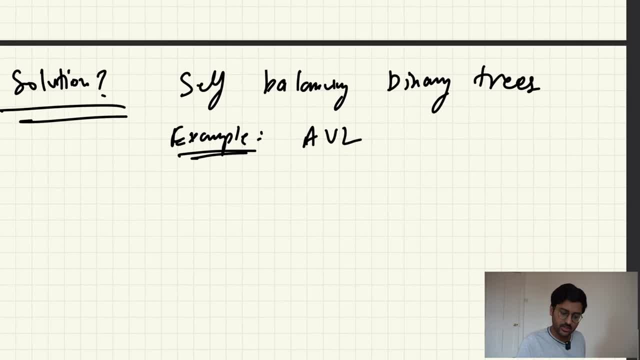 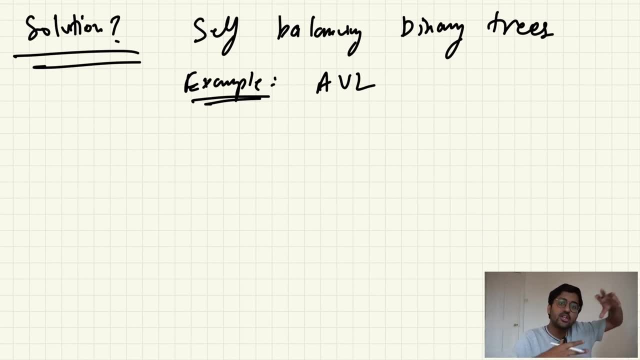 let's say you are adding something, adding something, adding something, and the tree becomes unbalanced. self-balancing binary tree will be like: okay, don't worry, You keep adding into the tree as you wish. I will restructure the tree in some way. 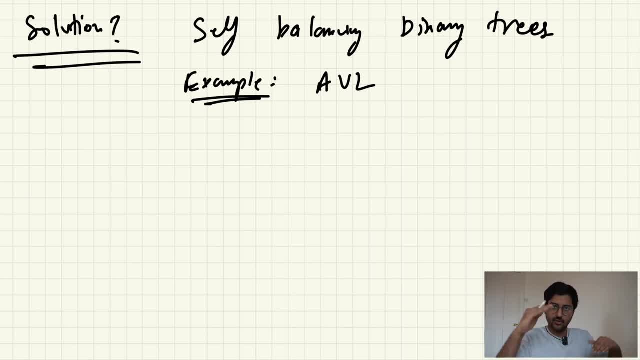 that it will always be balanced. And what is balanced? You already know the definition. That is what self-balancing binary tree is. Don't worry about how it's working Okay, Just think about what it's doing. for now, We will obviously look into. 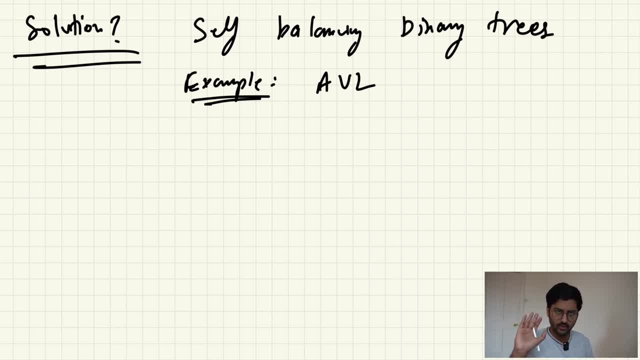 the entire code base, entire algorithm, all the theory, everything we will cover in this video. So don't worry about that. Try to focus on what this problem it is solving. What is meaning by self-balancing? Self-balancing means. 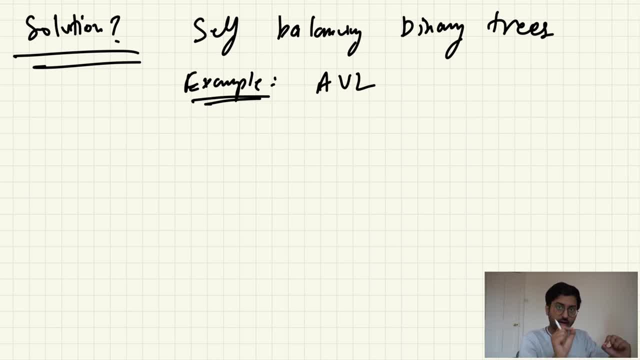 you just keep inserting in it and we will apply some algorithm that whenever you insert an item and that insertion makes the tree unbalanced, it will be like: okay, Kunal just added 20 in the tree, a node with value of 20, and. 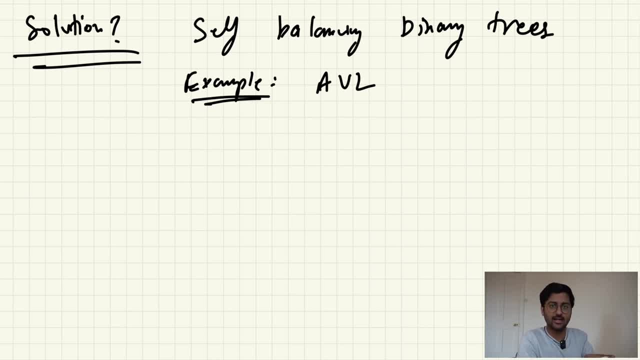 it has made my tree unbalanced. No problem, Kunal, Just add it as you want And normally, and I will restructure the tree in such a way that it will become balanced, That it will become balanced, Okay. So, for example, 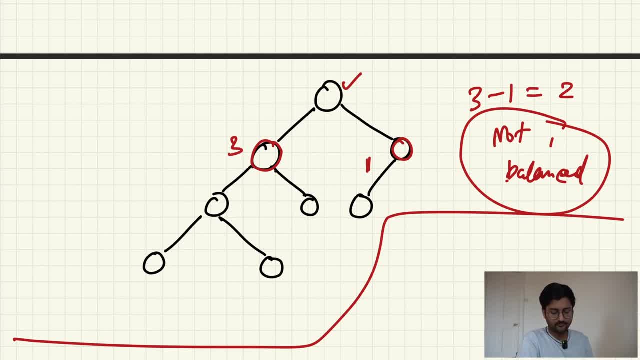 this is balanced tree. Okay, It's the same tree as previously, So it's going to be like: okay, Kunal, right now, this is balanced, No problem. Kunal is going to be like: okay, I will add one more. 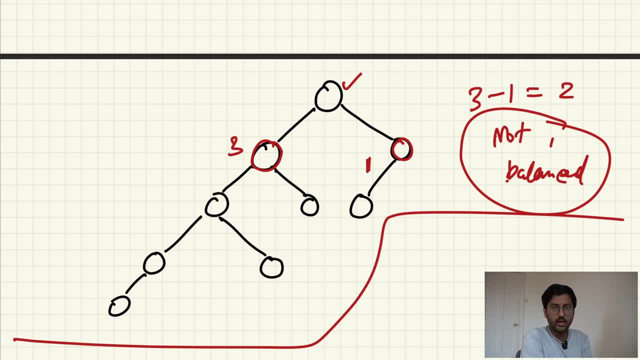 node over here, The tree is going to be like: oh, now you added one more node. Now this tree is unbalanced. So don't worry, Add your node where it's supposed to go. I will then restructure the tree and balance it. 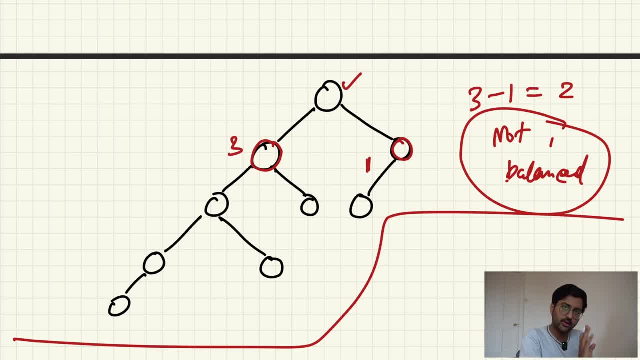 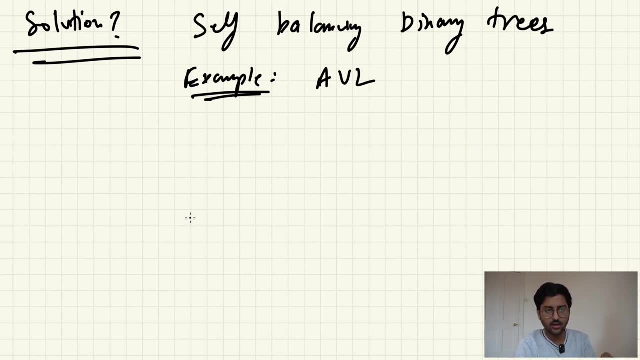 How we are going to balance it, we will figure out later. Okay, Sounds good, Let's move forward. So that is basically what self-balancing binary tree is, And one of those trees is called AVL tree, So let's see how AVL 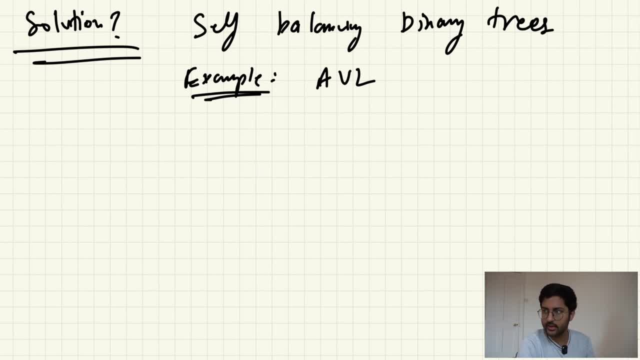 tree solves this problem. and what does it mean by AVL tree? So AVL tree, self-balancing binary tree, the full form is, I think, based on the people who founded it. could be that So it's called Adelson. 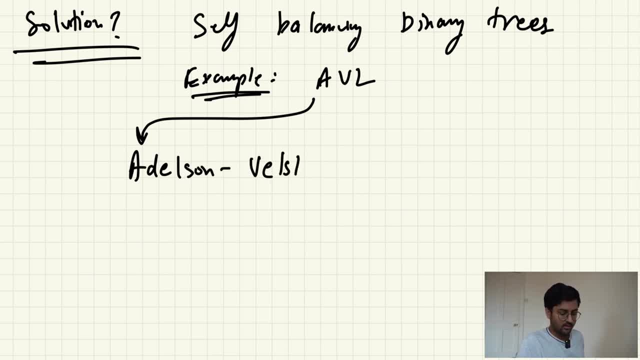 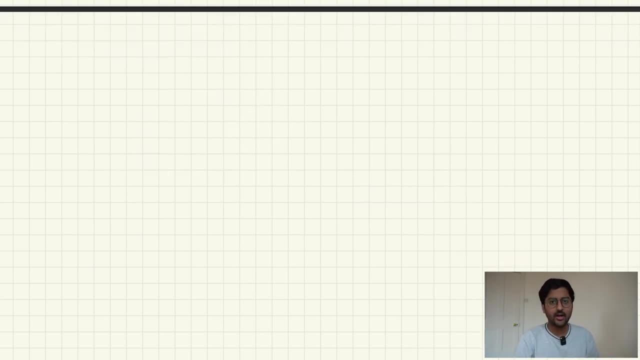 Adelson, Adelson, Welski, Welski and Landis AVL trees. Okay, Cool, How it works, Let's see. Okay, So let's see how AVL tree functions. So, Kunal, we know that you are saying that AVL tree is. 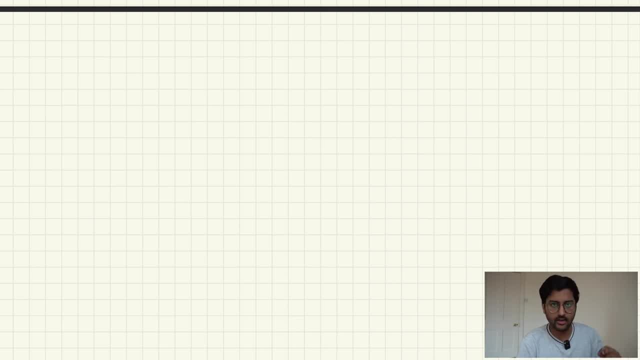 a self-balancing binary tree? Okay, no problem. Sometimes we have. we may insert some node in a tree and that will make that tree unbalanced. We know what unbalanced means And when tree is like. oh Kunal, you just. 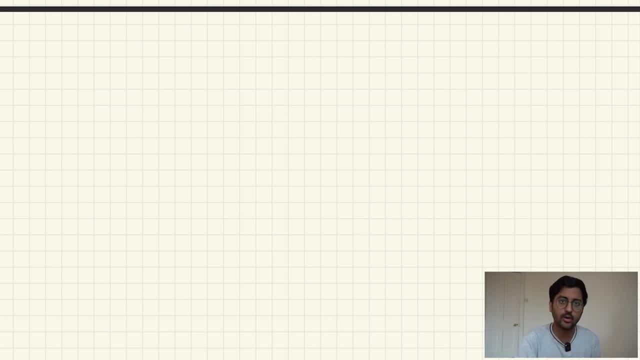 inserted this node, tree has become unbalanced. Now, don't worry, Kunal, I AVL tree, I am an AVL tree, so I will make the tree balanced automatically. So obviously, if a tree has become unbalanced, then to make it. 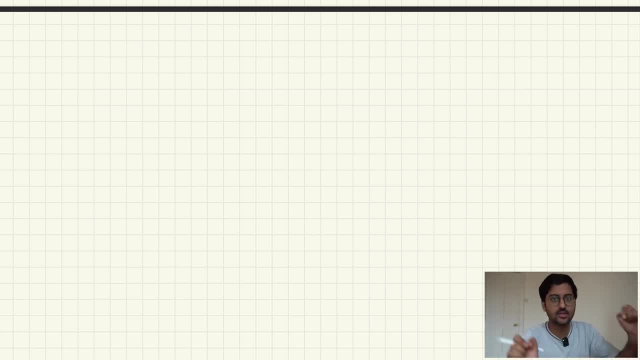 balanced. you have to change the structure of the tree, You have to move some nodes around to make the structure of the tree Balanced. pretty common sense. Now the question is, how do we do that? So what is the basic method? 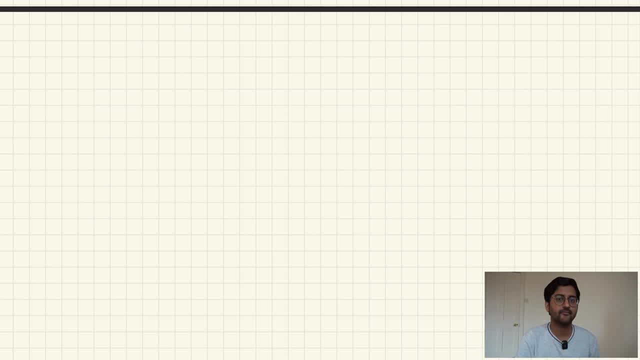 via which the tree will adjust itself. What is the basic method? Let's see. So let's say you have a node. Let's say this is a parent node, This is a child node, This is tree number 1.. This is 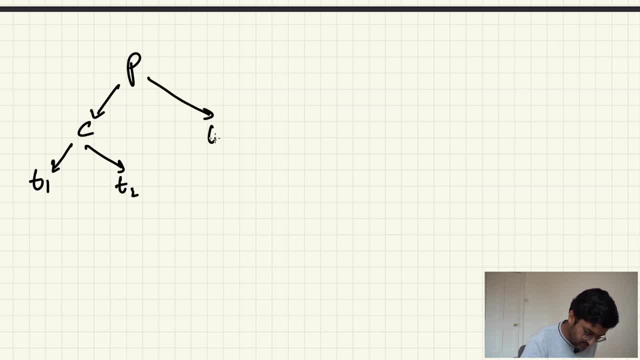 tree number 2.. This is tree number 3.. So there are two methods using which we are going to form our algorithm, but two basic steps. First one is, if you want to, there is only two things you can do for every node. So let's say you found. 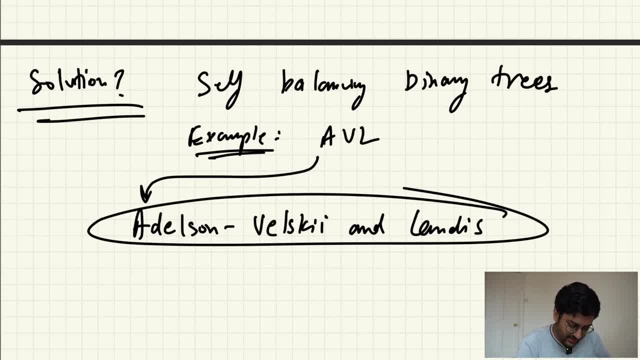 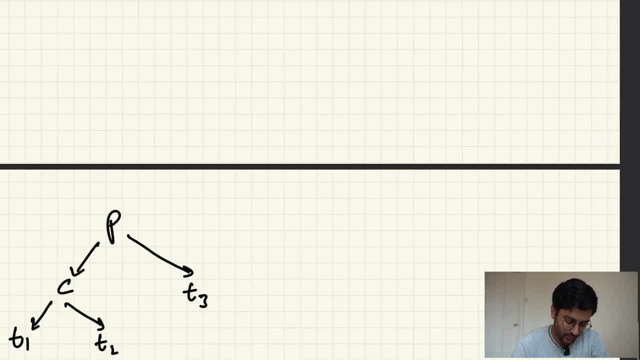 a node and you are like this node is making it unbalanced. For example, if you try to look for, you started adding it from here. let's say you started adding it from here. let me show you how it works. Let me show you how it works. 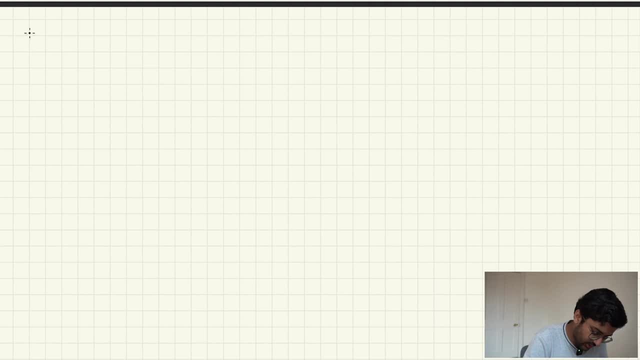 So before moving forward, I will just write down the algorithm for AVL tree. Then it will make more sense. Step 1 you have to do is insert normally. Insert normally node node n, For example. insert normally node n. Now start. 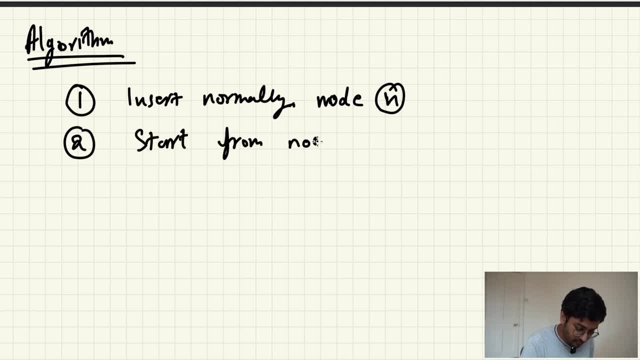 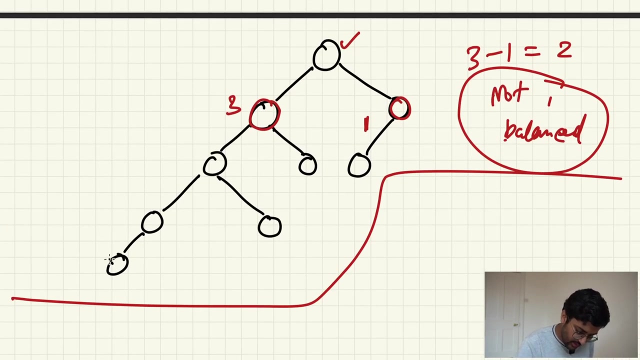 from node n and find the node that makes the tree unbalanced. So you are saying, Kunal, start from the bottom up. Yes, Taking an example of the previous question, add the node normally. Added the node normally. Start from this node n. 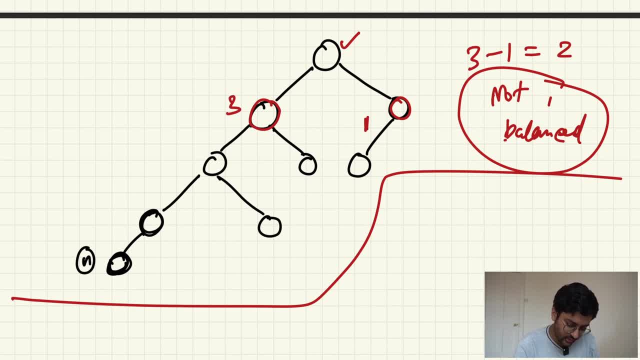 work above. Is this node unbalanced? No, it's not. Is this node unbalanced? Yes, it is Sorry. no, it's not. Is this node unbalanced? Yes, it is So. is this node unbalanced? 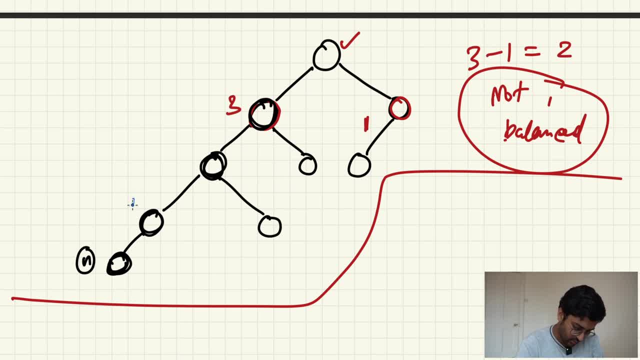 No, No, this is not unbalanced. Okay, keep moving up. No, this is not unbalanced. Okay, keep moving up. Yes, this is unbalanced. This node is unbalanced. So now we will solve this particular subtree before. 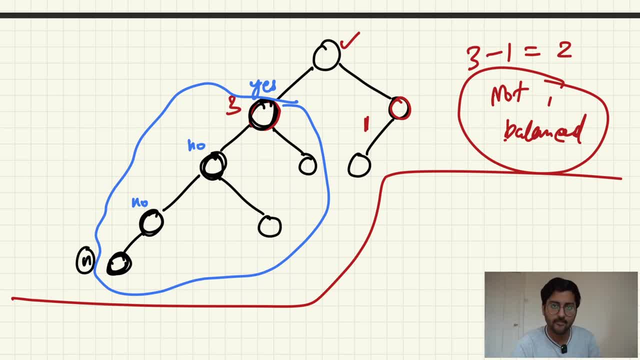 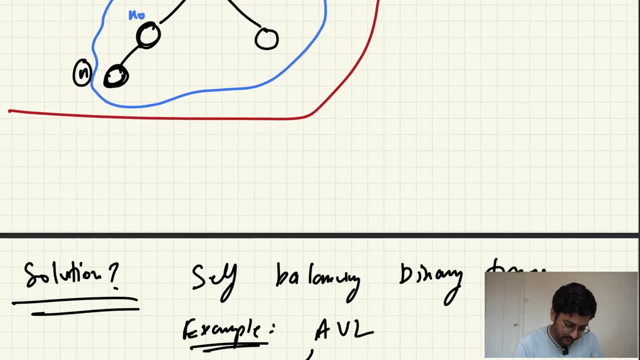 moving more up. That is avial tree For every subtree. how you can solve it is for every subtree. think only two things you can do. Let's say we have this subtree, So in this case, in the bottom one, this will be: 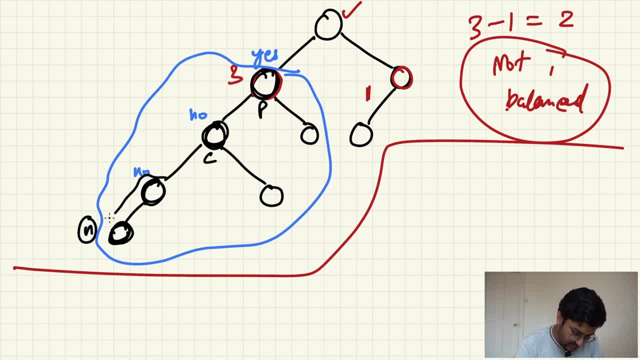 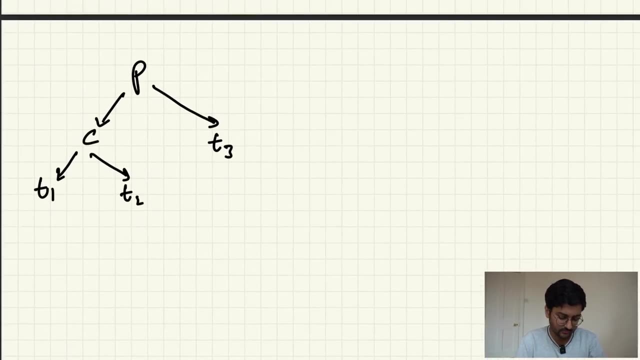 equal to p, This will be equal to child, This will be equal to tree1.. This will be equal to tree2.. And this will be equal to tree3.. Make sense? So only two operations you can perform: Parent, child, tree1,, tree2, tree3. 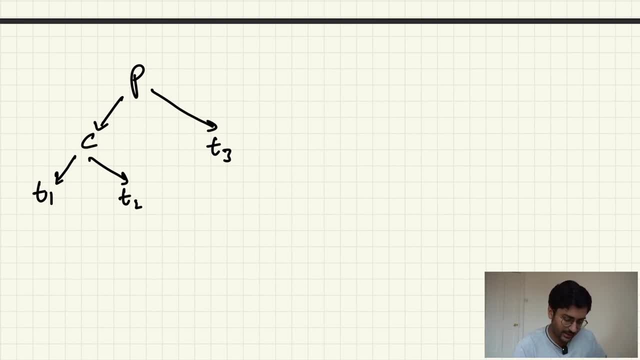 I showed you in the real world example how this is going to be related, So you can check that out. You can either rotate it on the right hand side or you can rotate it on the left hand side. If I rotate it on the right hand side, 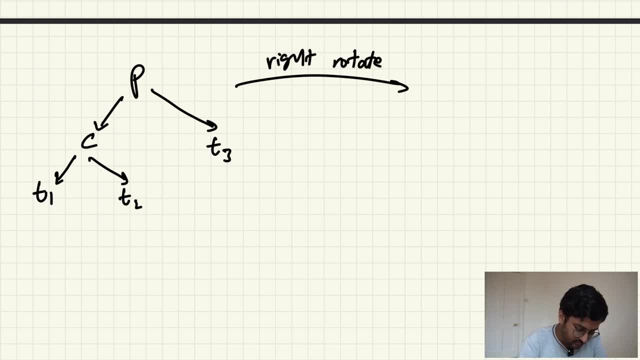 it will go down. So this will go down, C will go up, C will go here, p will go down And p will obviously go on the right hand side of c, because p is greater than c and in binary trees, anything. 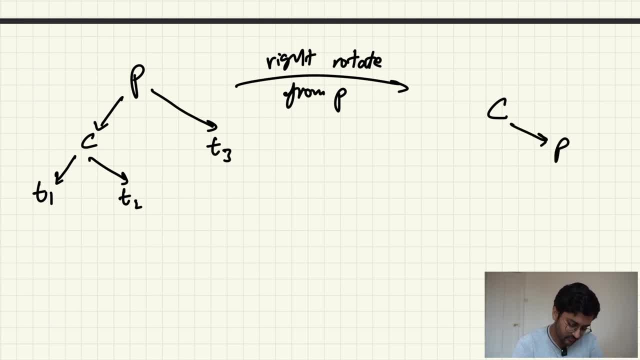 that is greater than the node goes on the right hand side. p has tree3 on the right hand side Now, no problem. Now c has tree1 on the left hand side, No problem. tree2 was replaced by p. tree2 is actually, I know, smaller. 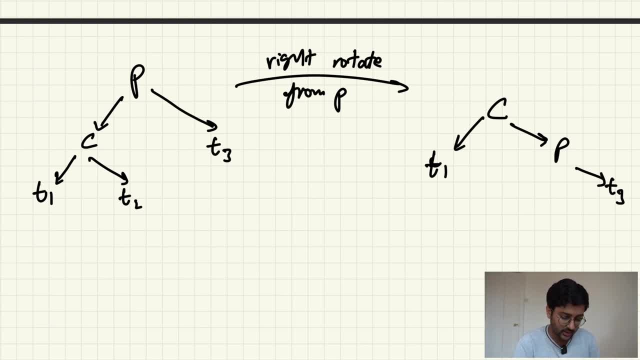 than p, because it was originally on the left hand side of p, So it will be on the left hand side of p. Similarly, this is left rotate. This is like the basic concept. Please note that the binary search tree property- that all the elements on the left hand side- has to be smaller. 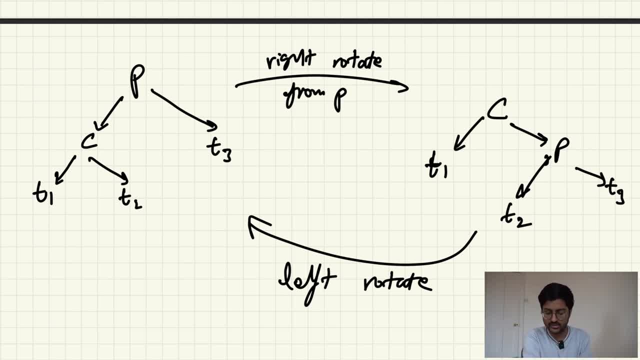 and right hand side has to be bigger for every node is still holding true for this case. Originally, t2 was on the left hand side of p. Now also, t2 is on the left hand side of p. Originally c was actually. 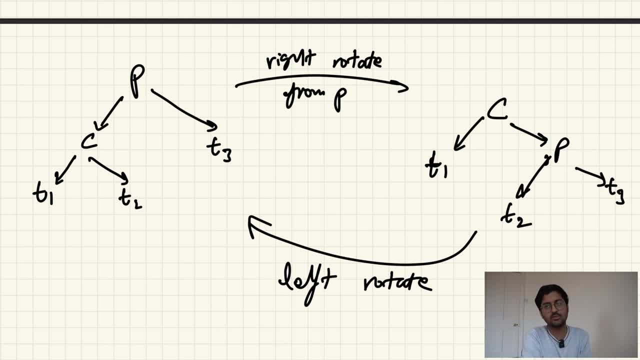 smaller than p. In the rotated one also, c is smaller than p. Similarly, you can do the left rotate also. If you want to do left rotate, then okay, p will come up, c will go down, t2 will go on the right hand side, and so on and so forth. 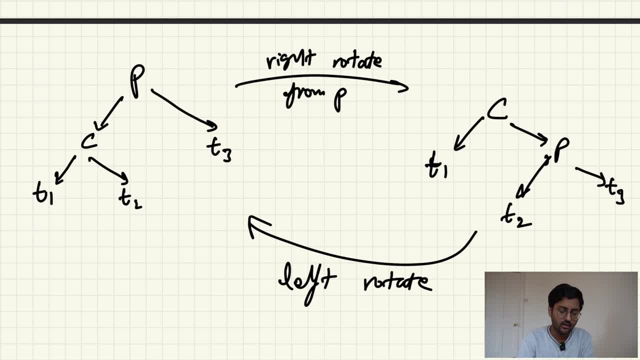 Very simple. These are the two basic formulas that we will use. Okay, Very simple. So AVL tree is not difficult, It is a little confusing. It can get a little confusing because there are so many moving components. After this we will see four rules of 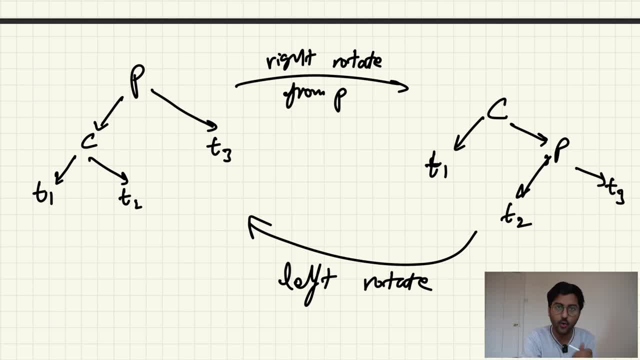 how to apply these two methods. You can apply these two methods in four ways, Okay, Okay, So it is not difficult at all. It is just like there are too many components. There are two things like this, and then there are four rules. 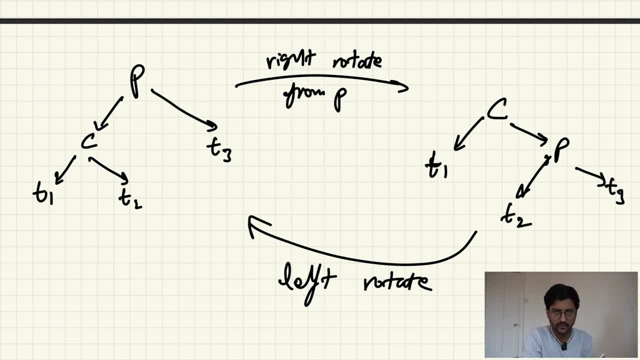 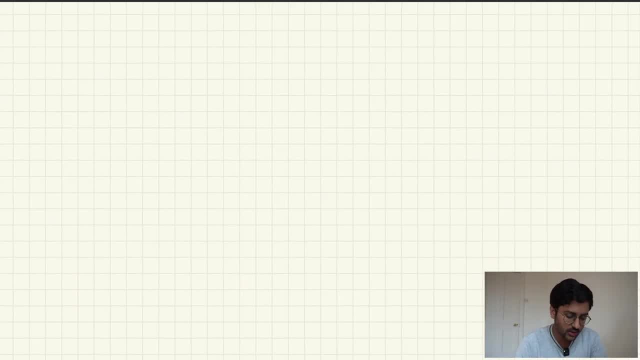 And then there is the balanced and unbalanced thing. So it is not difficult at all. I hope this is clear, Very simple stuff. So let's take an example. So if I take this example over here, If I take this example, 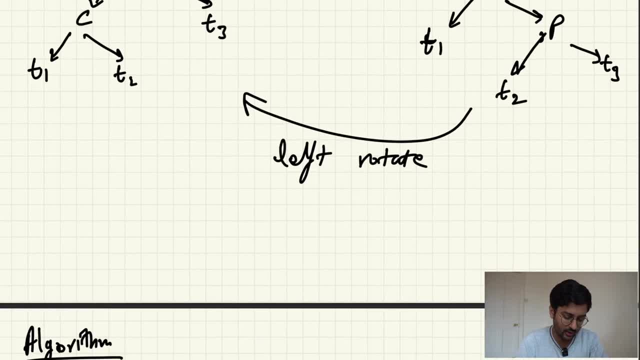 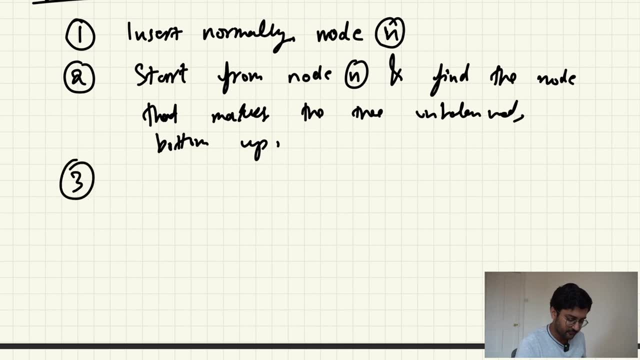 this one, like we found in AVL tree. So you know how it basically works That start from the node n, find the one and bottom up and after that, using one of the four rules, rotate. Okay, That's it. What four rules? 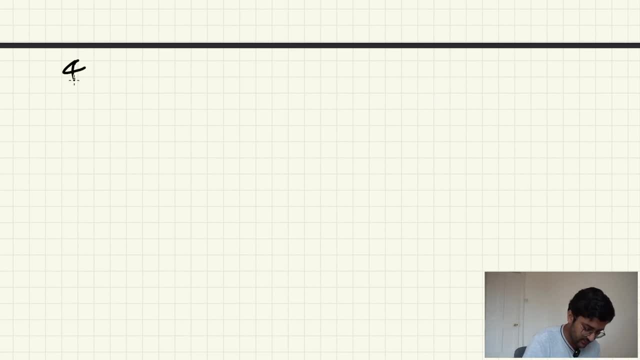 Let's see Four rules. Rule number one. Rule number one: It's very simple In the previous example. let's say we had a parent is over here and let's say you have a child over here and that child has a grand. 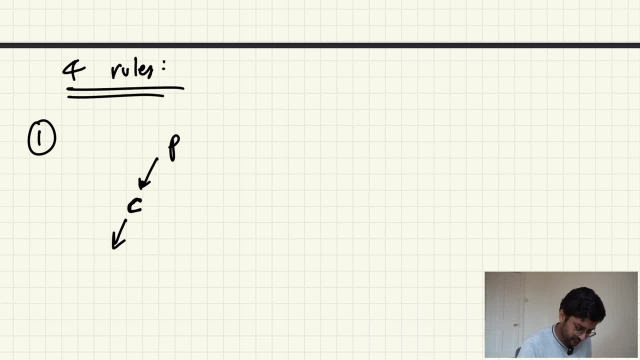 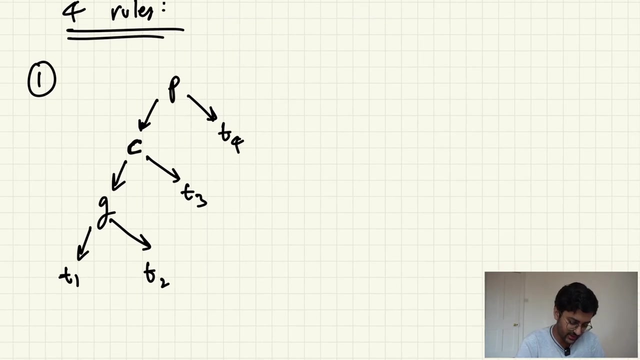 child over here, G Okay, And then this has tree one and and tree two, tree three and tree four. Let's say you have a situation like this. There are only four rules possible. Okay, Now you will be like Kunal. 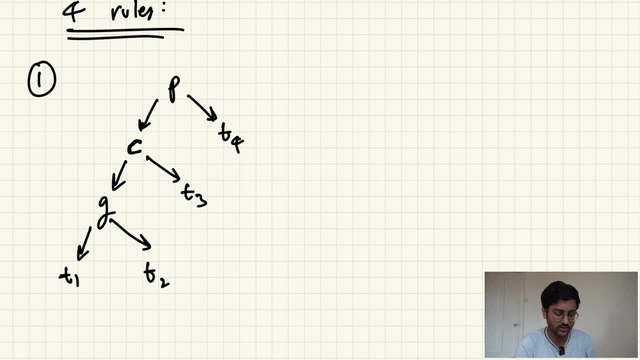 how did you figure out? this is the grand child and the grand child is, let's say, not on the right hand side. That is also one of the cases that we will cover, But the grand child is actually in the line of where the element was added. 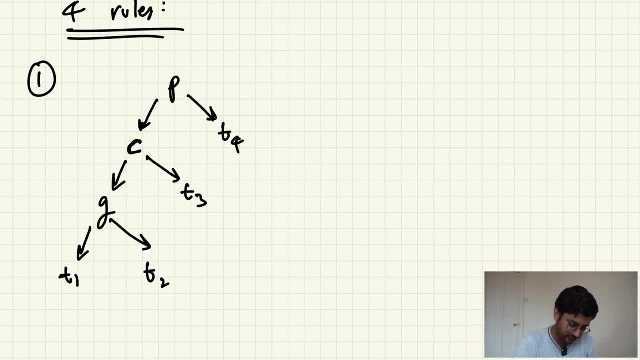 So if your element was added over here, then this will be grand child Because it is in the line from the element added to the parent. Okay, If the element was added, you know, somewhere over here, then this would be grand child because it's in the line to the parent. 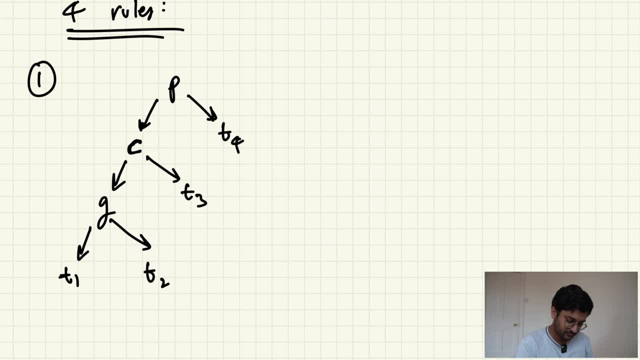 I hope that is clear. It's very simple stuff. Okay, Let's move forward. So let's say we have one of these four cases. So in this case, imagine that the P point. let's say, for example, these cases are for unbalanced. 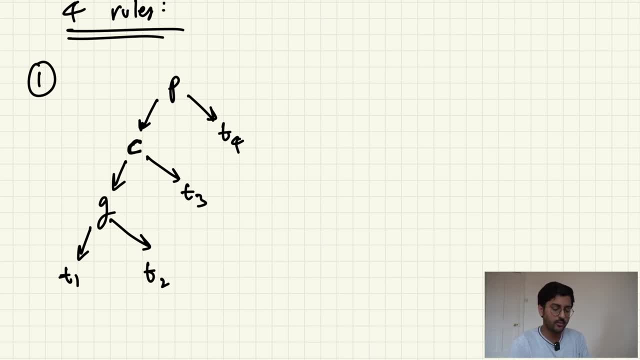 binary tree sub trees. So this P is where we are going to be rotating it. So in this case, what we are going to do is, if we find a case like this, we are just going to right rotate, Right rotate From P. 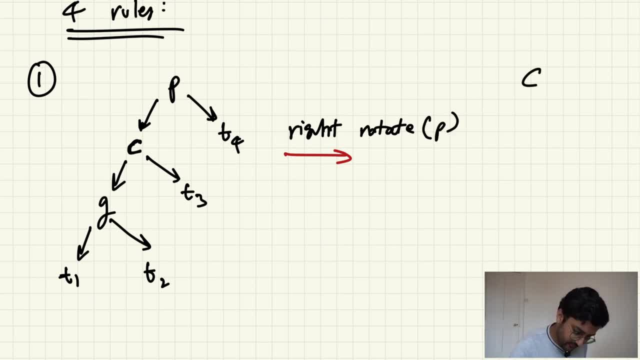 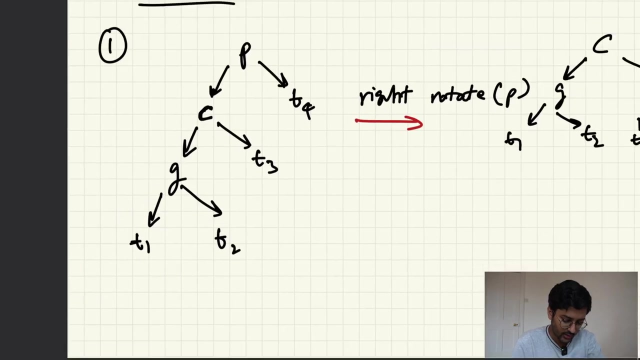 So C will come above, P will go over here, T4 will go over here. Then what? T3 will go over here, G will stay here, T1, T2.. Make sense, Sounds good, Okay. Case number two. 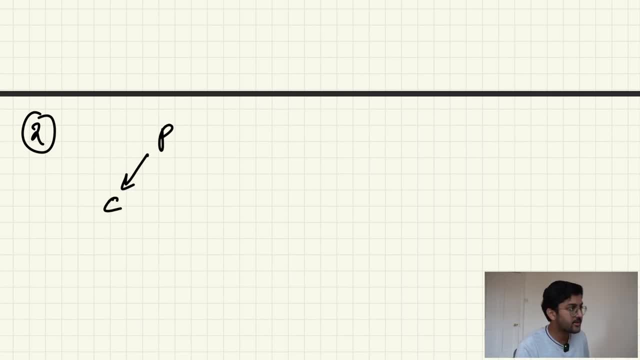 Let's say: parent like this, You have child like this. And let's say: here you have T4.. And let's say: now you inserted something, There was a tree over here- T3.. And let's say: you inserted an item over here. 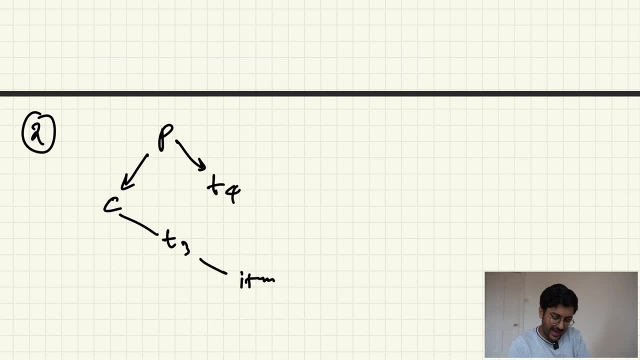 Then the item inserted in that lane, the child of child is going to be the grand child. Okay, Okay, Okay. T3, T3, T2, T1.. These are subtrees T1,, T2, T3.. Okay, Alright. 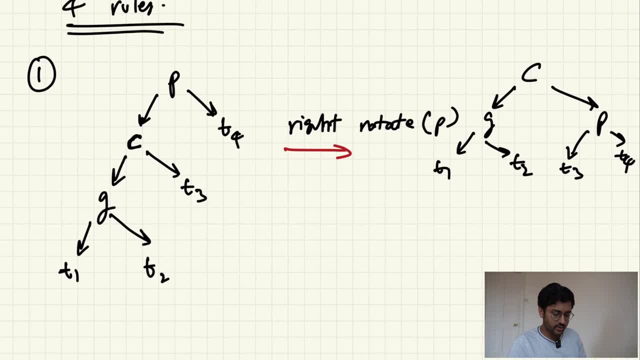 Now what we are going to do is this is actually going to be the. this first one is going to be the left-left case. So you have the child and grand child. Both are on the left-left side. Both are on the left-left side. 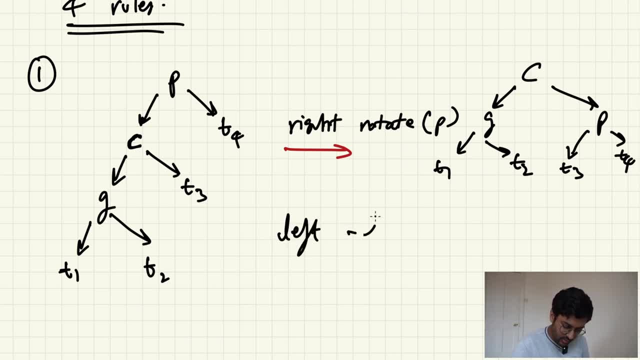 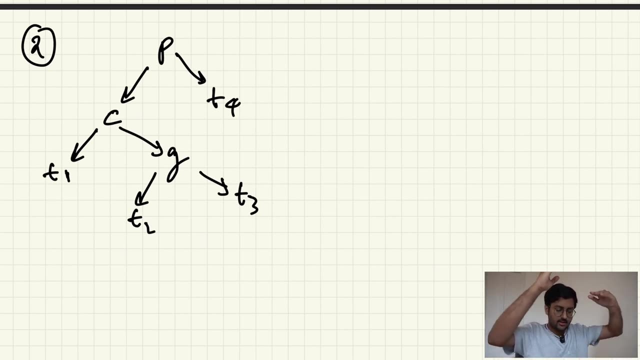 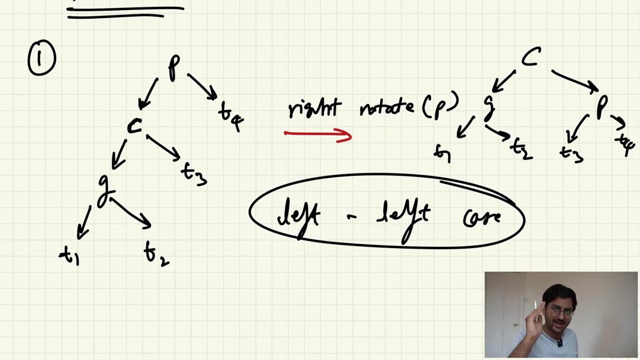 So left, left, left, left case. Here you can see that it's left-right, So this is left-right case. Your motivation is to convert the tree in a single line, This parent-child, grand-child, right. Convert it into a single line. 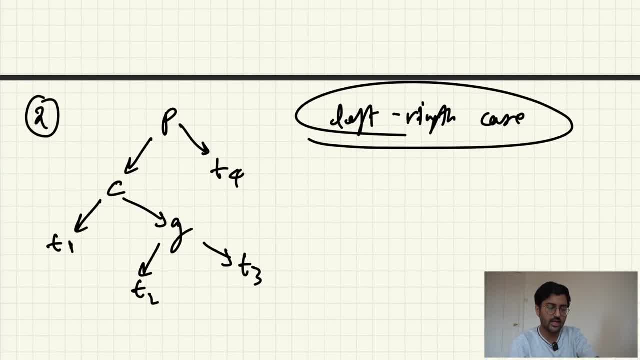 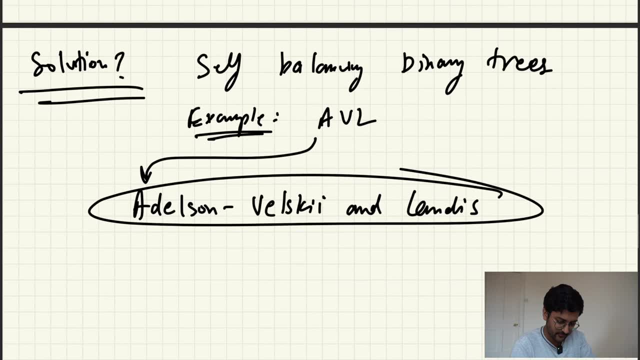 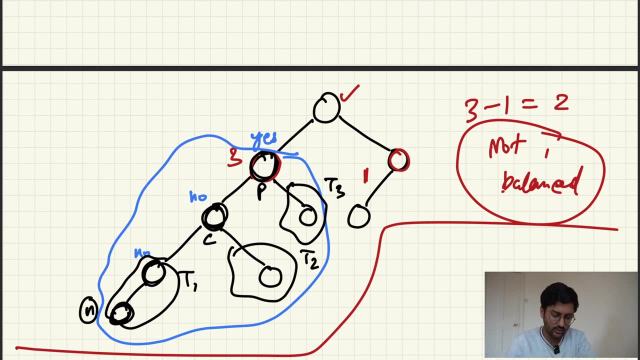 That should be your motivation. So, because then you will be able to rotate and make it balanced. Okay. So here you can see it was, for example, in this case single line- parent-child, grand-child- Okay, Similarly, you can rotate. 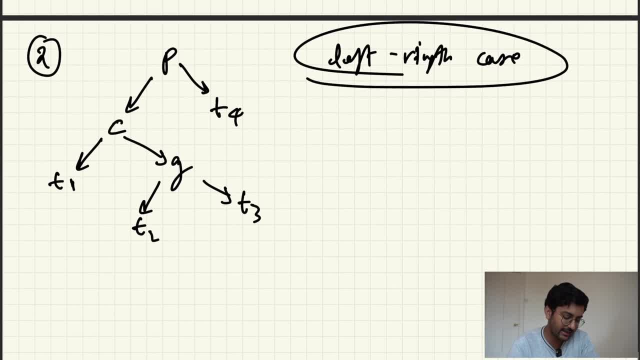 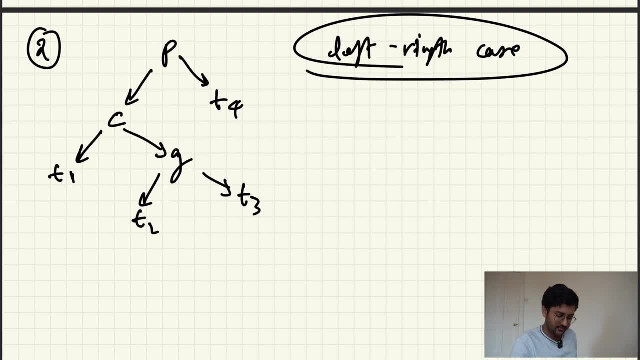 But here you can see, it is not in a single line, It is zig-zag. So I am going to first make it into a single line. So, to make it into a single line, I start from the bottom, and what I will do is I will put. 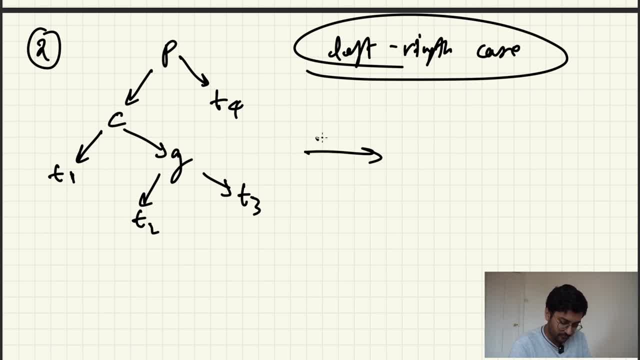 g over here. I will do left rotate g, sorry c. Left rotate c. That will bring g above. So it will make my tree something like this: g will come over here and then child will come over here. Tree 1,. 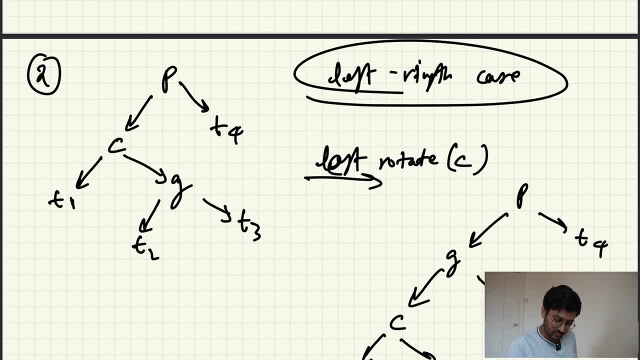 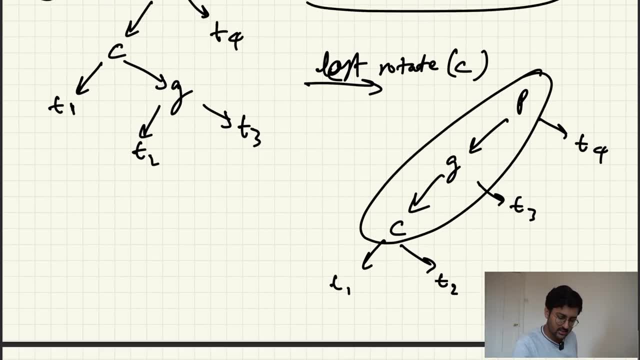 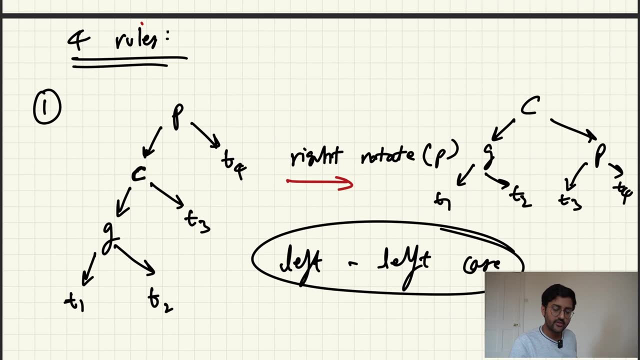 tree 2, tree 3.. Now you can see it is in one single line. And is this not the same as this one first one? So what is the case for first one? What do we do when we have a structure like the first one? 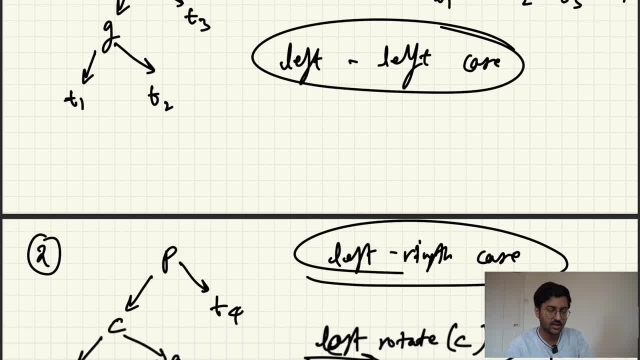 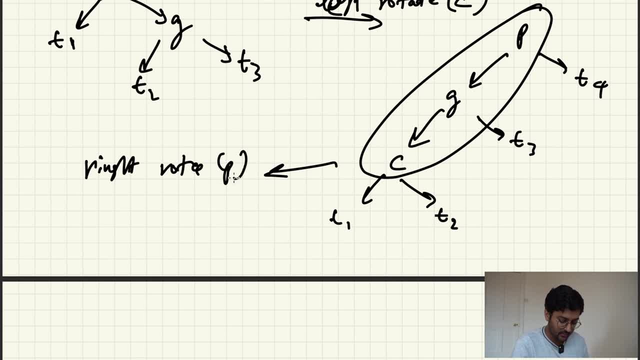 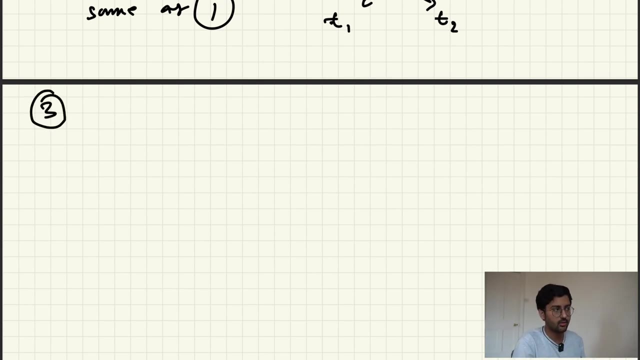 We right rotate on p, Right rotate on p. After this, right rotate p. Same as one. Very simple, Don't try to think about it. These are the only cases you can have. Then. what other solution do you need? What other explanation do you need? 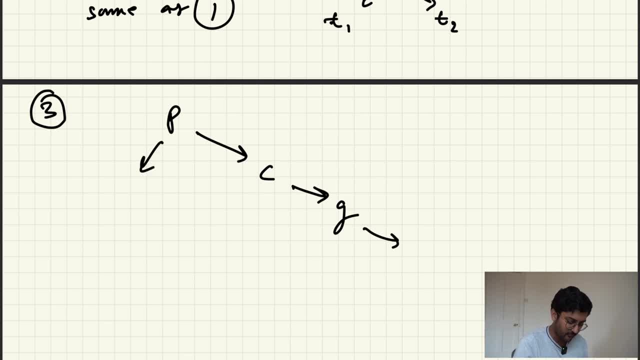 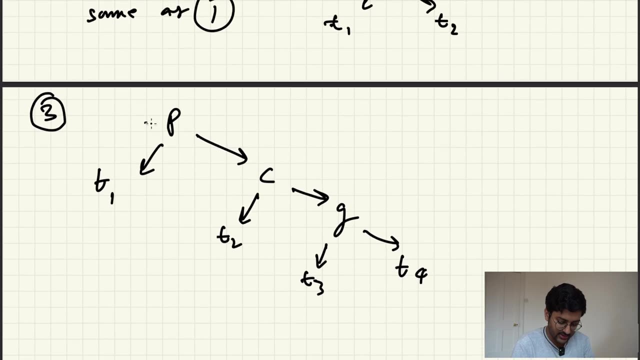 Let's say parent, child, grandchild 4, or I can say T1, T2, T3, T4. It is one single line, So i will just simply rotate. It is right-浞 case, So i will rotate it on the left hand side. 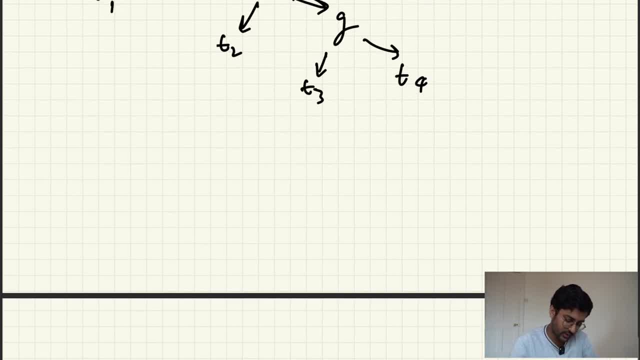 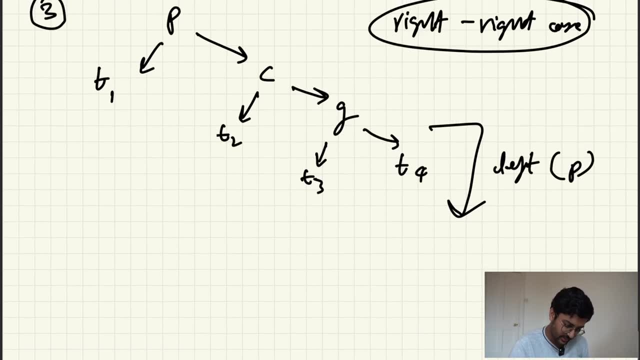 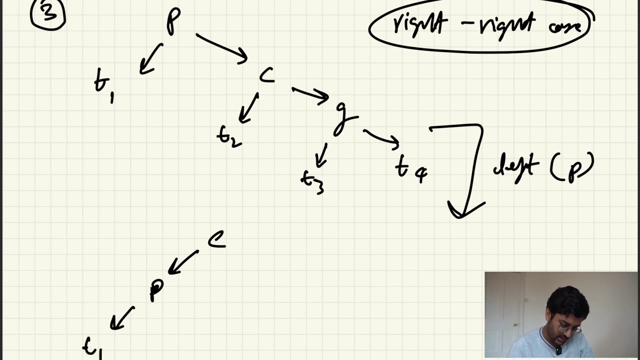 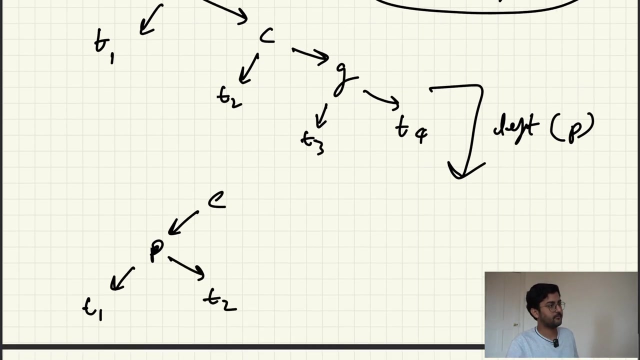 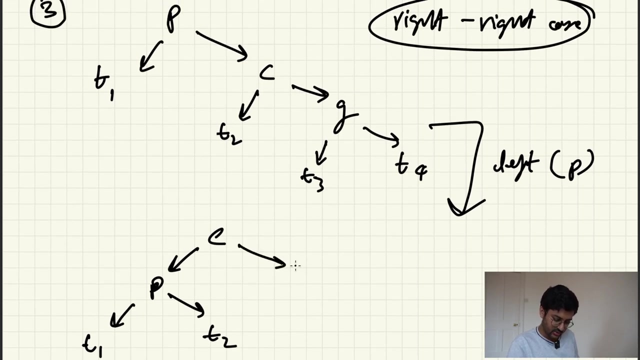 Right, right case. Move it on the left hand side. Left rotate on P. C will come above. P will go here. T1 will go over here. T2 will go over here. okay, because this has to be greater than P. greater than P, that is fine. G will. 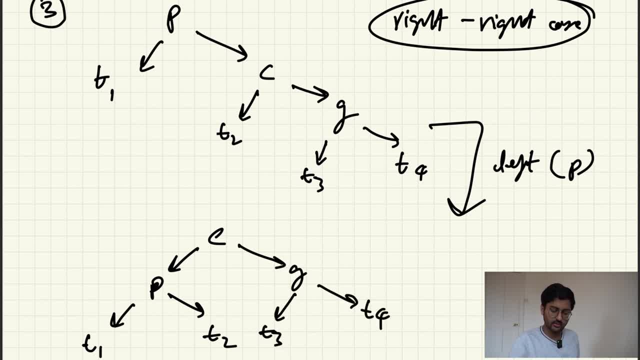 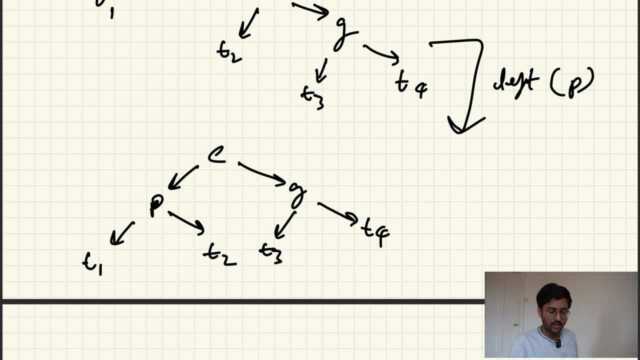 be here. T4 will be here. T3 will be here. that's it Balanced. Now you will be like Kunal. how do you know that the individual trees, T1, T2, T3, T4, are balanced? 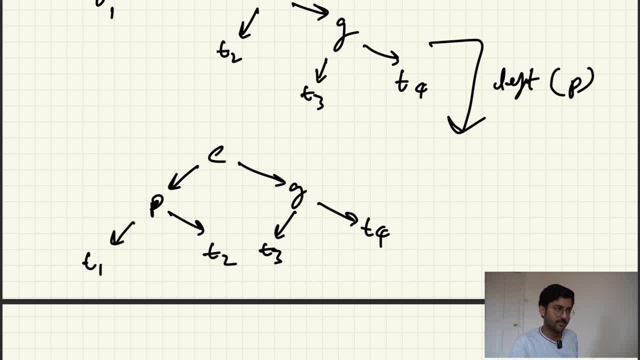 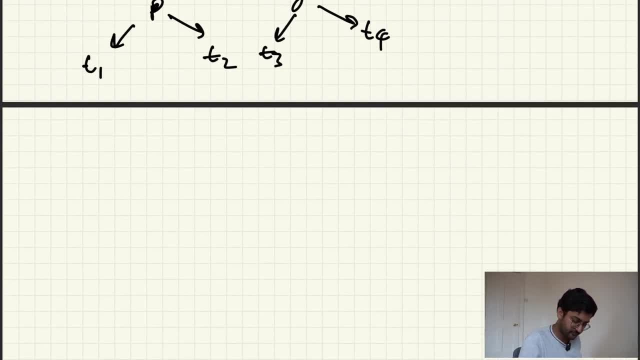 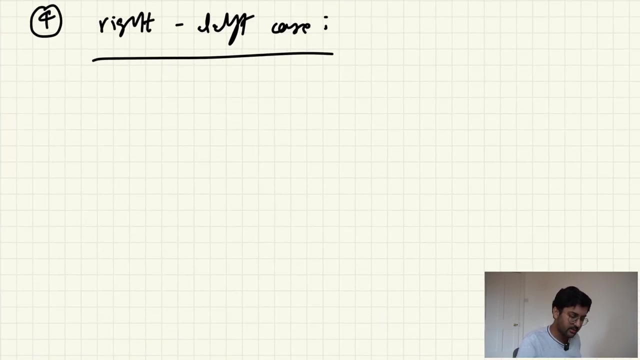 Because we are starting from bottom up. okay, that's why Right, right case. done one more case left. Right, left case. this is again very simple. let's say I have my parent over here, my child over here and my grandchild over here- T1, T2,, T3, T4, so I have to make it in one single. 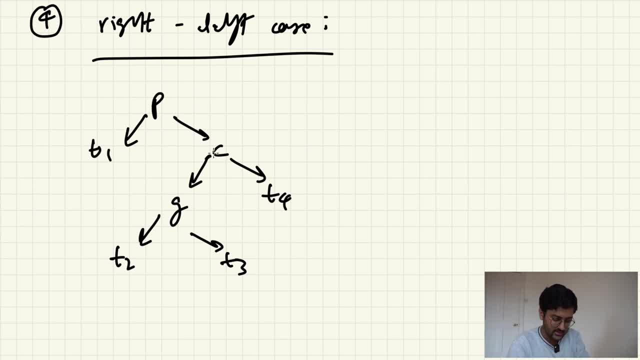 line. I will start from the bottom up, so this one. I will see C and I am going to right rotate it on C. this will become G and C will come over here. T4, T2, T1, T3. 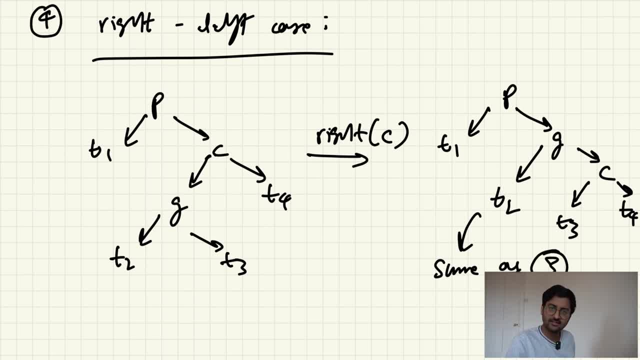 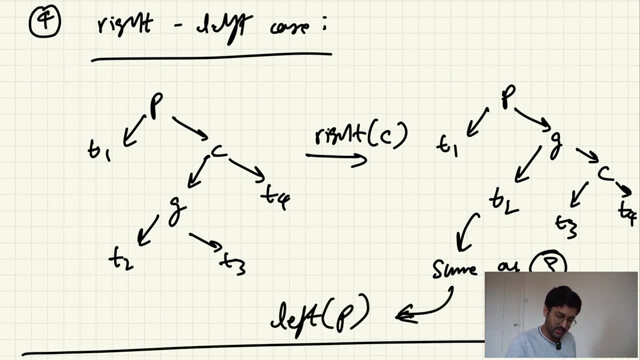 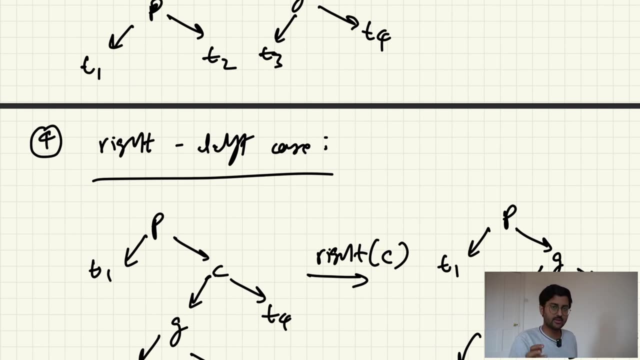 Now, this is same as point number 3, right, Same as point number 3, so I will do left rotate on P. These are the only four cases. why do we have these two extra cases? Because sometimes you get right left, sometimes you get left right. those are the only two. 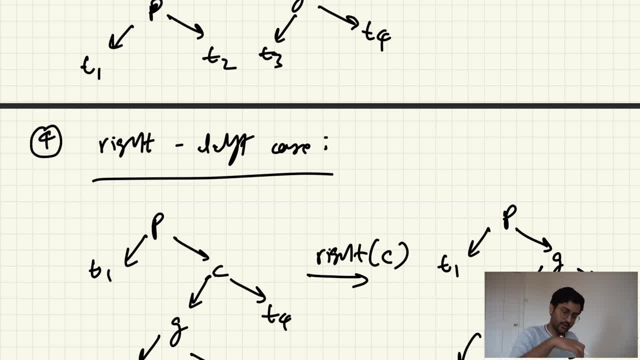 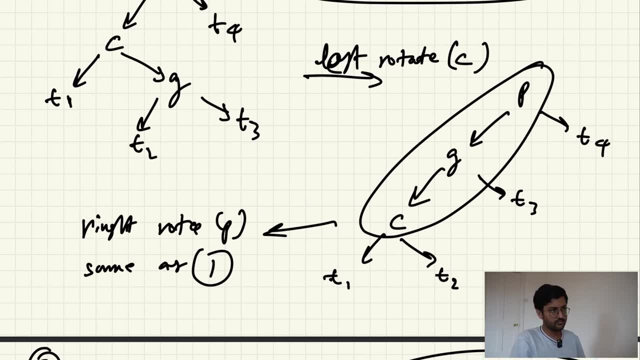 possible explanations. so you first make it in a single line and then rotate it. And how do you know that individual trees are balanced? Because we are starting from the bottom up. that's the AVL algorithm. insert it normally. start from the bottom node. 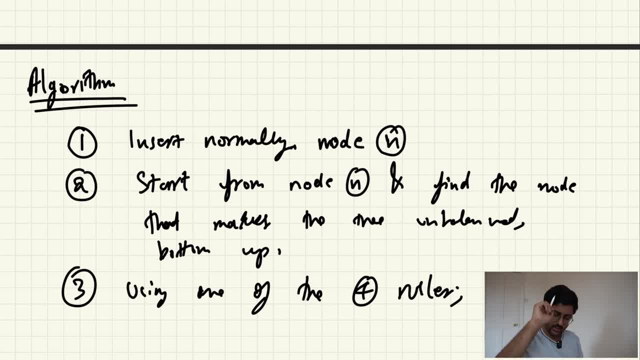 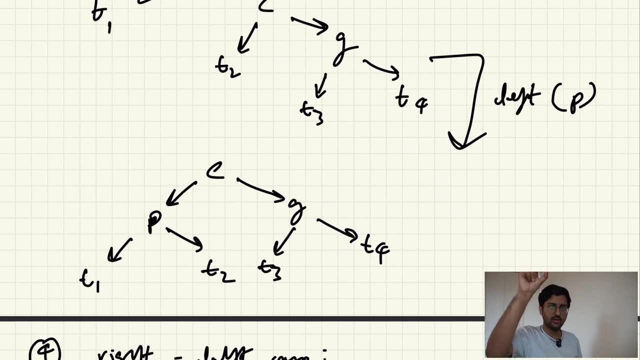 And find the node that makes it unbalanced from bottom up, then do the one of the four rotations. That's it, very simple, Because that node made it unbalanced right. That is why we are going to figure out the first tree that makes it unbalanced. we are 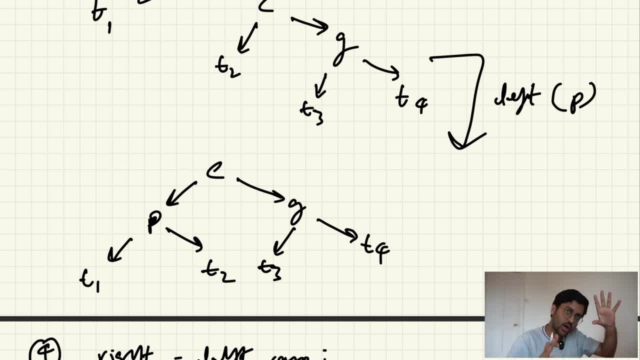 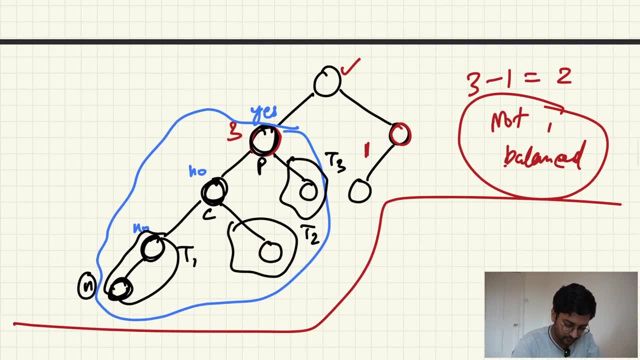 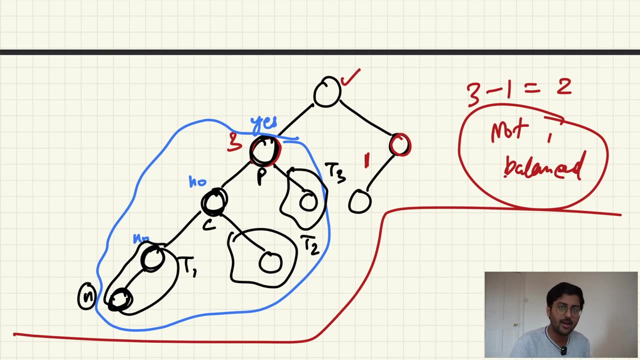 going to solve that tree. So when the subtree itself is not unbalanced, the other tree- oh yeah, that's one more other point. So we added one node. then we made sure that the first tree that it unbalances we solve. 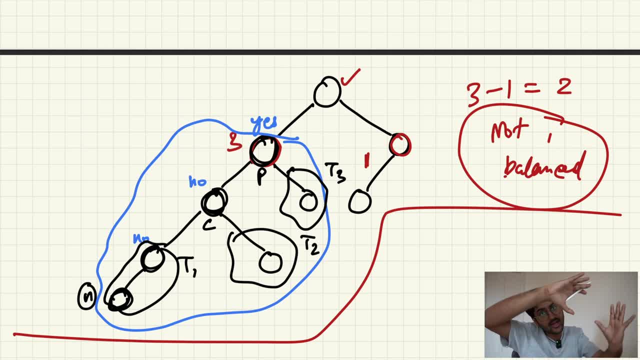 that. So this subtree we solved. So when the subtree is balanced, the above tree is also going to be fine balanced if it is already balanced. Try to understand: while we are adding elements we are making sure tree is balanced. So before I add an element, let's say 100 elements are in the AVL tree. we know that. 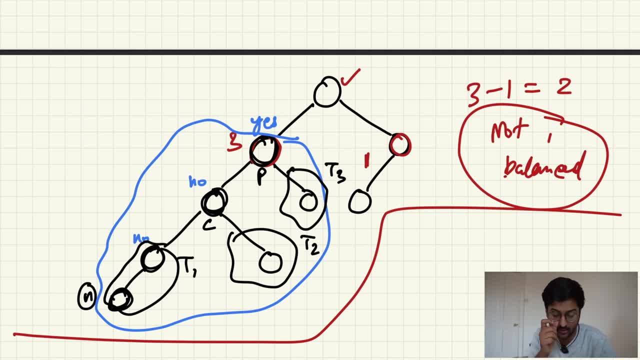 those 100 elements By definition of AVL tree. this is a very important point. I forgot about mentioning this. It's the intuition, the thing that will click When you are trying to add. let's say, you add 100 elements. okay, I know that 100 elements. 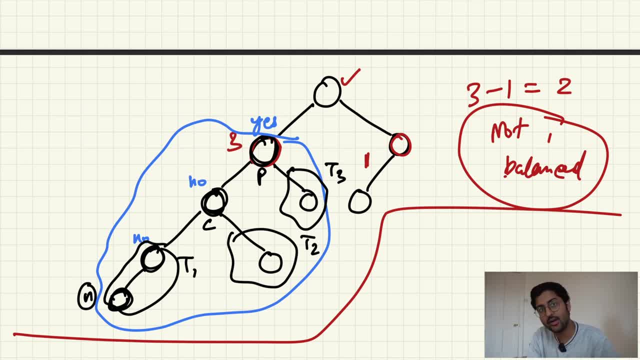 are added, 100 nodes are added in the tree. I know it's an AVL tree, so I know it is a balanced tree, Because at every point of time it will make it balanced. Now I add one more node and I'm like: okay, this node made a subtree, a part of this tree. 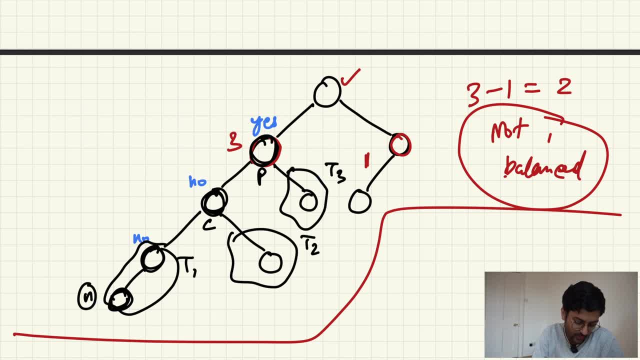 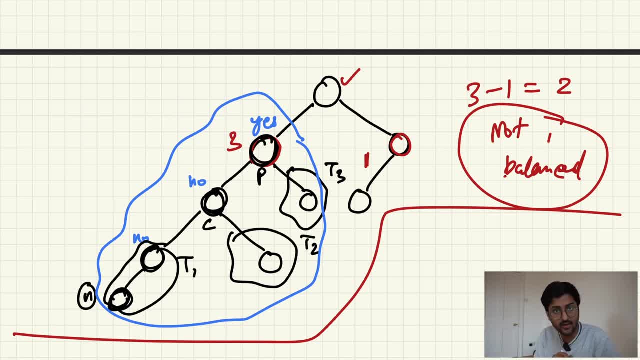 So I will just solve this subtree. I will make this subtree balanced and when this subtree is balanced, it is going to be fine, because it's not going to affect the entire tree, Because the entire tree is already balanced. Make sense Sounds good. 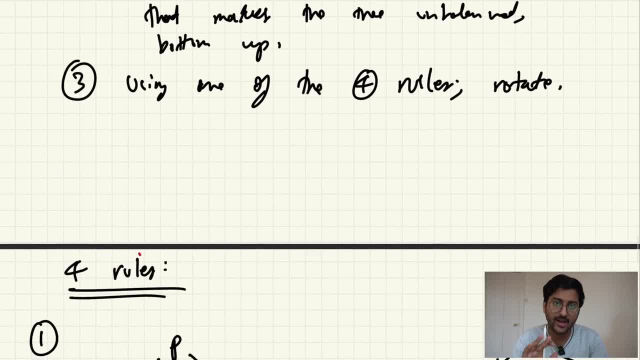 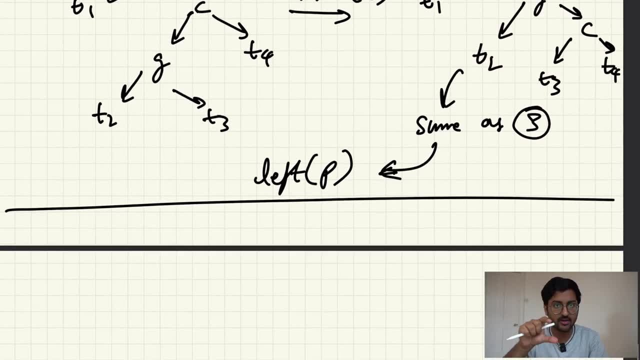 Okay, So the entire tree is already balanced. that is established, Only solve the subtree that became unbalanced. And if, using that subtree, other trees were unbalanced, those will also be balanced, Because the subtree was unbalanced, so it got balanced, hence all the other subtrees. 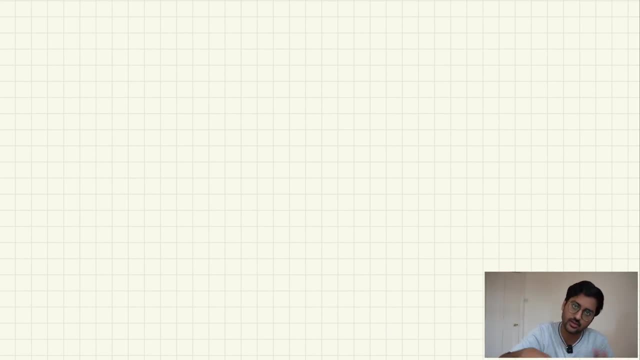 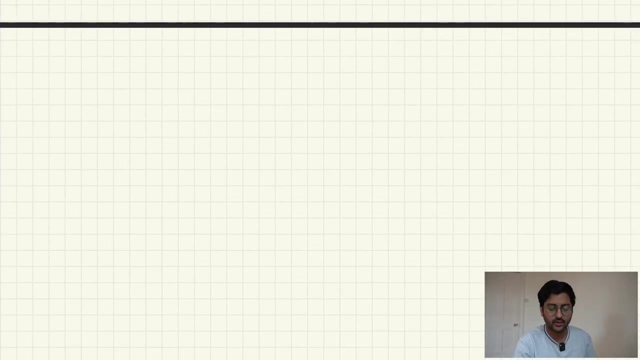 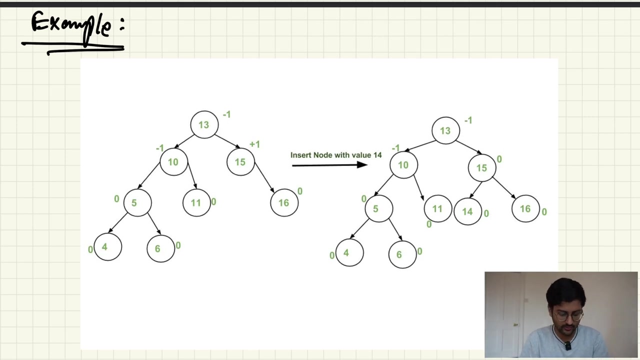 that were all the trees above it that were unbalanced because of it. those are now also automatically solved. Okay, Okay, Okay, Okay, Sounds good. We can take an example and see into a picture. Okay, So I got this example online from GeeksforGeeks and I didn't want to, you know, make it all. 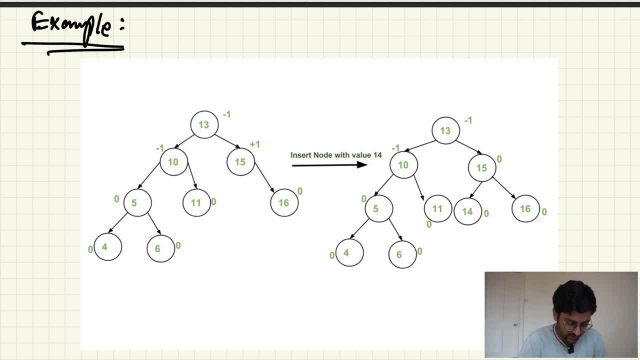 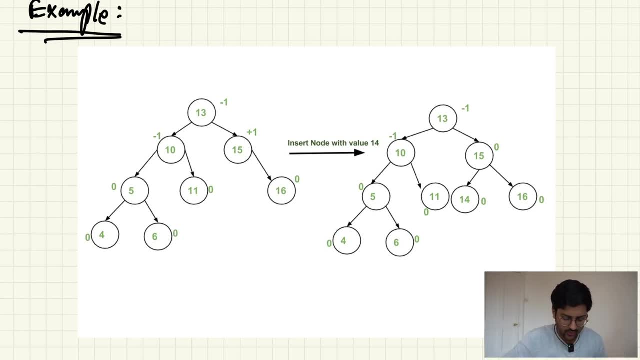 dirty, so this is looking much prettier. So here you can see- they have a tree over here and the node values. it says minus one plus one, zero, zero. these are just differences in height, so don't worry about that. Okay, We'll see it in the code when we do left heavy and right heavy, like how to calculate. 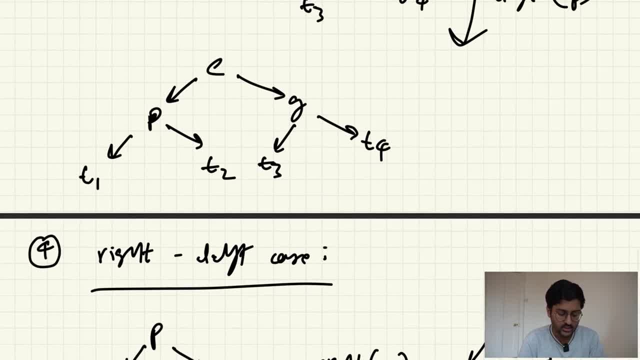 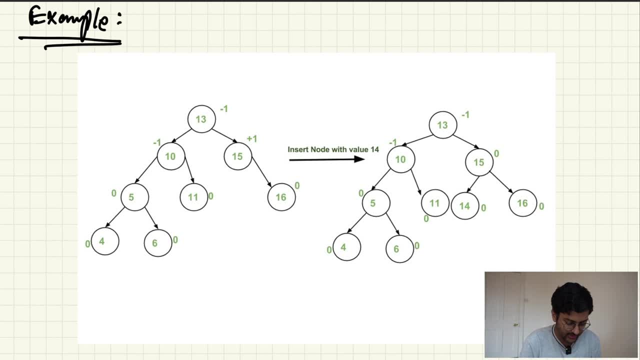 it using a formula. So when you see, okay, In these four cases, how are we going to write that in code? We'll see that in just a minute, don't worry. So here you can see that this is the normal tree. 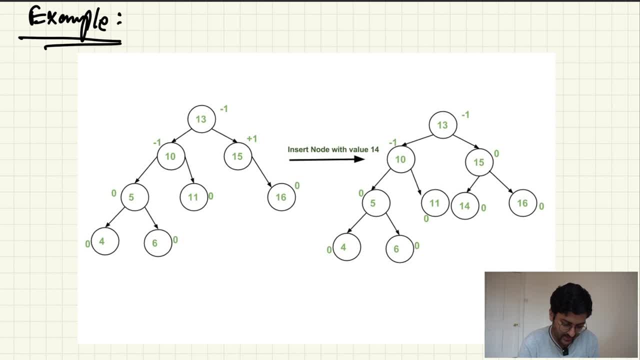 Okay, It is balanced. It's saying insert the value 14.. Okay, It inserted normally 14. in the left hand 15, as you can see over here. it inserted 14 over here, No problem, Did this make it unbalanced? 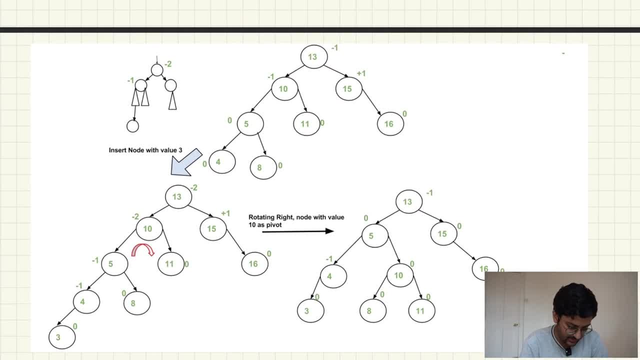 No, it didn't. Okay, Move forward. Now, here it says: insert three. So three is inserted over here, No problem, Three is inserted over here, but this three made it unbalanced. which subtree did it make unbalanced? Uh, four, four. 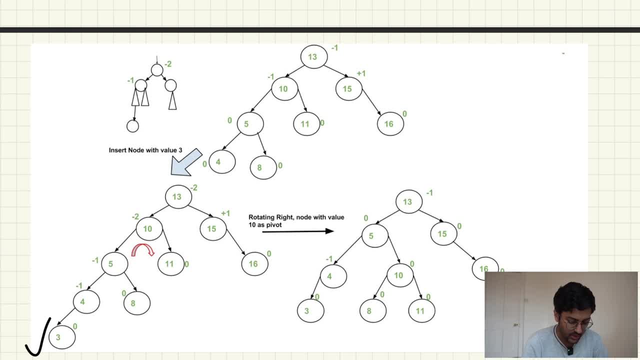 Did it make four unbalanced? No, Did it make five unbalanced? No. Did it make 10 unbalanced? Yes, This is actually the same case that we had previously, So it's going to be like: okay, this is parent, child, grandchild, parent, child, grandchild. 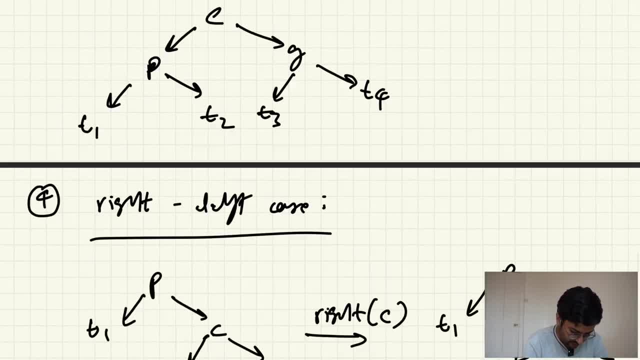 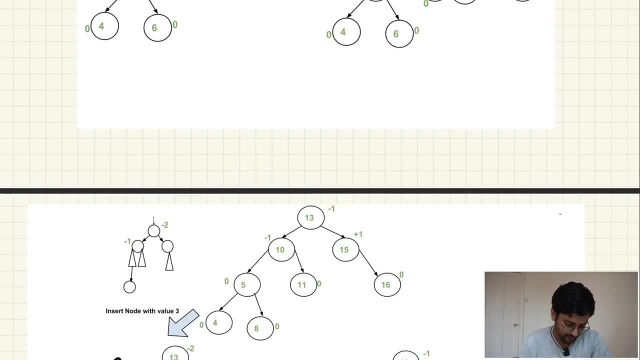 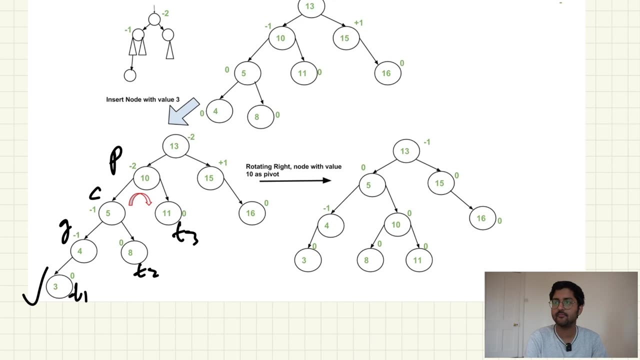 tree one tree, two tree, three. What is this case? This is parent, child, grandchild- tree- one tree, two tree three. tree four: right rotate, Right rotate, 10.. Done, Fixed. I hope now it's clear. 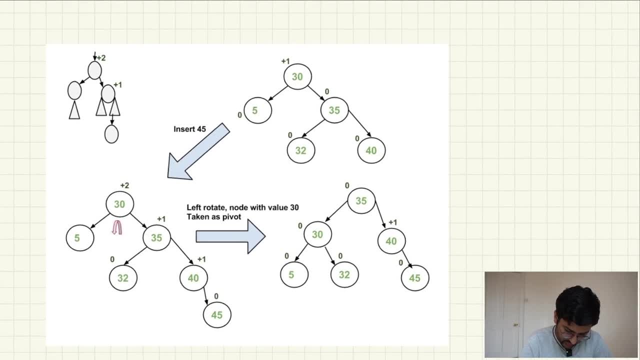 Now insert 45. In this example it will insert normally 45 over here, over here, No problem. Now this is making it: what unbalanced? Is 40 unbalanced? No? Is 35 unbalanced? 1 minus 0 plus 1, no. 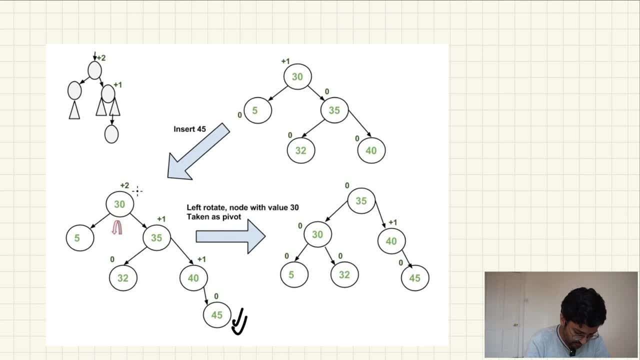 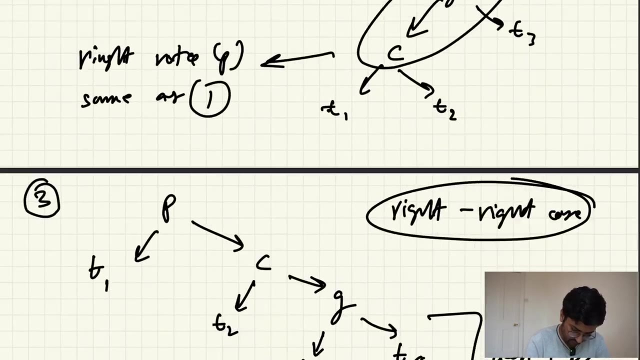 Is 30 unbalanced. Yes, 30 is unbalanced. So P, child, grandchild, This is right-right case. So right-right case means left rotate. Right-right case, left rotate. How simple is that? How simple. 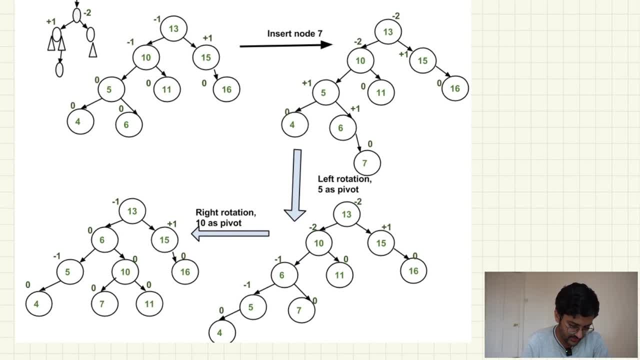 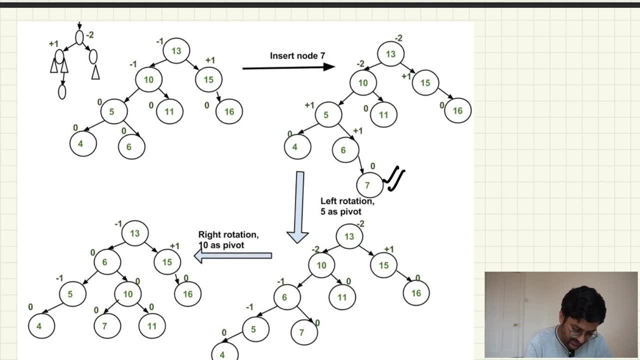 Cool. Now here it's saying: insert node 7.. 7 will go over here, No problem. So 7 is making which balance, which subtree unbalanced? 6? No 5? No 10? Is it making 10 unbalanced? 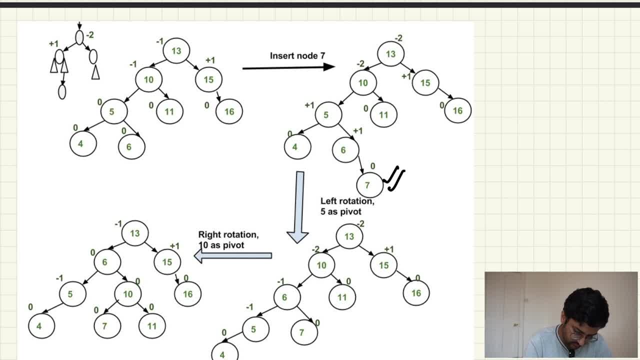 Yes, it is making 10 unbalanced, Because this height is 2.. That height is 0. So minus 2.. So it is making it unbalanced. Ok, So here it is saying: insert node 7.. 7 will go over here. 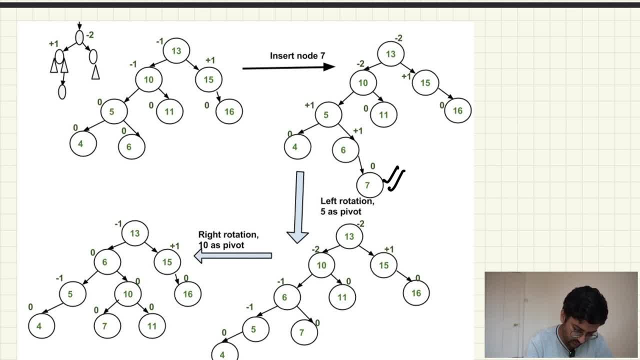 No problem. So 7 is making which balance, Which subtree unbalanced? 6? No, 5? No 10.. is making it unbalanced? 0 minus 2 is 0. this is 2. see 1, 2 and 0. you know how it. 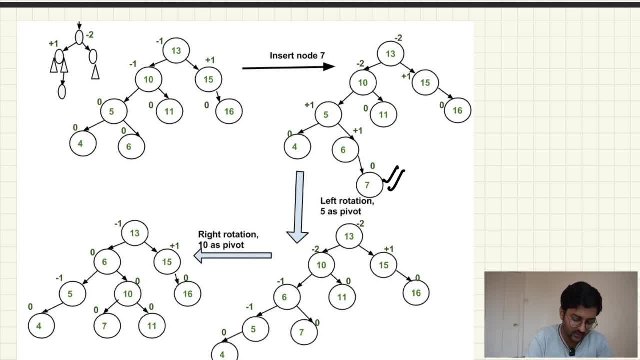 is 0 right height for every sub tree. so height for this is because this is only one node, 0 how it hide for this. 5 is what? 1, 2 so 2 minus or 0 minus 2, if you're doing right minus left minus 2, so 10 is unbalanced. so if 10 is unbalanced, 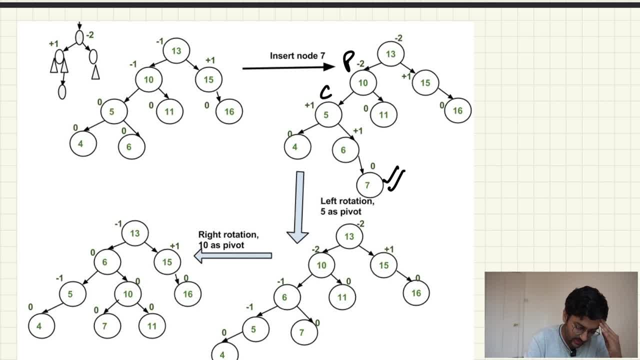 then this is P, this is child, and is this going to be grandchild or this going to be grandchild? grandchild is in the line of the number that is already added. right now, 7 was added. so in the path of 7 to P, in the path of 7 to P, the one. 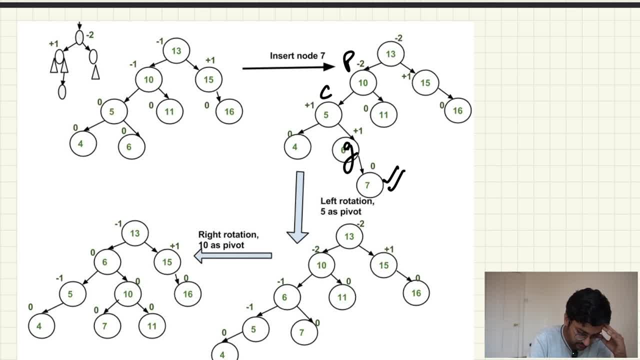 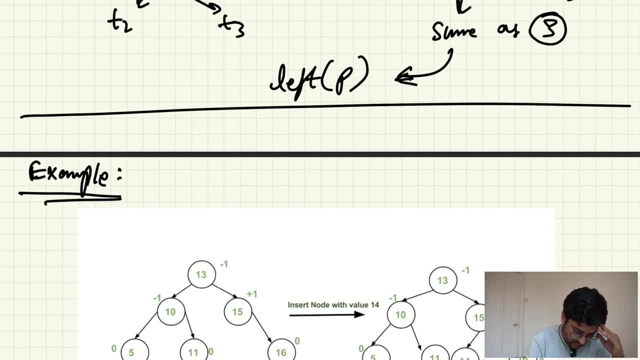 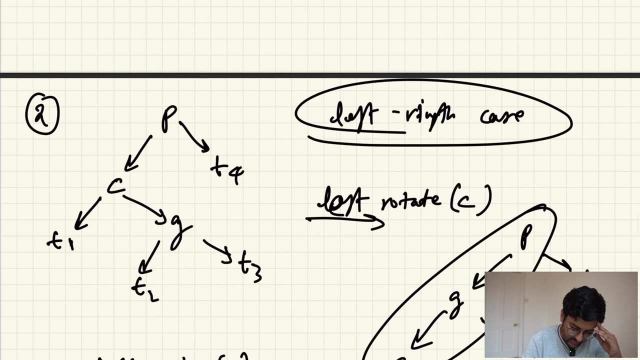 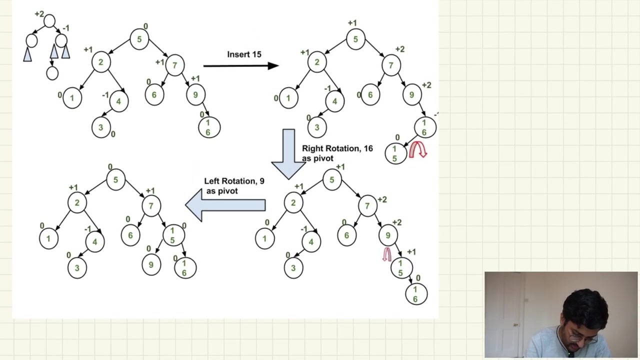 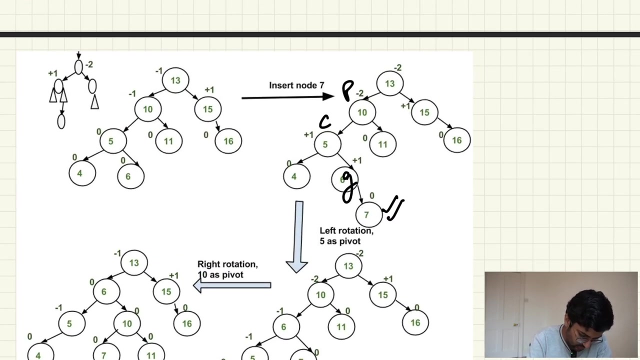 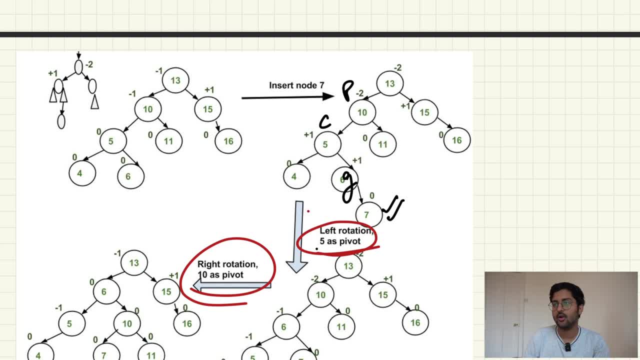 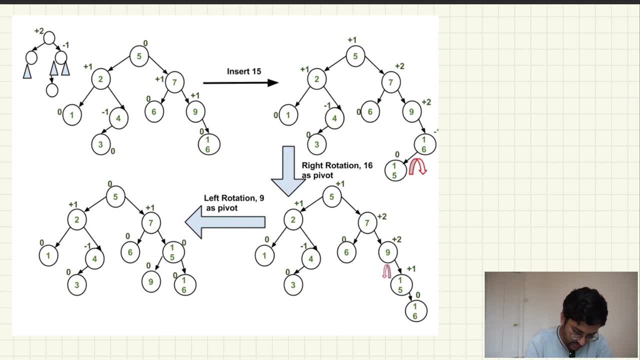 right rotate on 10, right rotate on 10, not a problem at all. very simple, very simple. similarly, now this case: insert 15: 15 is added over here. okay, is it making 16? insert 15: 15 is added over here. okay, is it making 16? 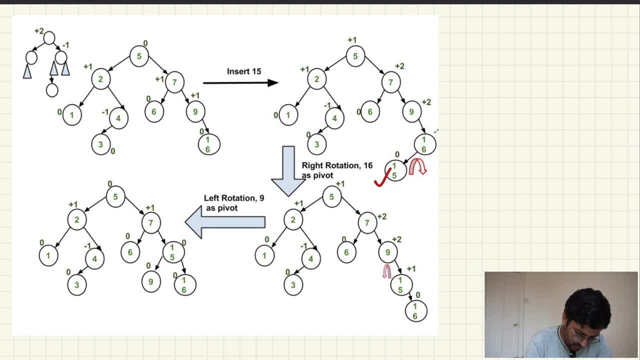 unbalanced? no, nine unbalanced, no, no unbalanced, no, no, actually wait. is it making 9 unbalanced? actually wait. is it making 9 unbalanced? yes, it is making nine unbalanced. because left height is zero, right? haha you this. because left high T0, right high T, it is no left. 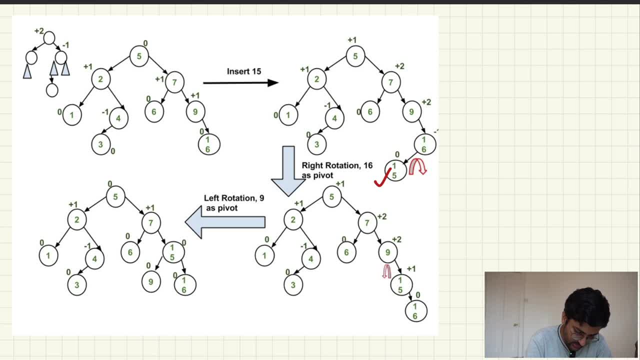 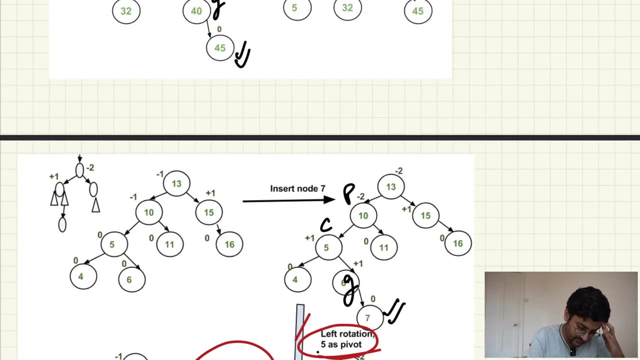 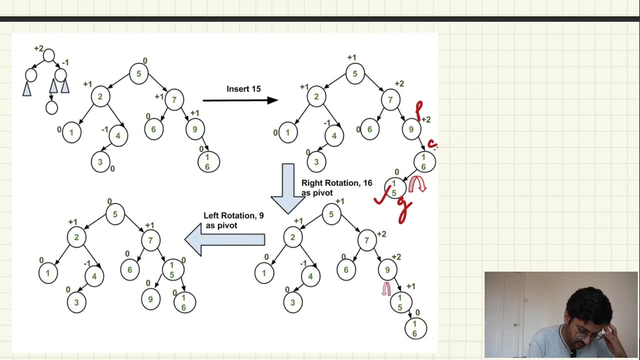 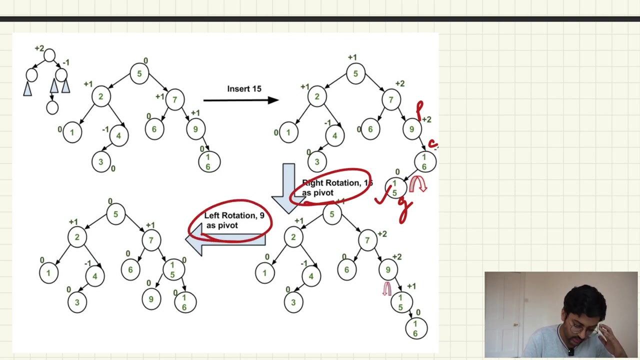 height is no, nothing. and then the right height is here one, so it is actually two. yeah, nine is unbalanced. so P, child, grandchild. so this is right left case. so in right left case, right rotate, C, left rotate, P, right rotate on 6, 16, yep. then left rotate on 9. yeah, T is balanced, cool. 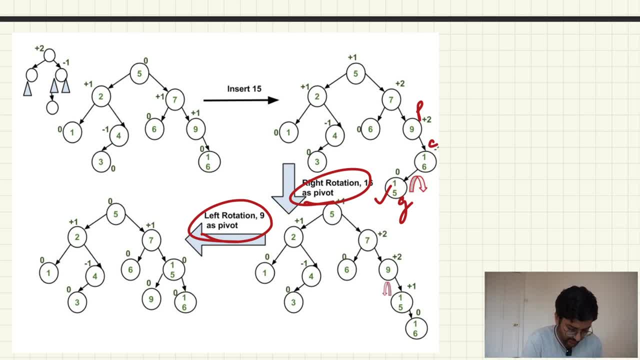 using these examples, I hope you understand that when you find a tree that is unbalanced, which is like this, you know, if you automatically solve this, then whole tree is salt, because originally whole tree was balanced as original, whole tree is balanced. this is the intuition behind it. this is where people 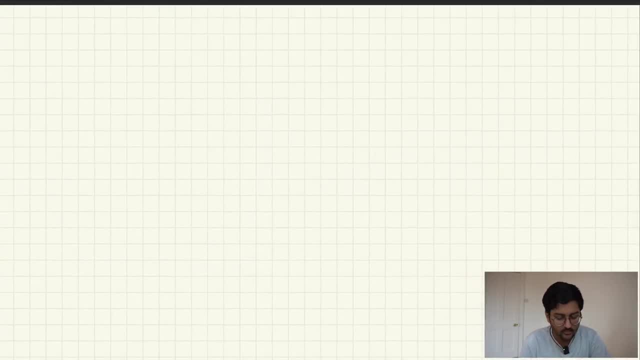 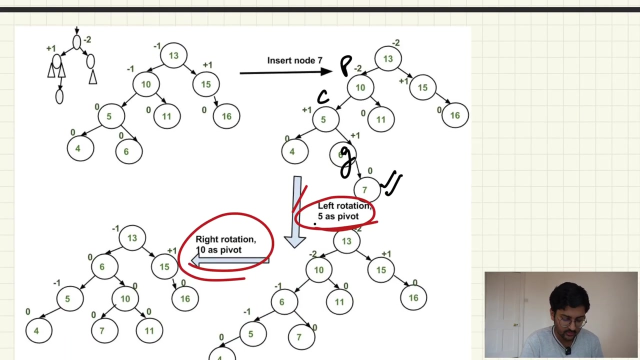 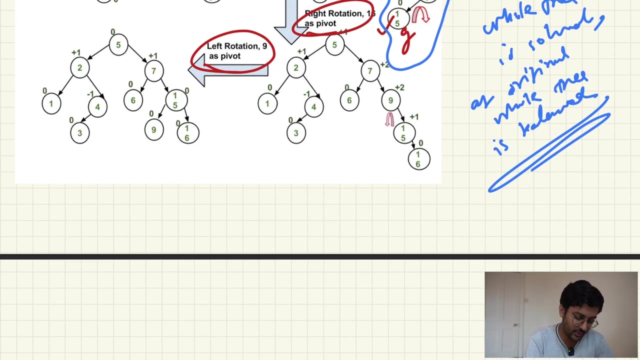 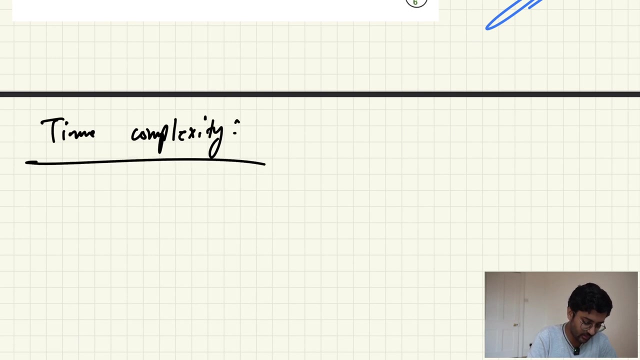 get doubt. so I believe I cleared that out. okay, sounds good, you all? right now let's call this. it's very simple, okay. so before we move on to the code, let me talk about the important part time complexity. time complexity, let's say we talk about for adding, because that's a performance function. 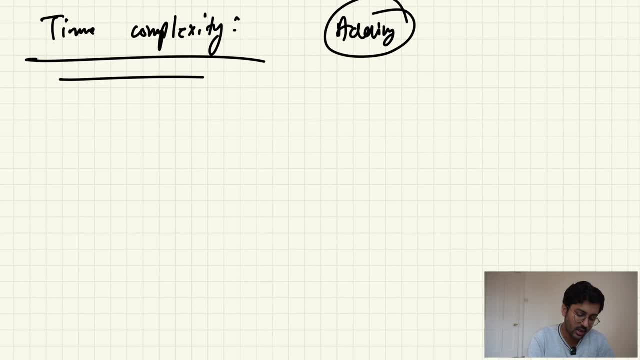 we are performing. so time complexity, because at all the times tree will be balanced in between time and complexity. to the time term it will be an variable problem. so it will be to the time when quantity 1 is the Waltz of the world, but at the time n of the world there are students interested. that's not quite to that point about time complexity, let's say so. at all the times 3 will be balanced, so it will be for a boundary, but beforebelieve it'll be there. we also need to multiply that. 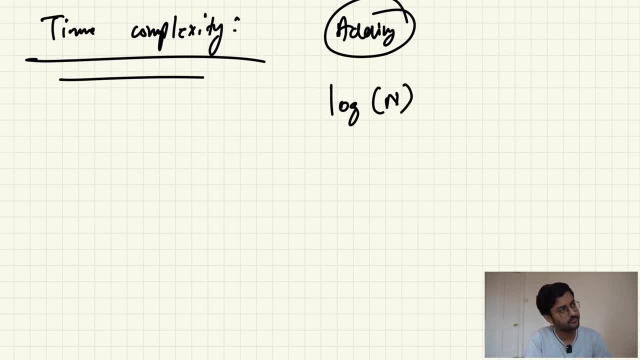 log of n. okay, log of n. can you tell me the amount of time, the time complexity that the rotation is taking? rotation is only at max two steps, either left rotate, light rotate or something like that. so rotation is taking constant time because i'm only rotating the subtree that was affected and since that affected will be fixed. 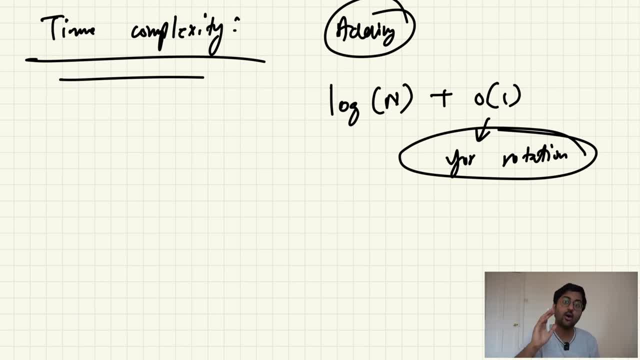 then all the trees will be fixed automatically, as i already told you, because the original tree was balanced and the rotation at max. we're just doing two rotations at max. that's what we're doing right, in left- right case or right left case. we are doing two rotations in left, left, right, right. 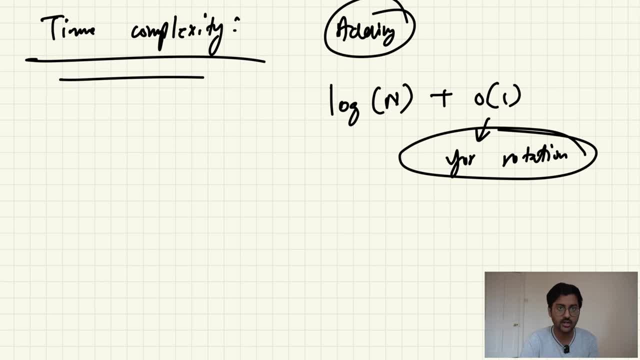 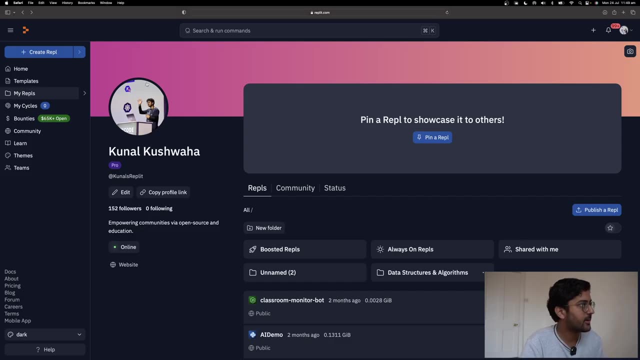 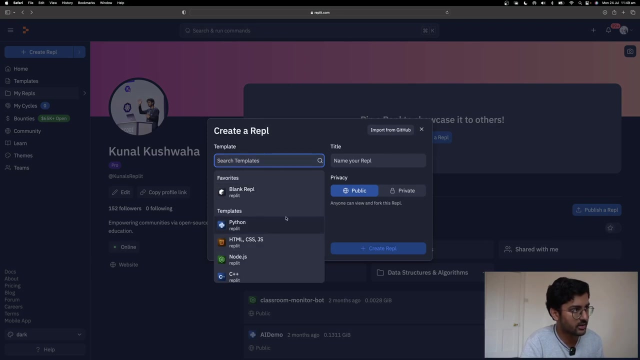 we are doing only one rotation to x, maximum two rotations, which is constant. so total complexity comes out to be o of log n. okay, you know we can code. all right, let's start with the coding part. you can check out the link to my code sample in the description below. that is going to be nice, because then you can directly run the. 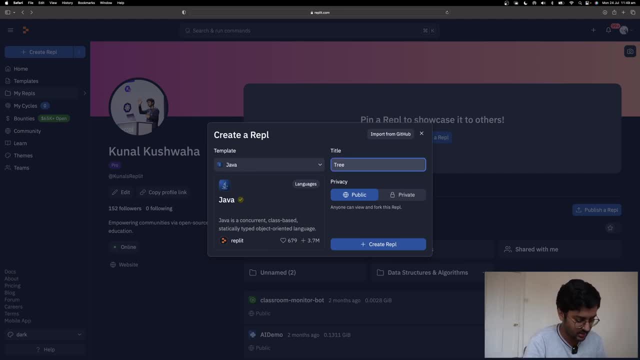 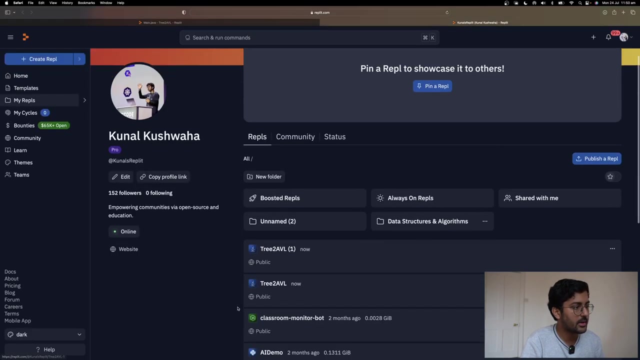 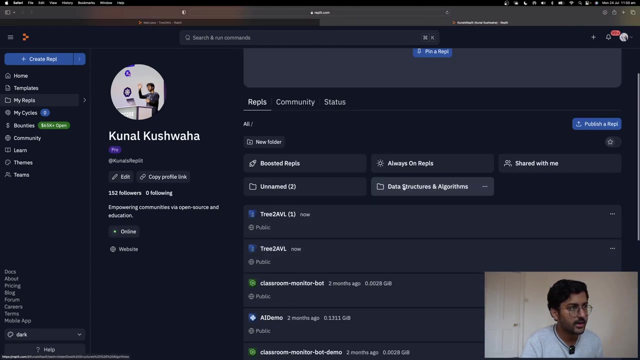 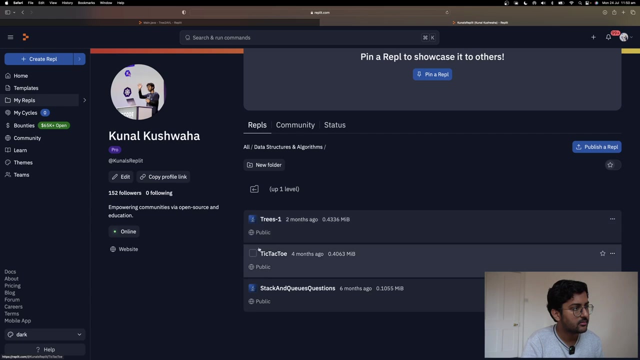 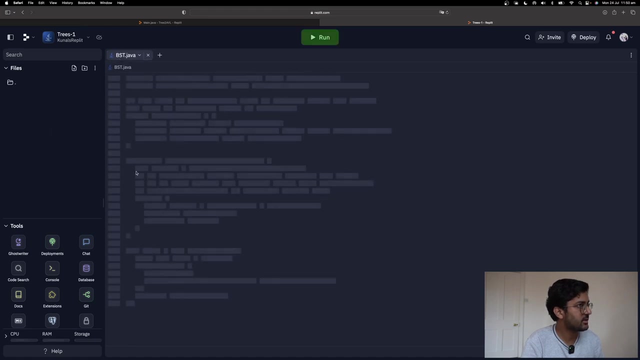 file on your browser. so i'm going to write tree to avl, create repl, and what i'm going to do is i'm actually going to copy paste my dataset algorithms. in the last one we did trees, so i'm just going to copy paste the binary search tree because we can use some of the functions you know. 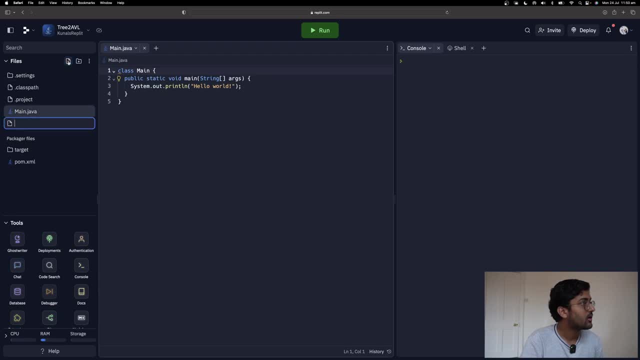 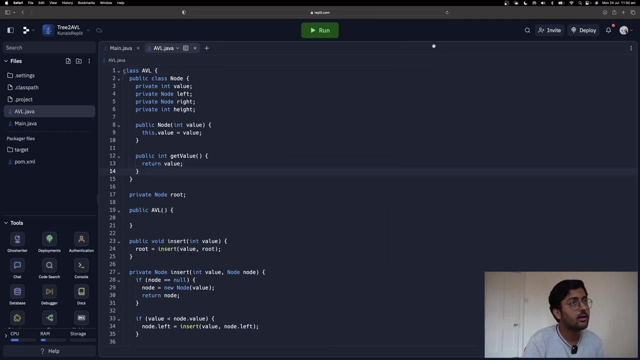 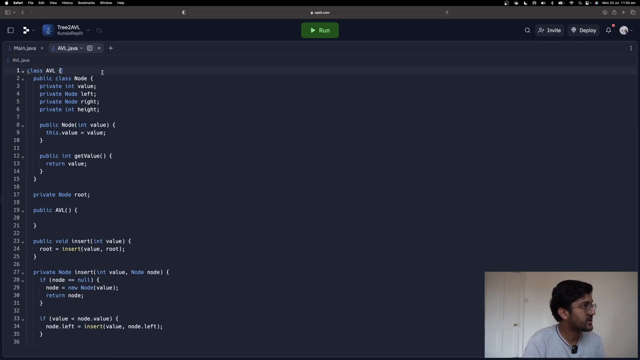 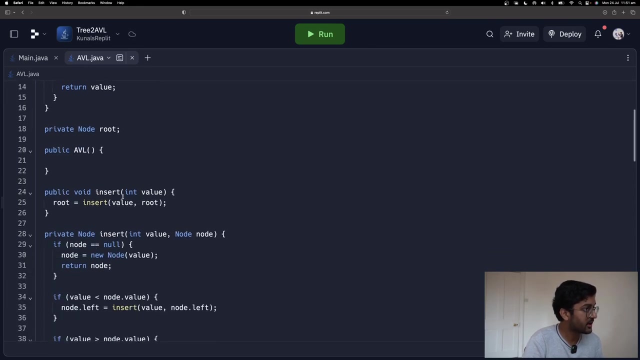 binary search 3: create avljava, copy paste it, avl, avl, hide it for now. and let me just double check, because whenever you copy paste, things can go a little wrong. so public class, node, everything looks fine. node root, root, fine insert. we will have to change a little bit, so don't worry about that. 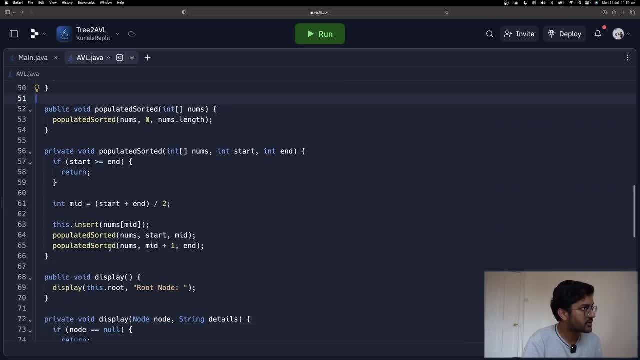 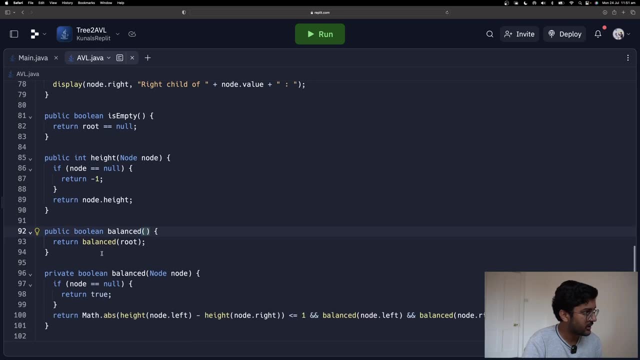 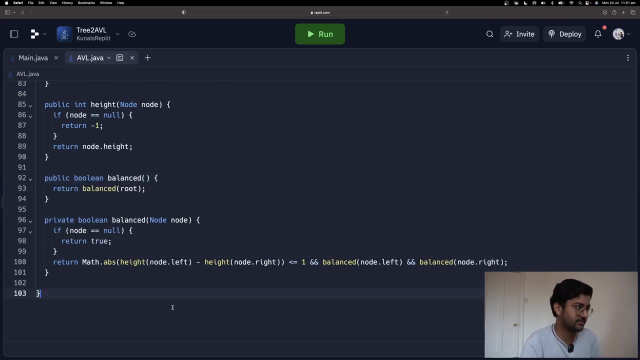 populate. populate with sorted is fine. populate with sorted is okay. display is okay, is empty okay. height okay. balanced is also okay, good. so if you don't know what these functions are, I mean you obviously will, because we just did, you know the tutorial, but this: 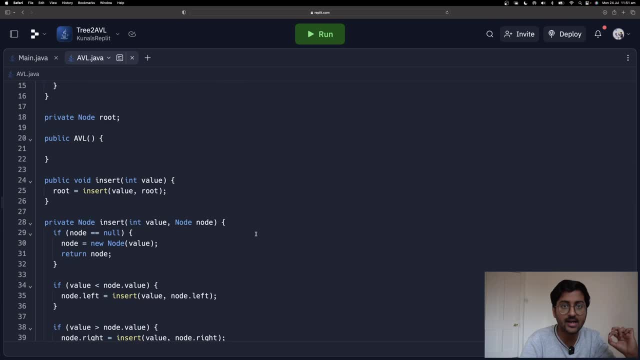 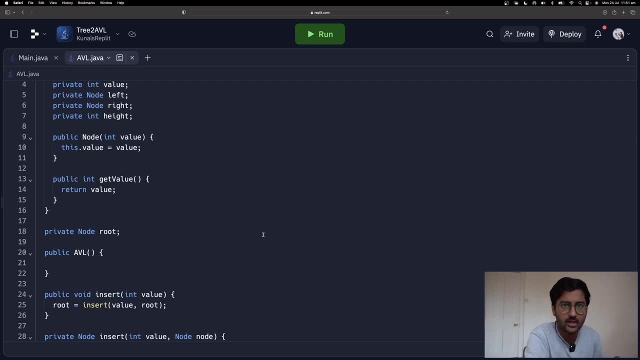 entire code. I have not just copy pasted. we did every. we wrote every single line of this code in the previous lecture. so please watch the previous lecture. you know it doesn't make sense. I write the same thing in again and again in every lecture. so every single line I have. 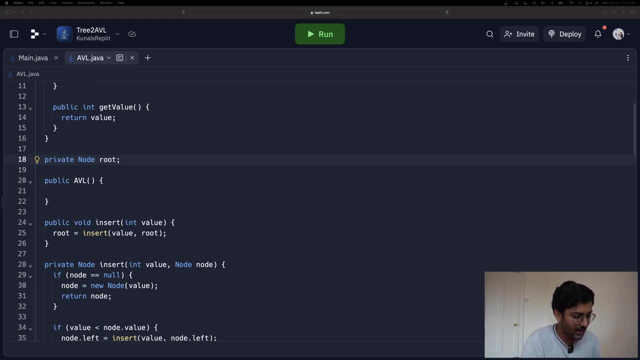 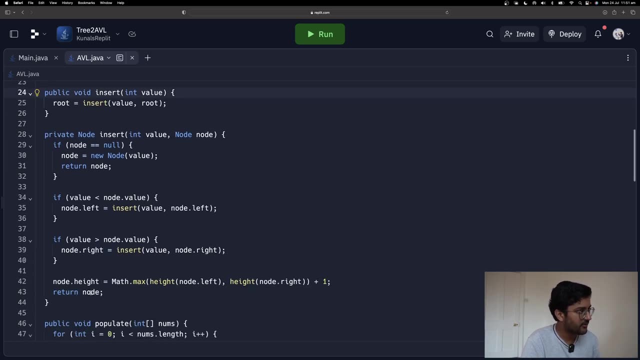 explained in the previous lecture. okay, now, what do we need to do? so we are inserting, normally, that is fine, but one thing we are changing is that we have to rotate this node that we have just entered. so this node that we have just entered, let's say, for root. 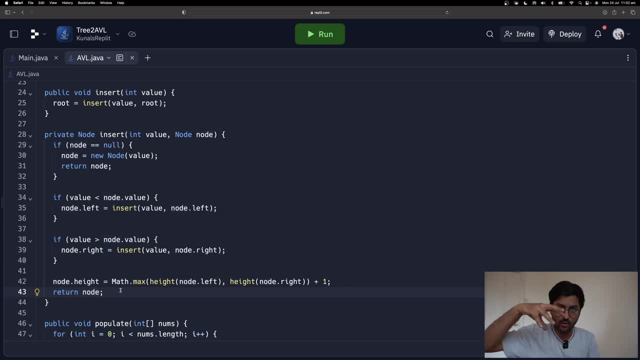 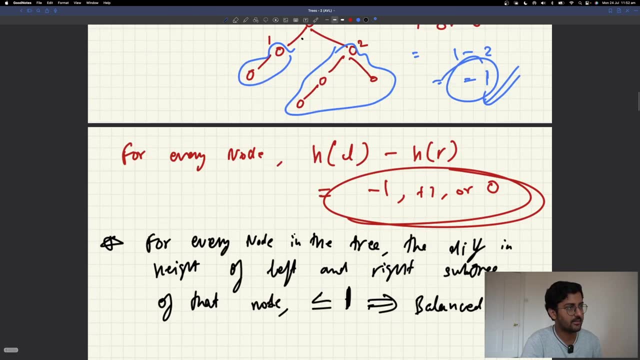 and it's going to in the end, when it goes down, down down. you know how the insertion works, right, so it's going down, down, down and in the previous example, like it will go down, it will go down, it will go down. then it will update it over here. so when it updates it over, 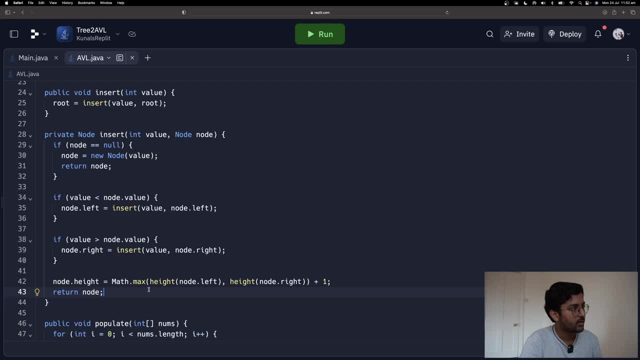 here I have to call this node in. let's say, I have to do what I have to do, rotate. so whatever, I will call a rotate on this node and this rotate is actually going to return the node itself, which is the root. so we'll go up and up and up and up. so, after rotating, so after it is done, 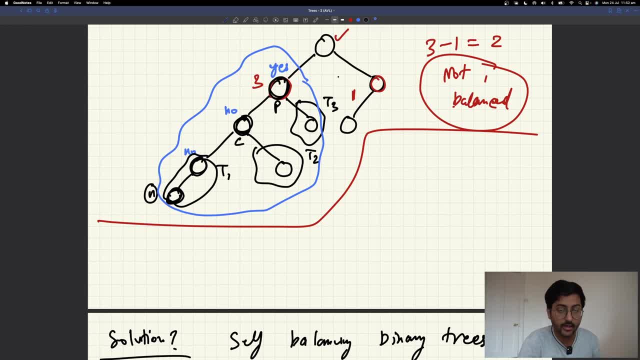 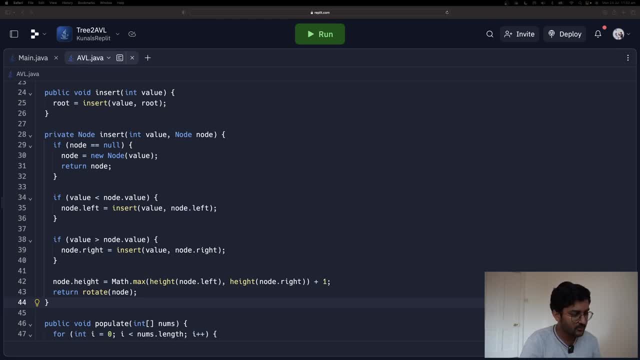 rotating. it will go up and up and up and it will rotate the root. sorry, return the root, okay. so that's the one thing we have to change over here and now. what I have to do is I have to create a rotate function. 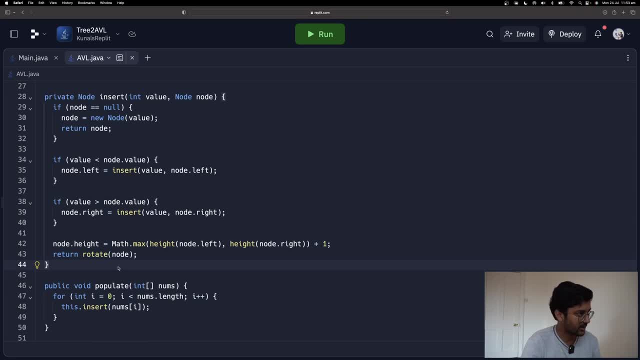 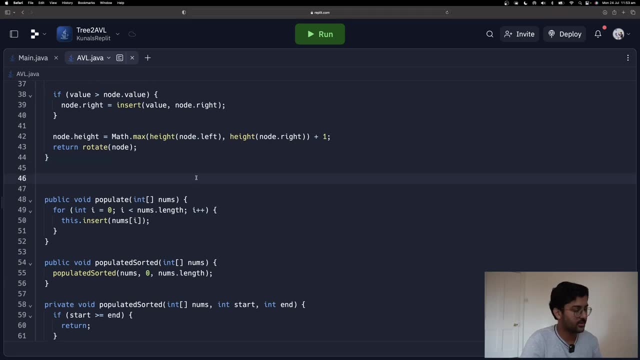 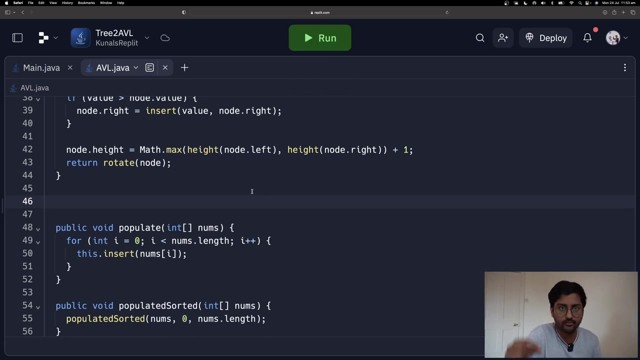 Okay, so let's see how we can do that. I'm going to turn off the AI feature, okay, I hope the screen is visible. the code can be found in the description below. you can directly click on run and you can run the code that I'm writing. so that's pretty cool. the link for this can be: 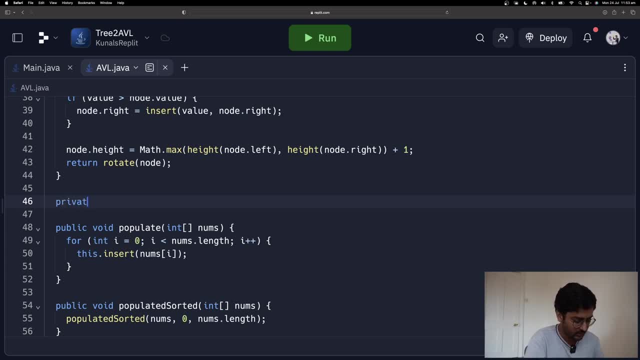 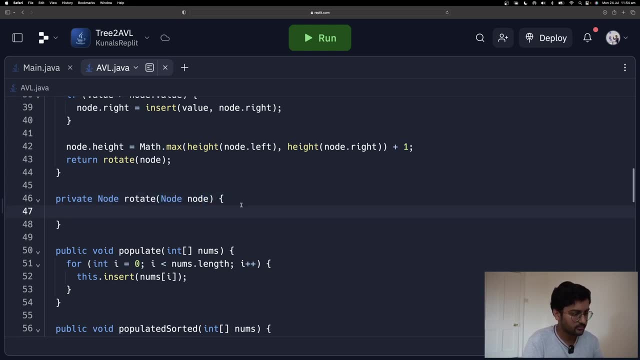 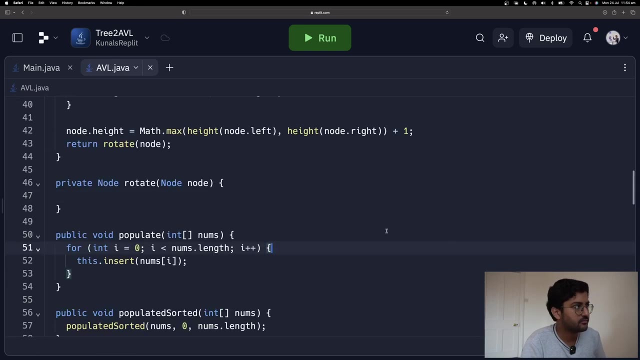 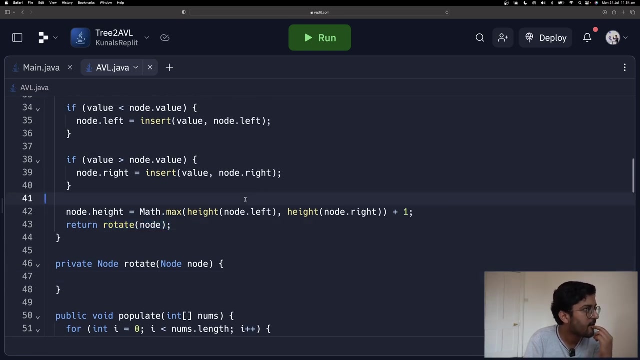 found in the description, just like every other link. so, private node, rotate node node. okay, we have to rotate, so no problem here. think about what is happening, Kunal. why did you call rotate over here? so when you're adding your node, in the end it's going to be like okay. 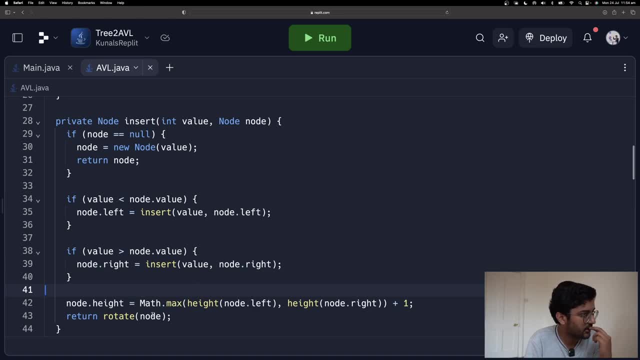 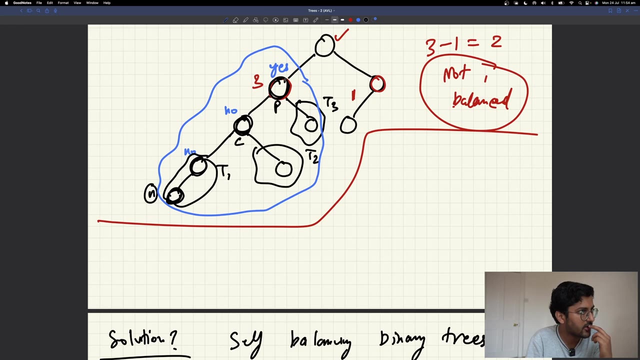 node is equal to the new node added, then return. so it's going to rotate that node. it's going to rotate this node and whenever you're trying to rotate and then it's going to keep on returning it like rotate on the nodes that I have called here in the previous part. 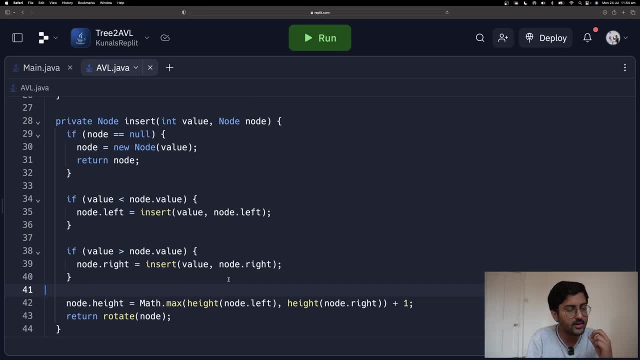 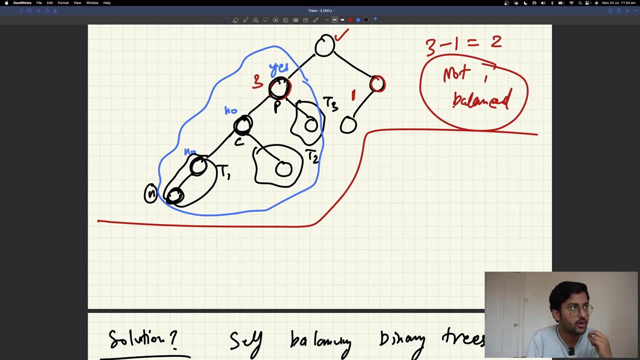 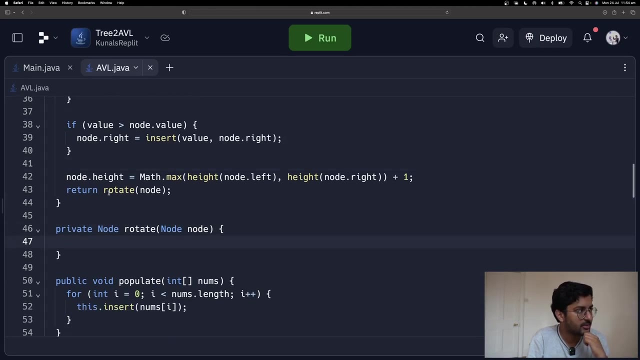 okay. so even though it keeps on calling it, it will not execute because these will all be balanced. there only be will be one node that is unbalanced. so how do we make that check? I hope that is this is clear. you can run it on pen and paper. you know recursion very good now. 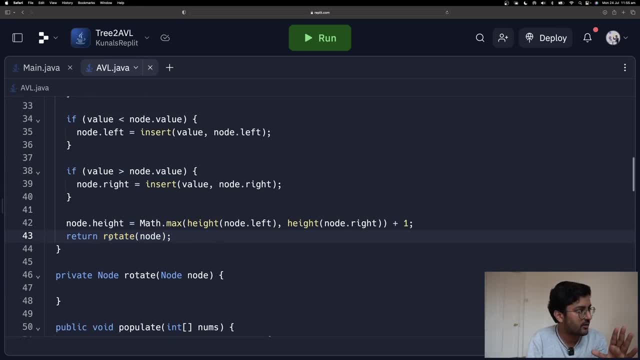 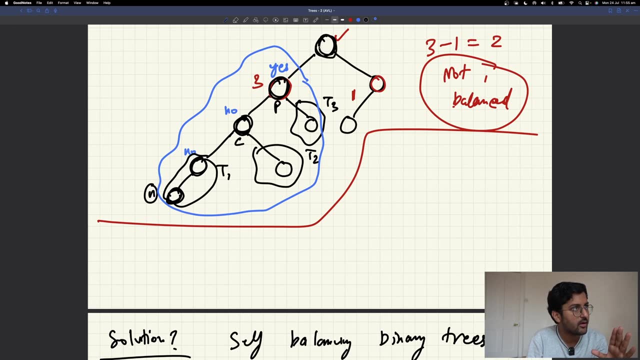 so I hope this is clear. please don't be confused on Kunal. why are you returning this node? I am in the end returning the. in the end it will return the root node only. okay, for every function call, first function call. 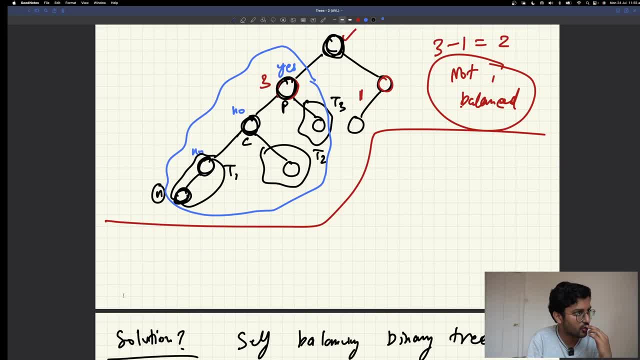 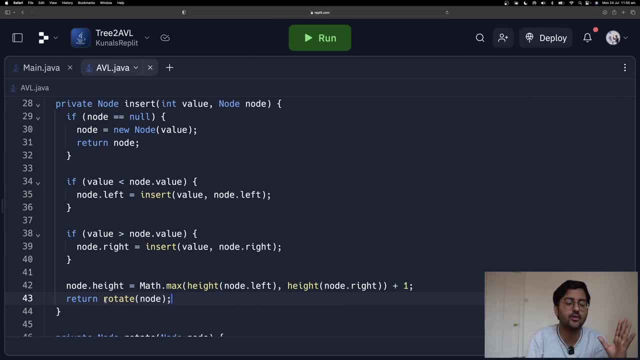 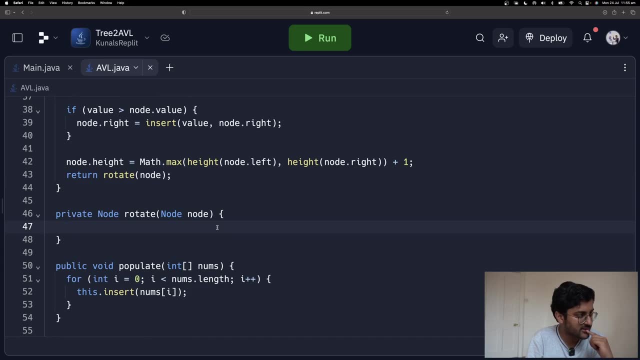 it is going to return the node and it will partially to rotate. rotate itself is returning the node only, so in reality it is just fixing the structure of the tree and then rotating the node itself. that is it private node rotate. so four cases. so one thing: I have to, I want you to. 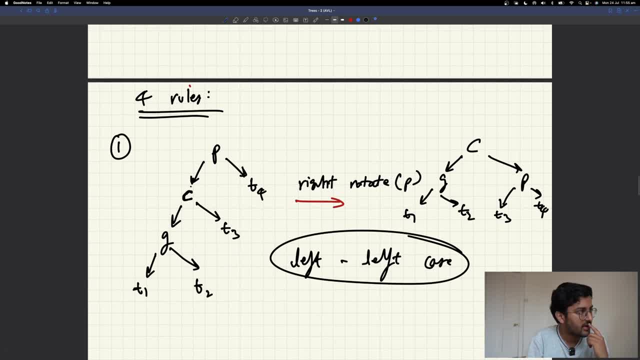 notice that in this case, when the height of- if you are on parent of, if you are on this node, if the height of left minus the height of right is greater than one, it basically means that it is left heavy because left has more height. very simple, so you will just do right rotate. 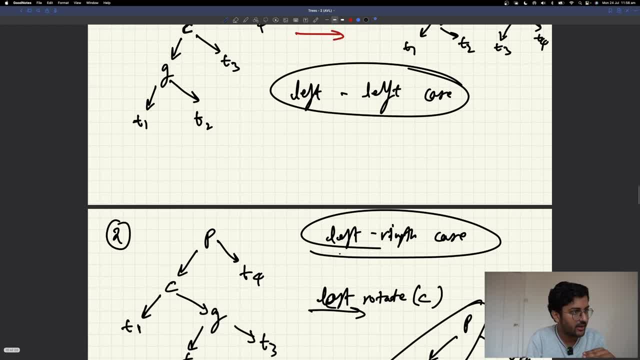 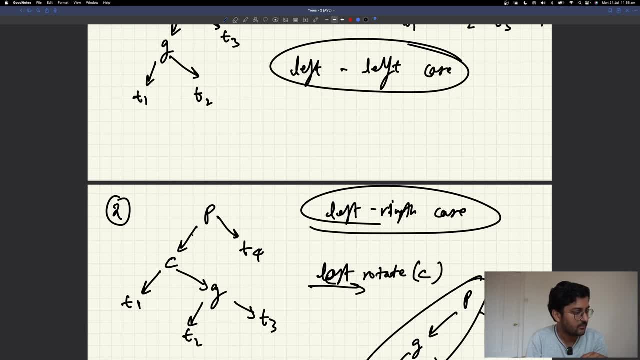 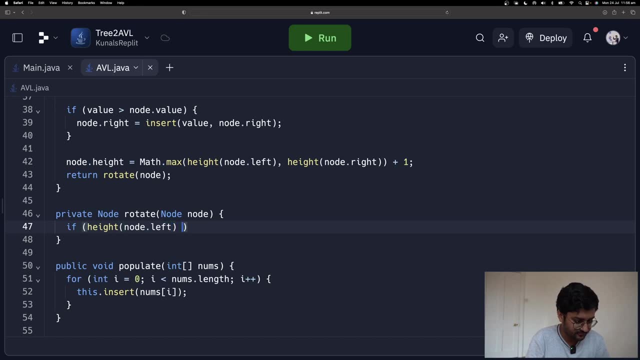 so left heavy is two cases, which is left left and left right case. so in left right case you can see. let me just write it down first. so if height of node dot left minus height of node dot right is greater than one, then I know that it is left heavy. 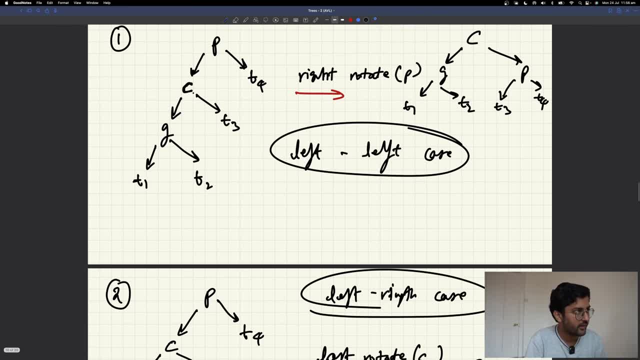 and now left heavy, has two cases. so if, if I take this child over here- if the height of node dot left, P dot left, dot left, if the height of this tree and this tree is positive, it means that it is left left case, because this is greater. so left left case. 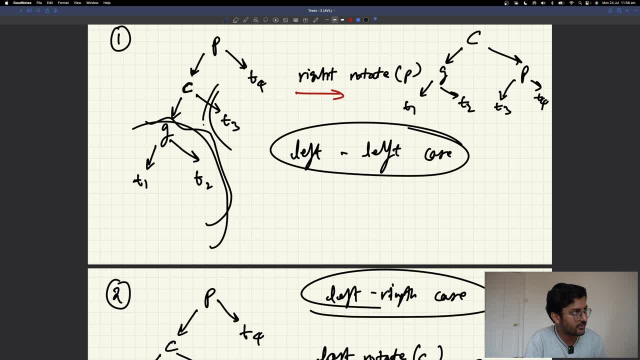 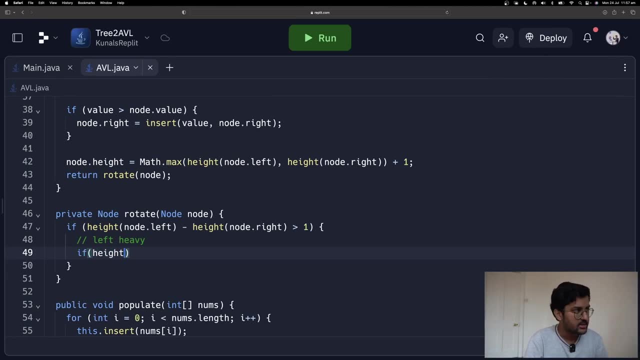 so left left case is: this height will be more, this height will be less. that is left left case, as you can see on the screen. so if height of node dot left, dot left and node dot left, dot right, see the thing is. don't try to think how these things are happening. 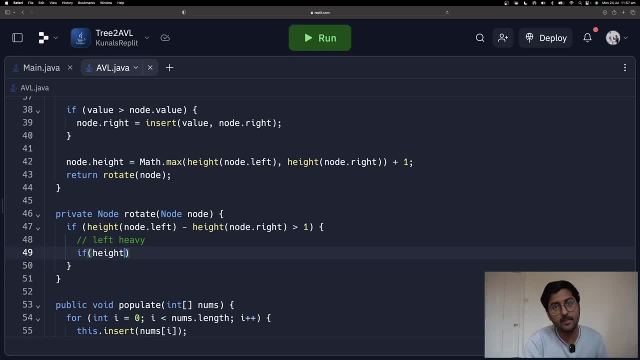 when it is right in front of your eyes. this is why in linked list many people get confused. in linked list you get questions like: okay, every three items you have to reverse, or whatever. so when you are debugging it and writing it down, and it is, the diagram is telling you. 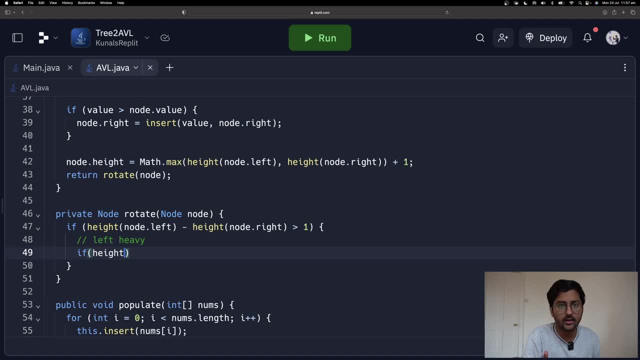 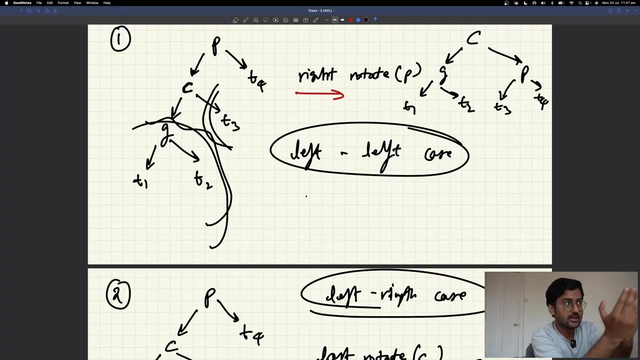 where all the arrows will go, then why do you need to think? there are two types of problem is in which you have to think. other type of problems like this are the visual problems. the diagram is telling me what to do. there is no intuition behind it, okay. 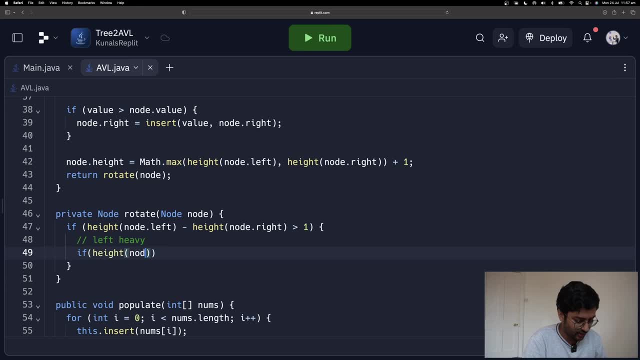 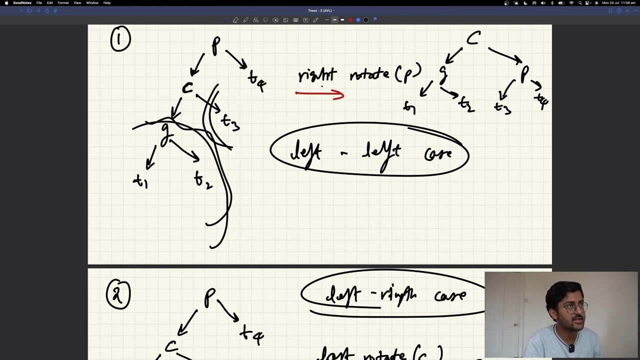 whatever the diagram is saying, I am doing so if height of node dot left, dot left is minus height of node dot left, dot right is actually positive. in that case- I know it is left, left case- What is the answer? in left, left case, right rotate on p. p is node, so right rotate. 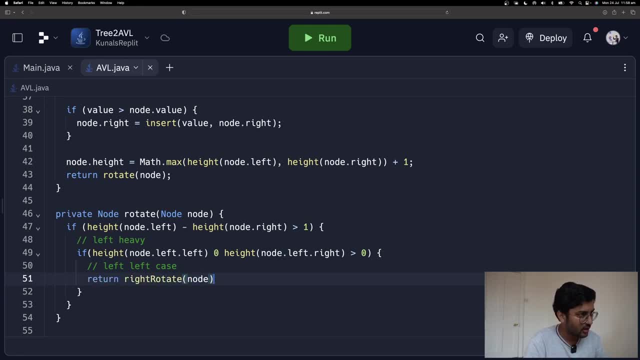 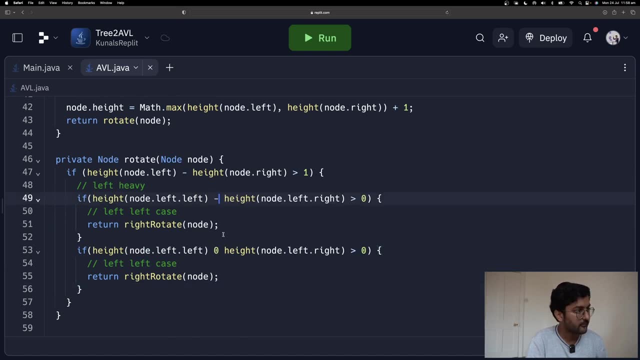 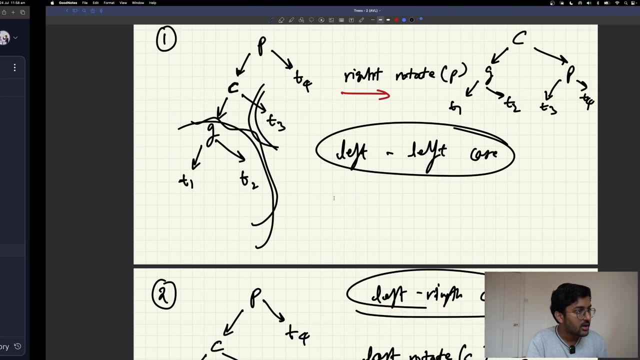 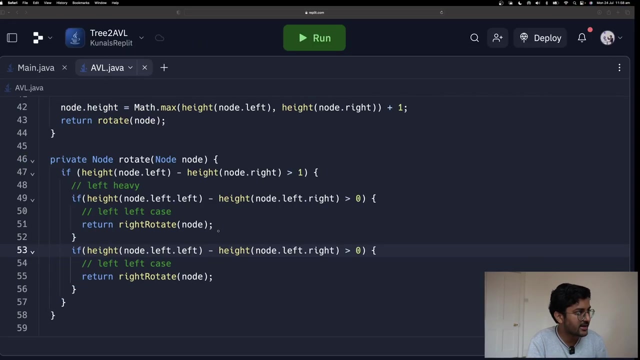 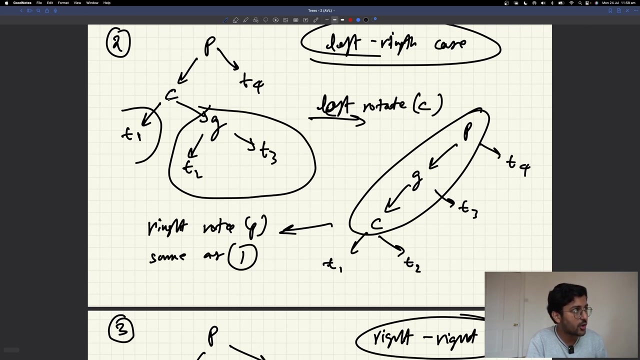 right rotate. I will clear it later on node. similarly, if this is negative meaning this height is greater, this height is smaller means it is left right case and left right case. we do what left rotate on child means node dot left. so we do left rotate on node dot left. 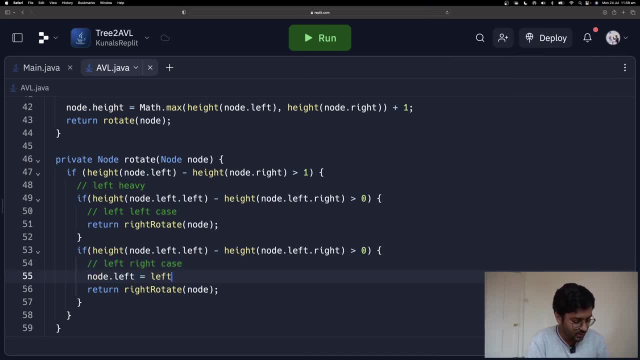 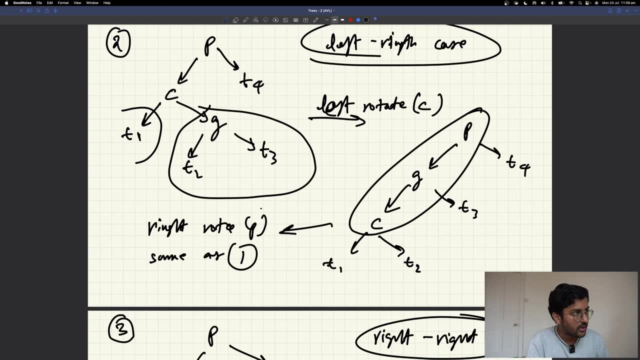 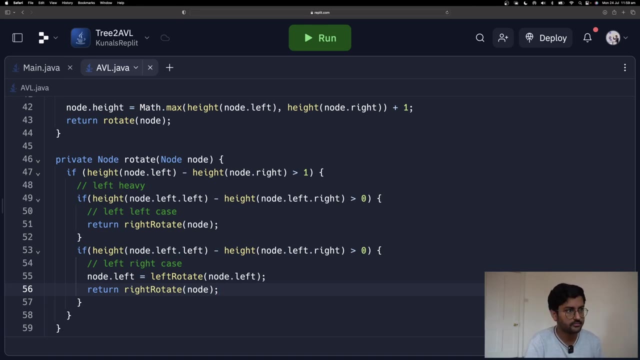 node dot left is going to be equal to left. rotate node dot left and then return right. rotate on the original node. right rotate on the original node. no problem. No problem at all. it will actually be equal to. if this is negative, make sense very simple. 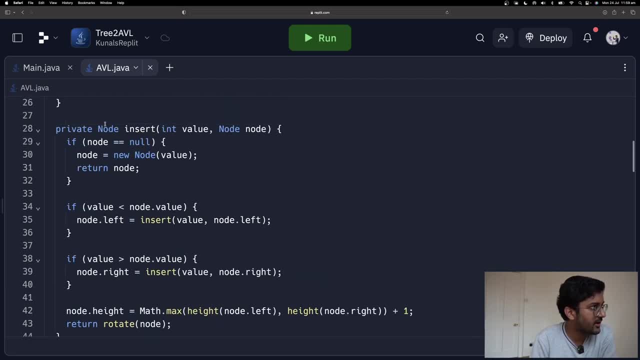 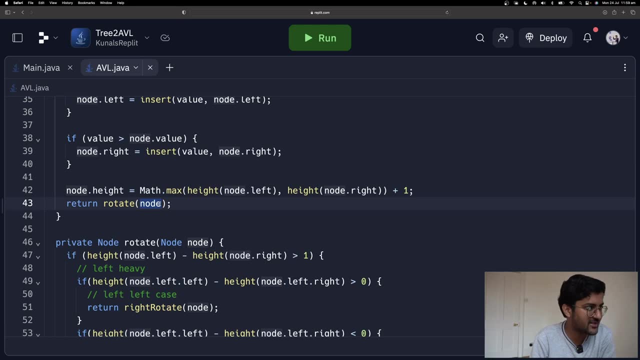 in recursion you will understand. in recursion I told you, if the return type is node, then you are going to be returning node. so if you are trying to fix it for this node, if you are trying to fix it, then this function is actually should also return the type node. 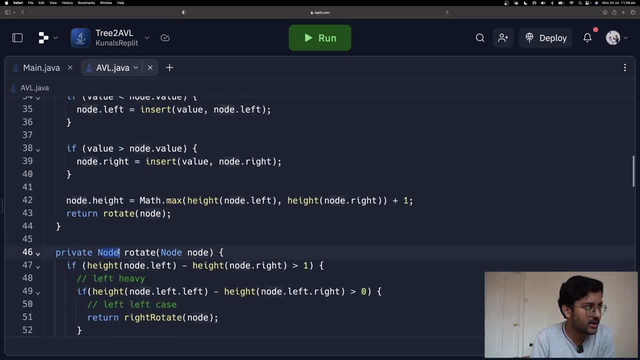 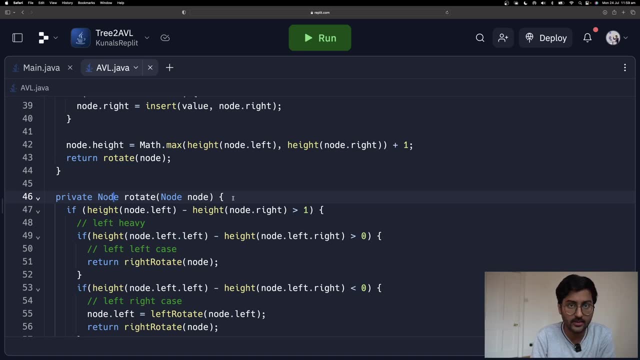 because this function is accepting node. that is why it is returning node, otherwise it will give you error. it will not even let you, you know, compile or whatever. so if you debug it, you can debug it on pen and paper. 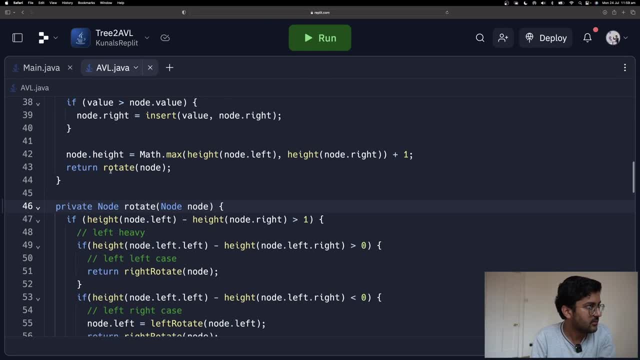 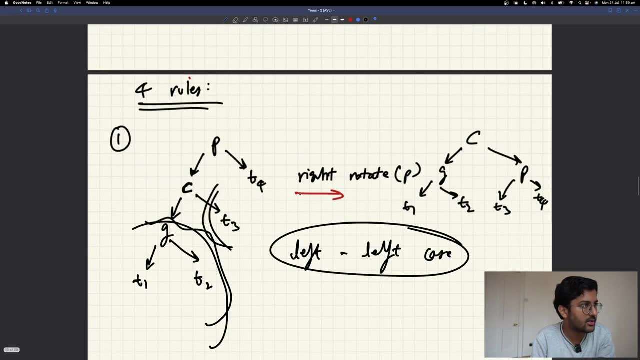 I showed you the entire thing. when I add it in over here, it is going to say like: okay, new node, added return node. so it is going to call the node for this one. call the rotate for this one. 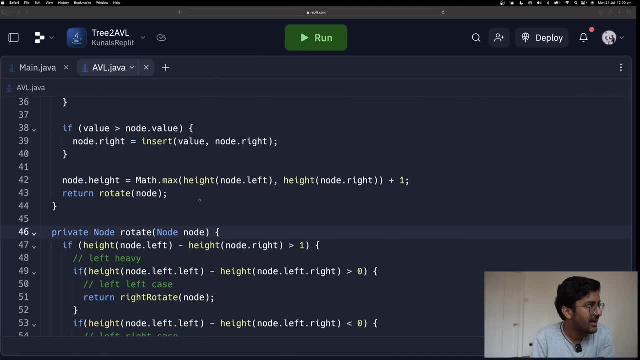 for this one. it will not execute because none of the conditions will satisfy. hence it will come out of here. and when it will come out of here, it will be like: okay, either over here or over here. 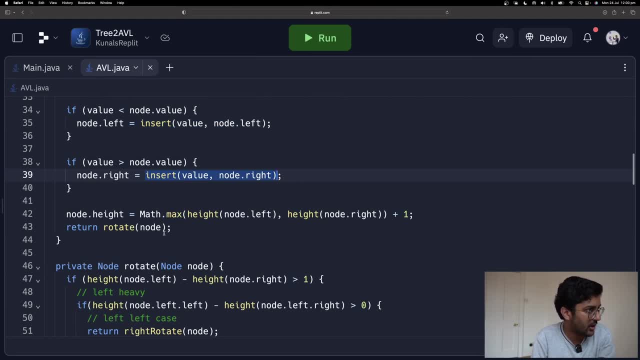 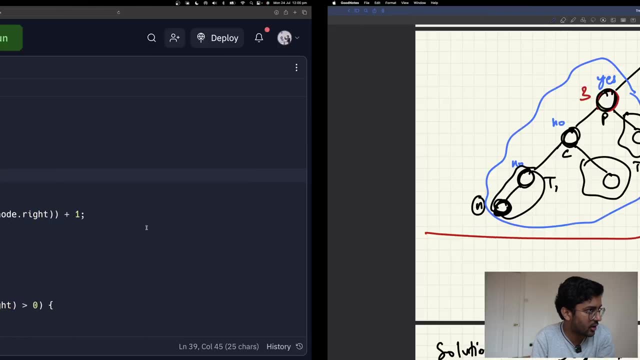 so it comes out over here, then nodeleft will be equal to whatever it was. so nodeleft will be equal to whatever it was, unchanged, and then it will be okay. I am not going to call rotate for this. 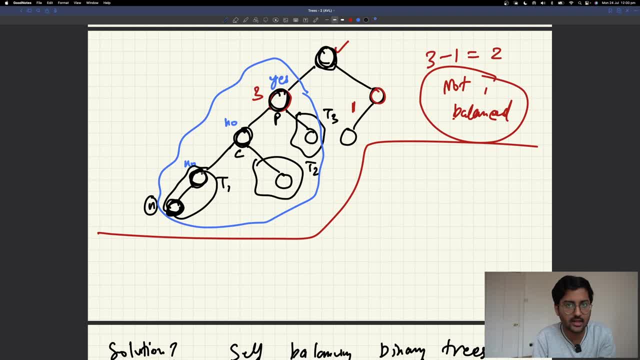 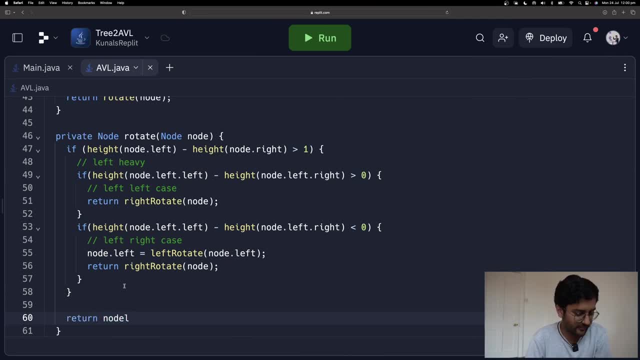 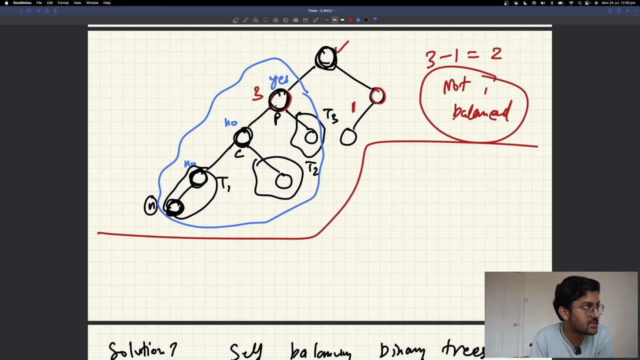 call rotate for this. it is going to say, okay, this does not satisfy the condition, so no worries, I will just return the node normally itself. return the node normally itself, and this will either be returned from here or here, so it will be like noderight. nodeleft means cleft, so for this node, 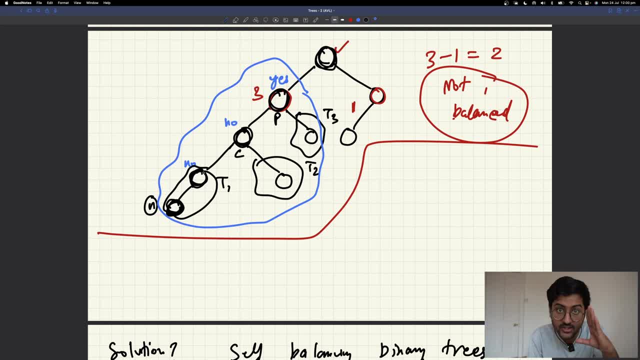 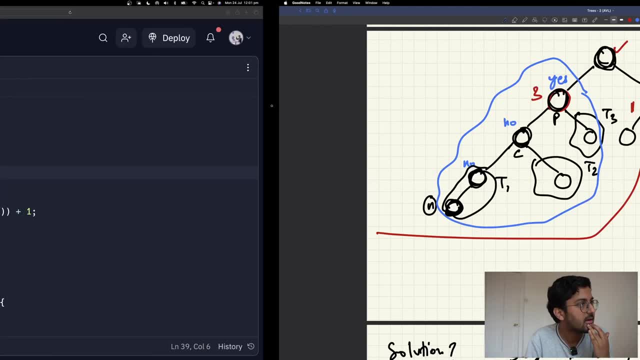 in recursion, nodeleft will be equal to this, only so. remaining unchanged, as you can see, remaining unchanged. I told you I won't show you the pen and paper stuff, but I am still doing okay. so now this for p. 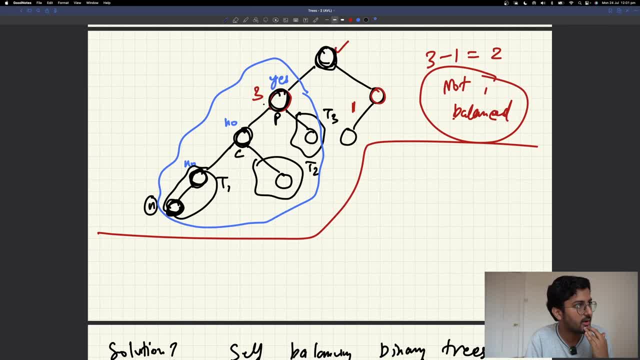 it will be like, okay, rotate it. so it is going to be like, okay, is this unbalanced? it is going to be like, yeah, then it will rotate it normally, and then whatever the node is supposed to be over here. 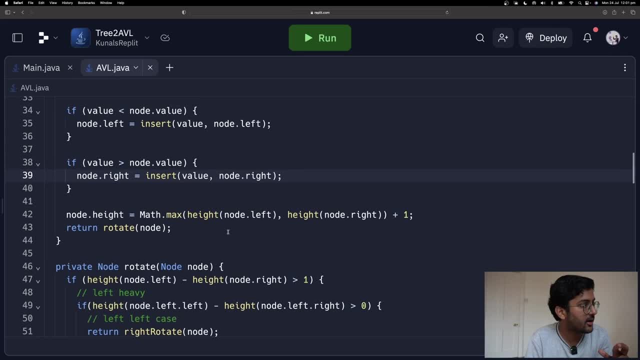 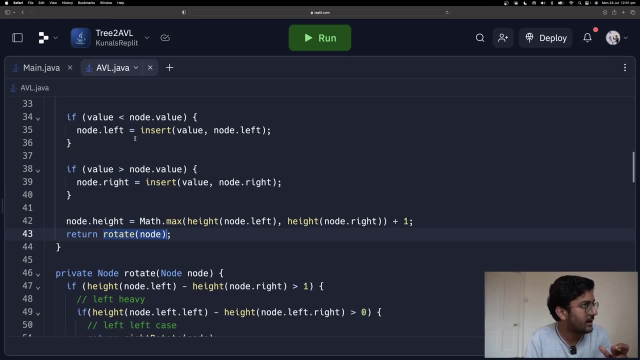 which is going to be child. it is going to return that and where it will return? from where it was called. so return the child that we have over here and it will be called from here, so it will return over here. 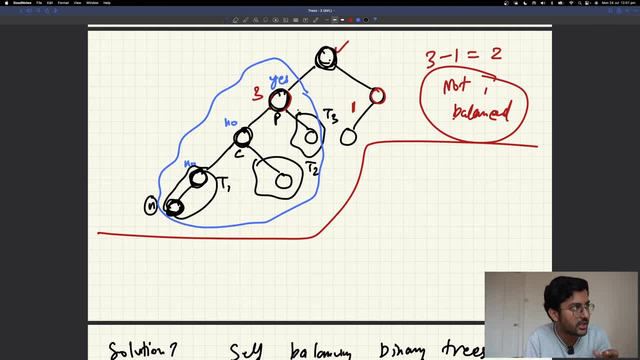 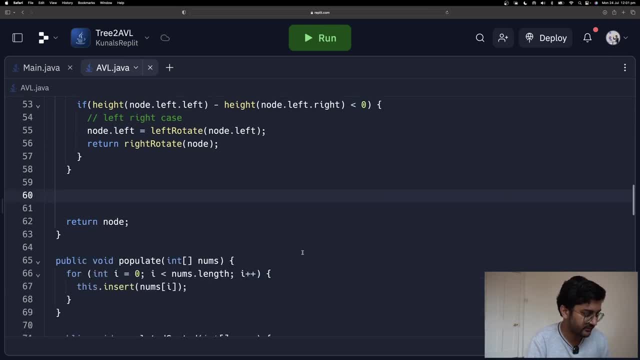 so this nodeleft will now be equal to child and this tree will be rotated. okay, cool, use the pen and paper. you will understand this is very simple stuff because we have done such questions before and I showed you the problem by running it also. 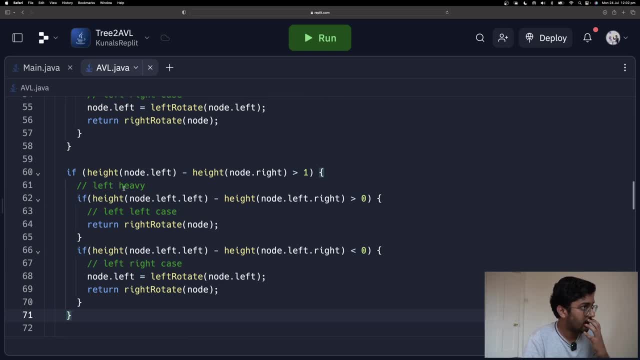 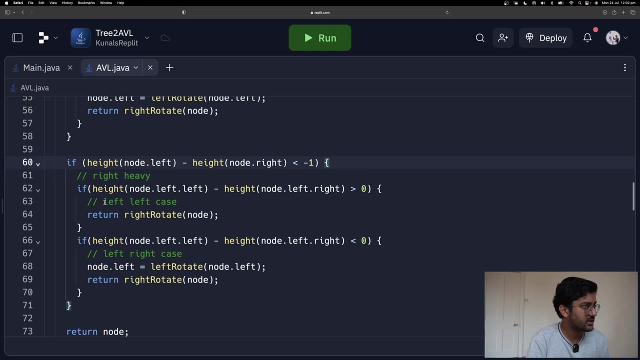 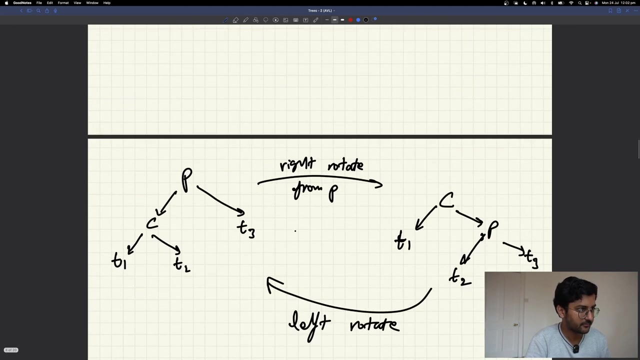 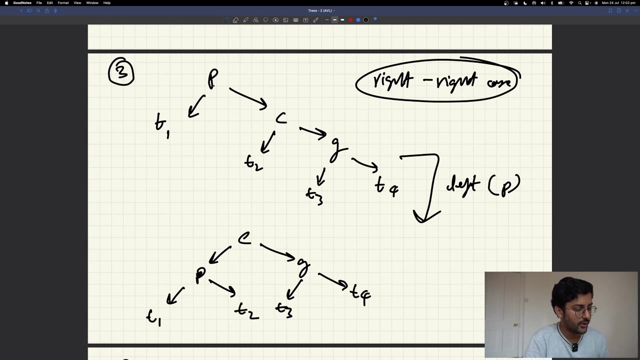 copy paste now. write heavy- write heavy is when this is actually less than minus 1, and write write case will be what node dot, node dot, write, write, write case. let's check the write write case. write write case. okay, node dot right dot left and node dot right, dot right. 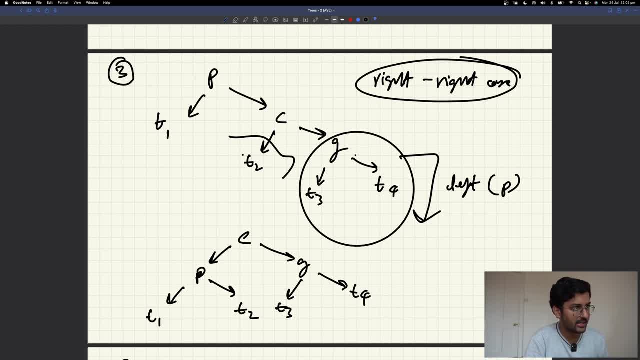 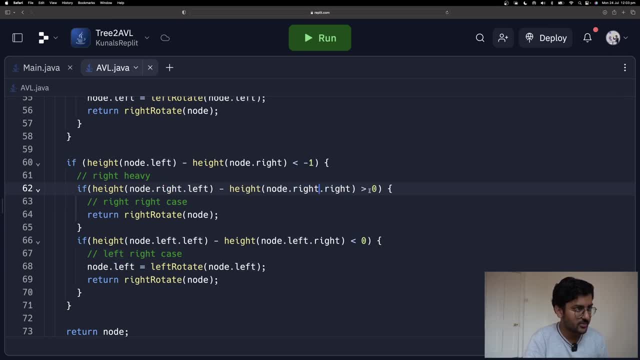 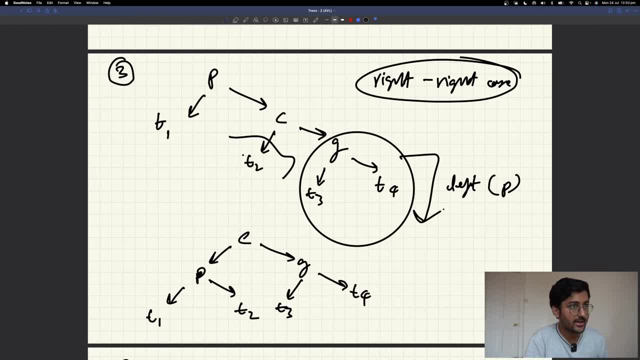 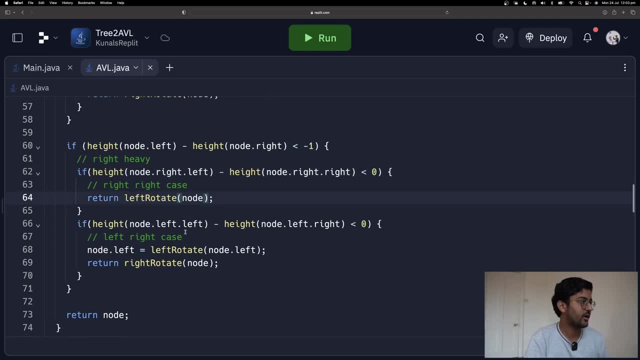 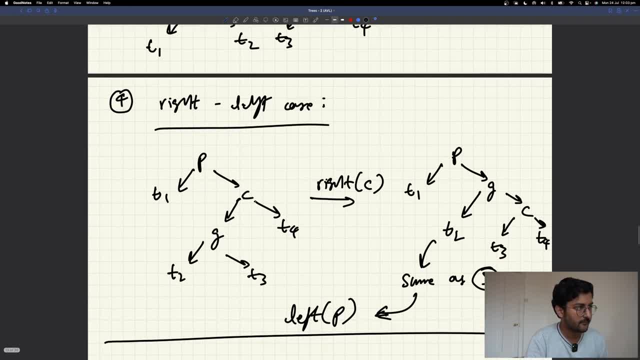 so node dot right, dot right should be negative. so node dot right, dot right should be negative. so node dot right, dot left should be negative. so node dot right, dot right should be positive. so node dot right, dot right should be positive. 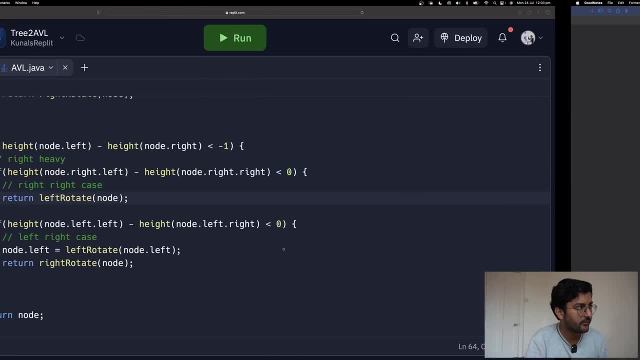 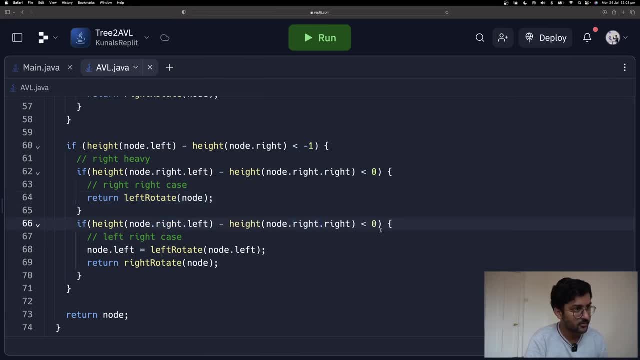 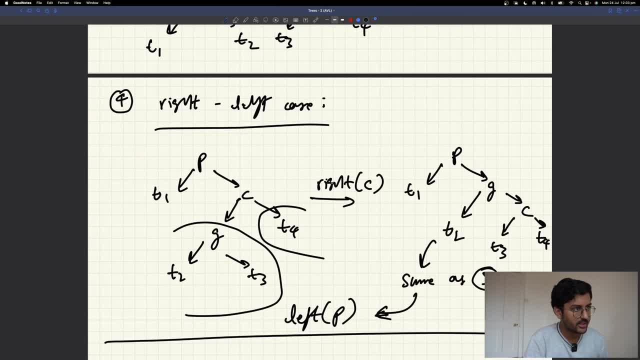 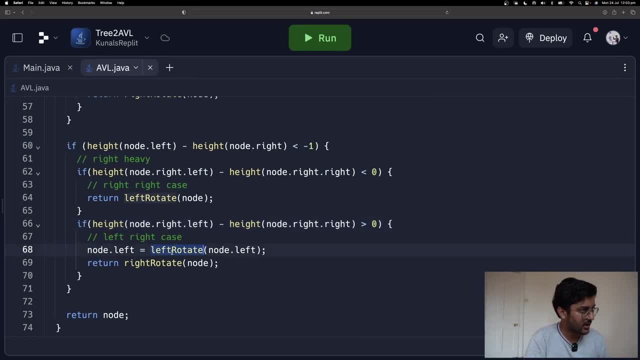 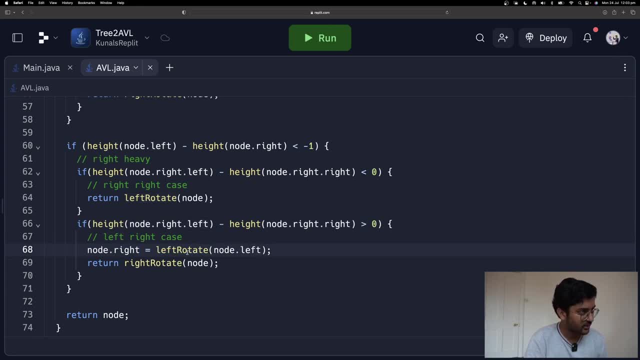 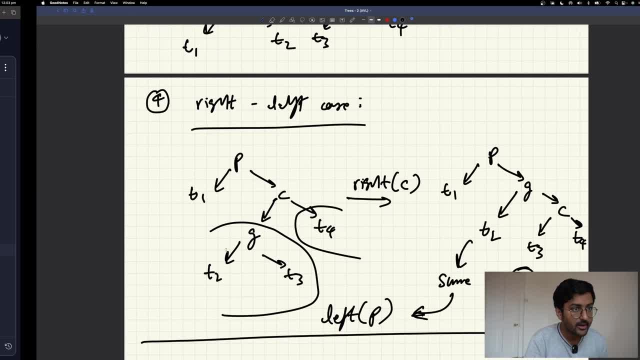 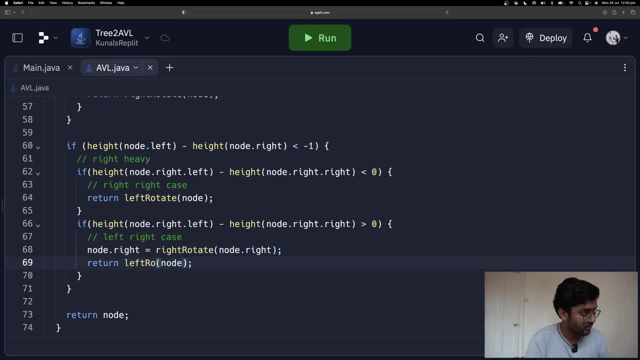 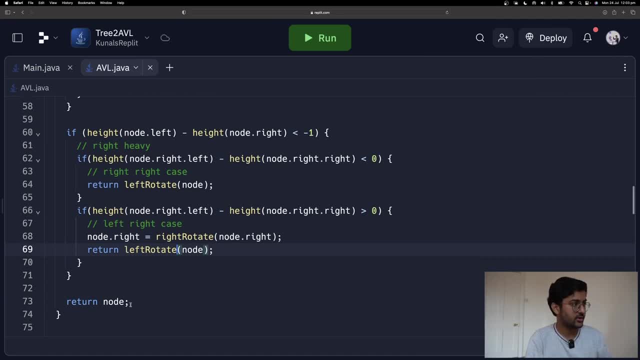 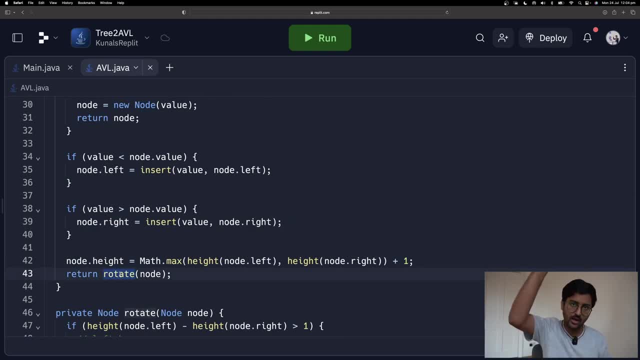 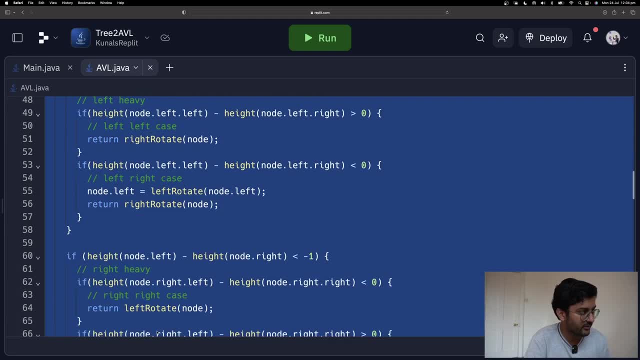 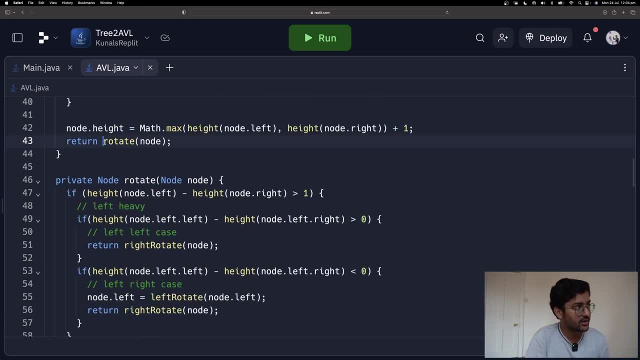 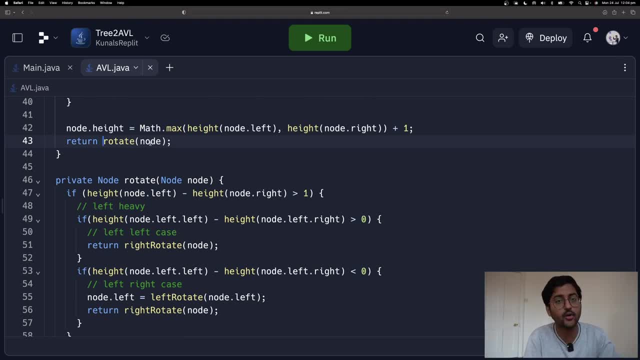 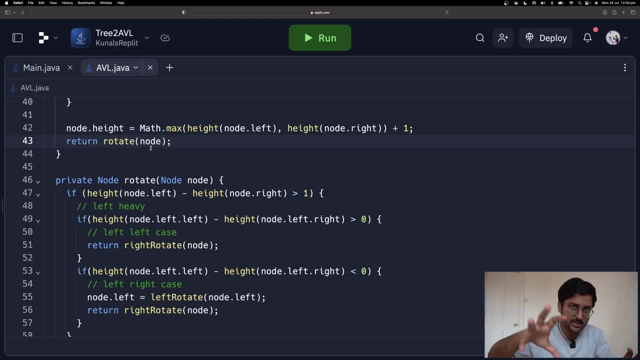 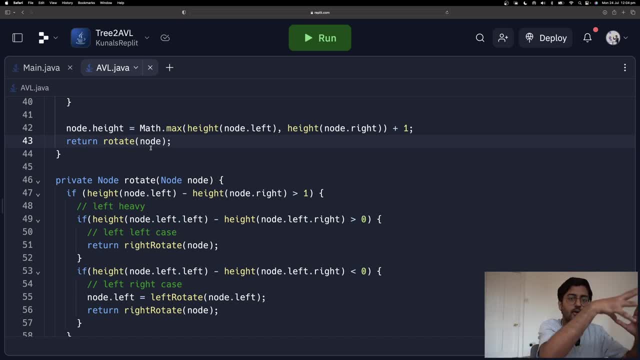 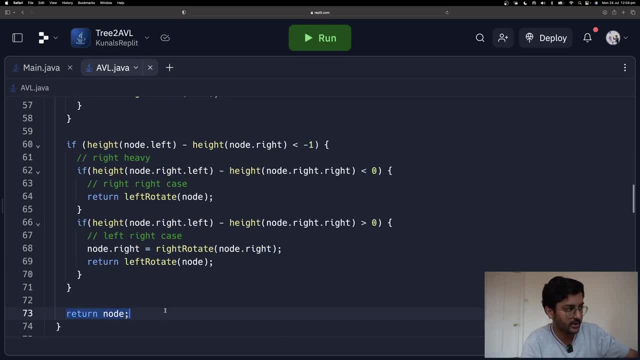 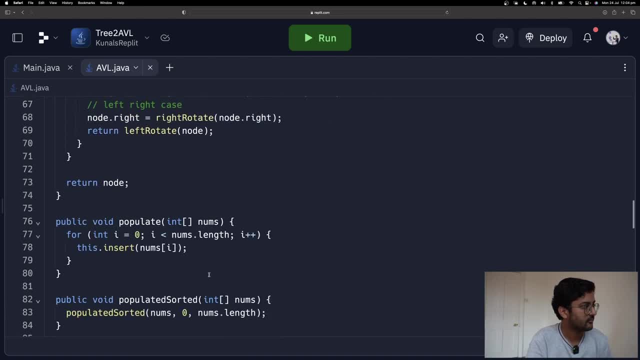 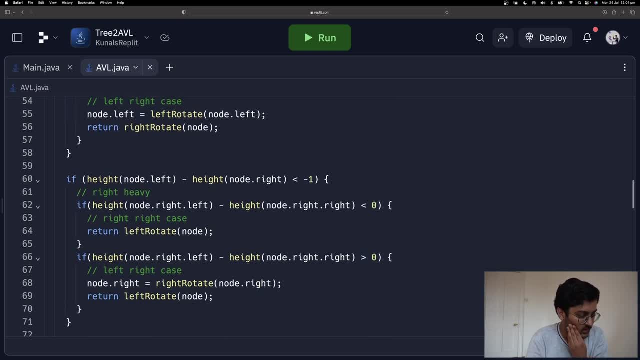 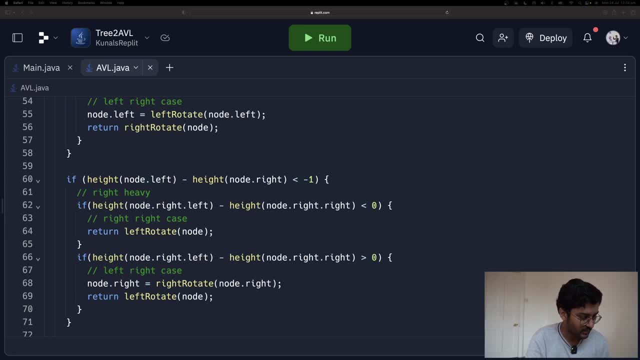 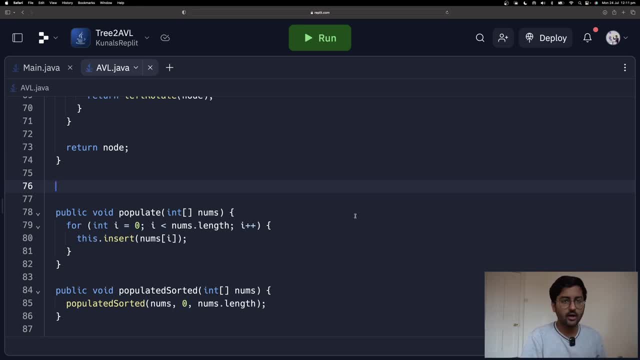 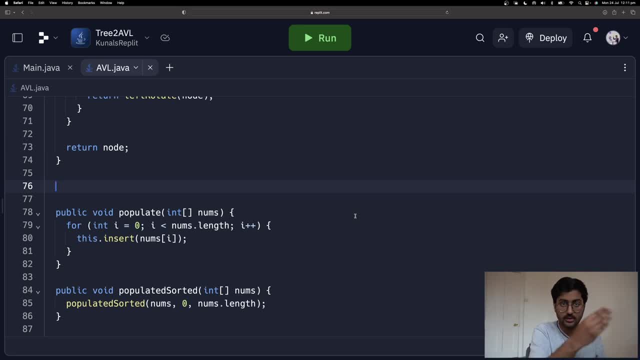 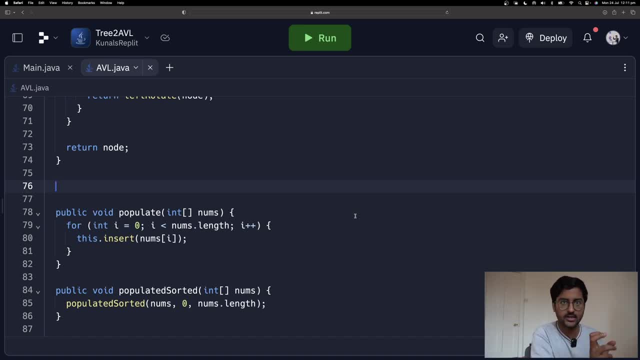 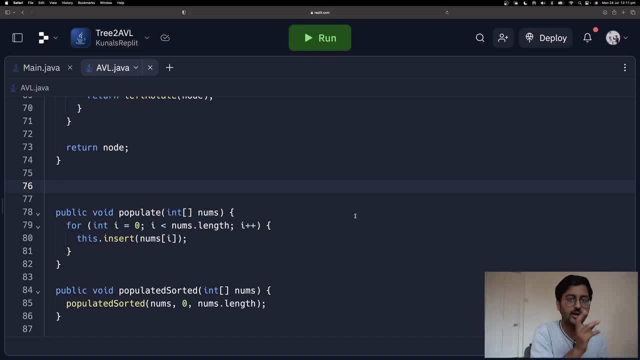 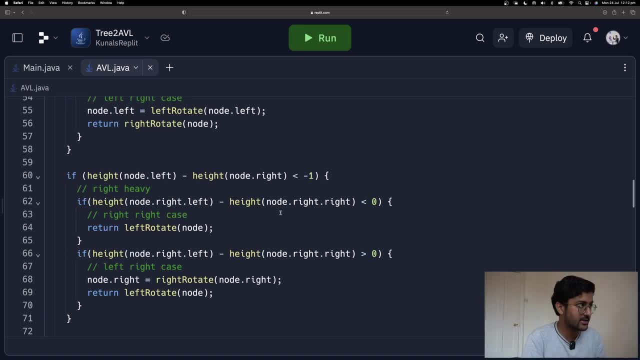 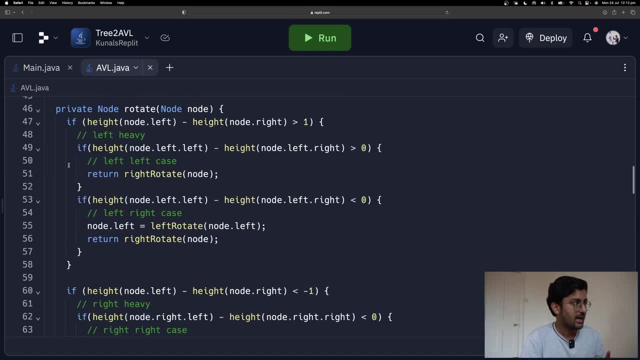 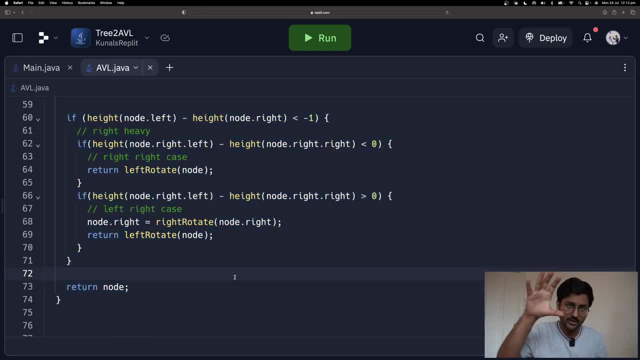 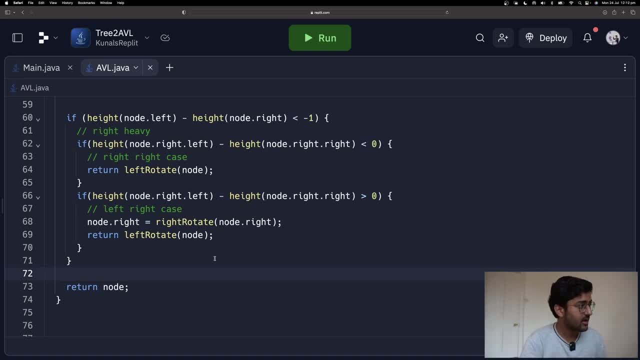 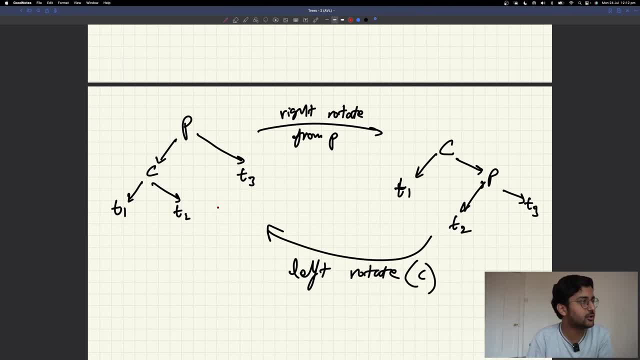 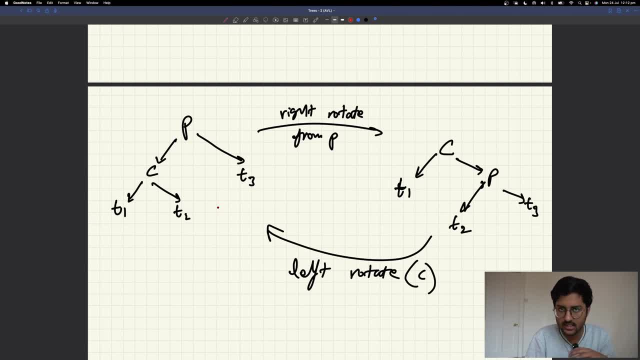 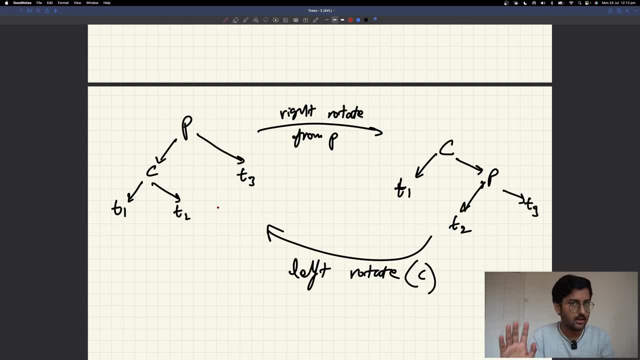 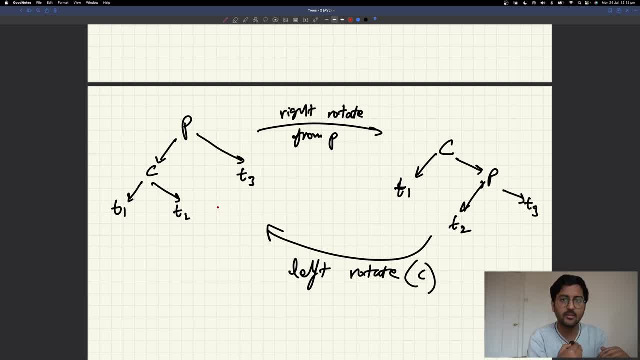 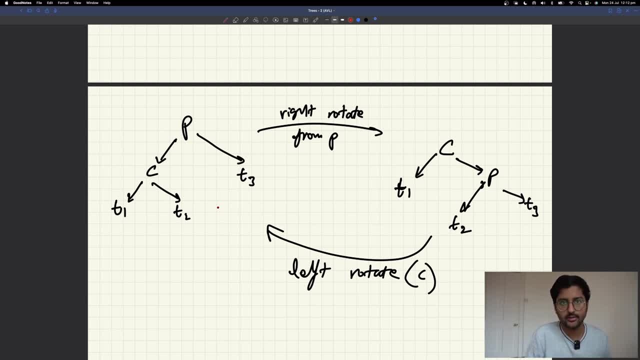 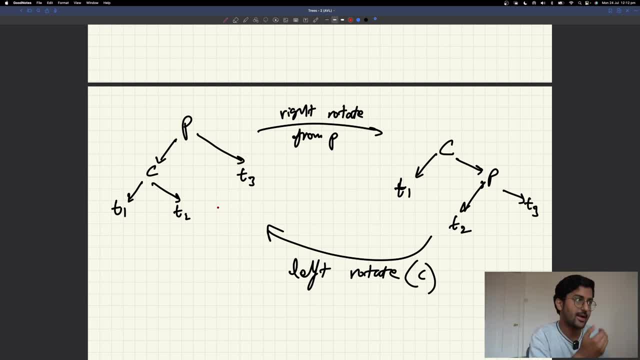 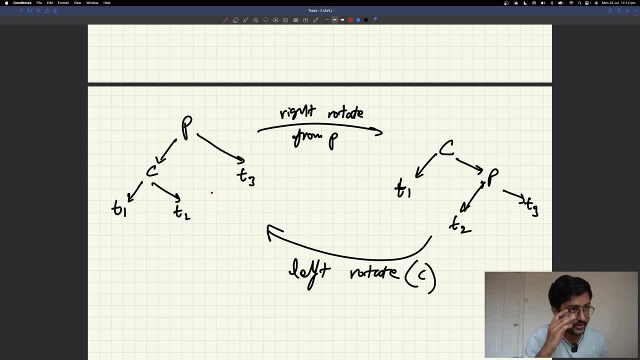 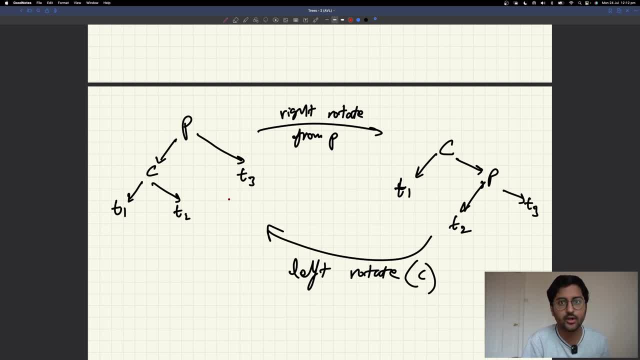 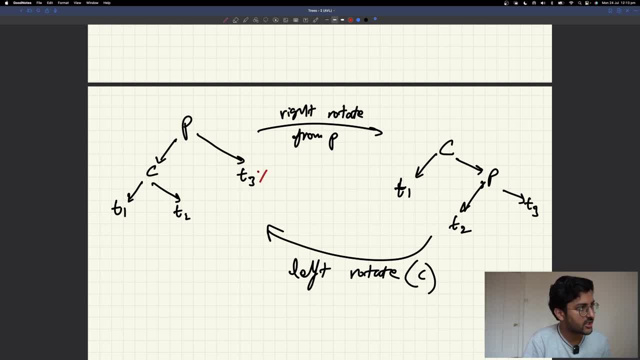 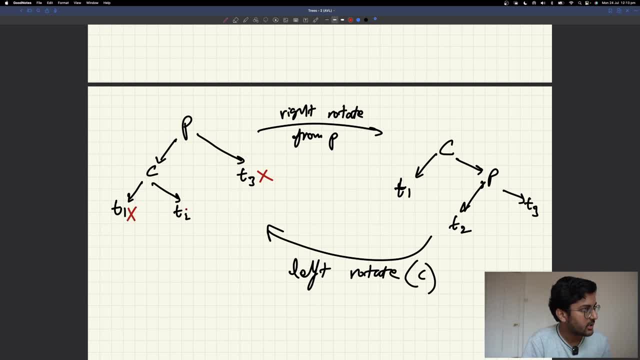 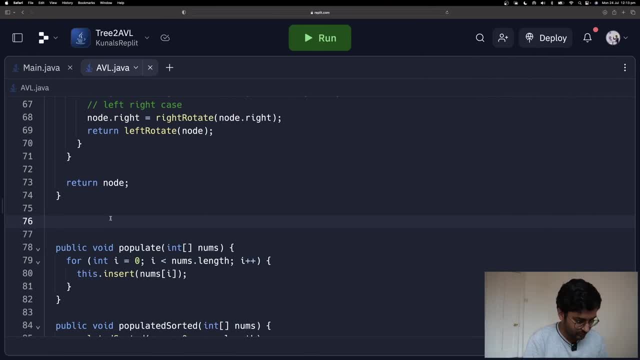 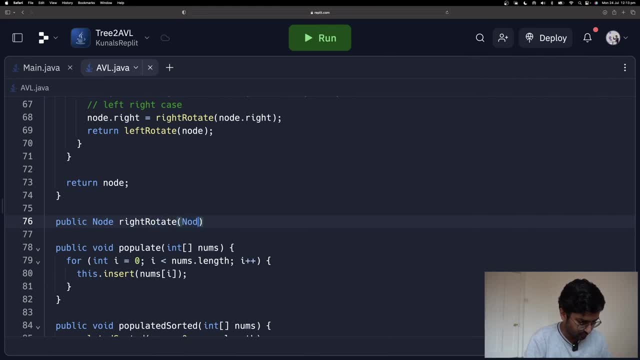 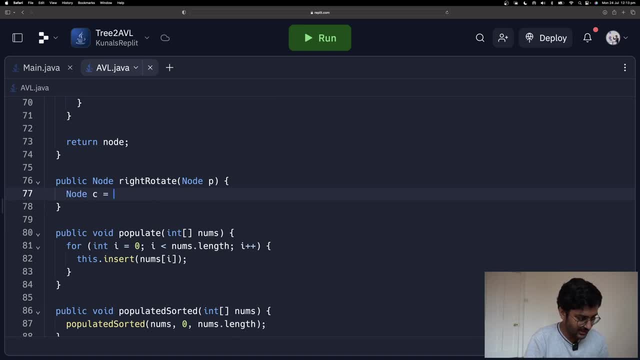 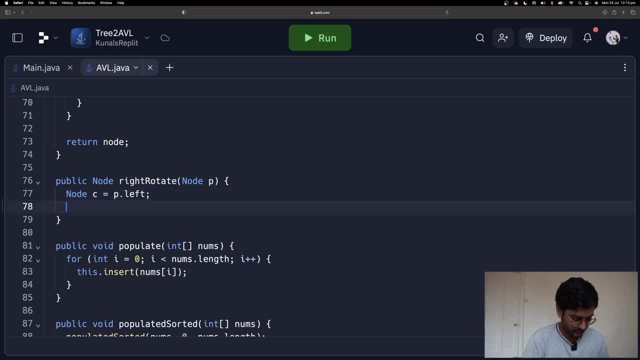 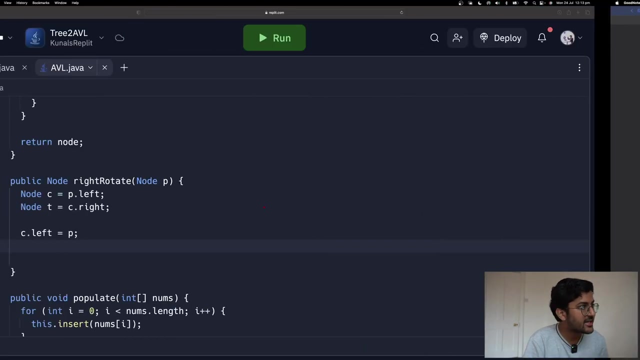 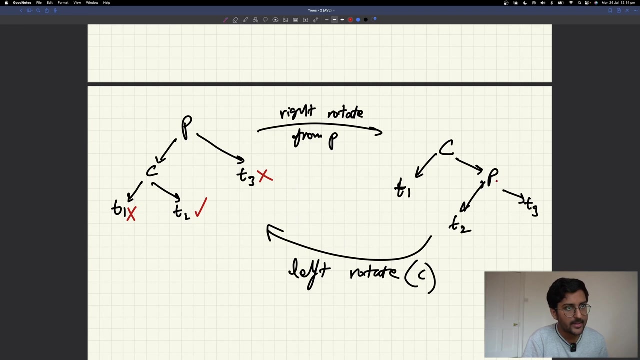 equal to P dot left, dot right now, or C dot right. T is equal to C dot right, T is equal to C dot right. okay, now right rotate. C dot left will become P and P dot left. sorry, C dot right will become P, C dot right will become P and P dot left. 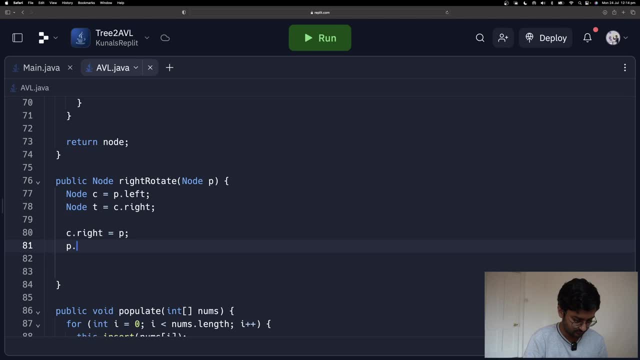 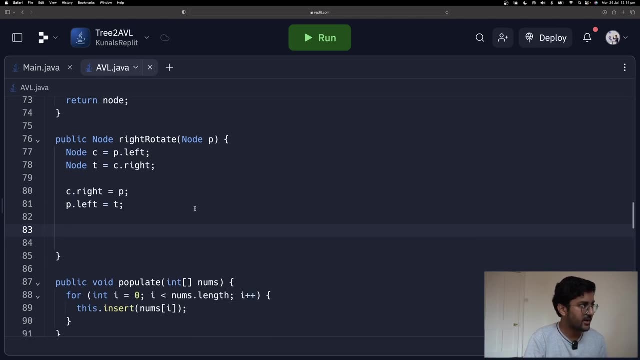 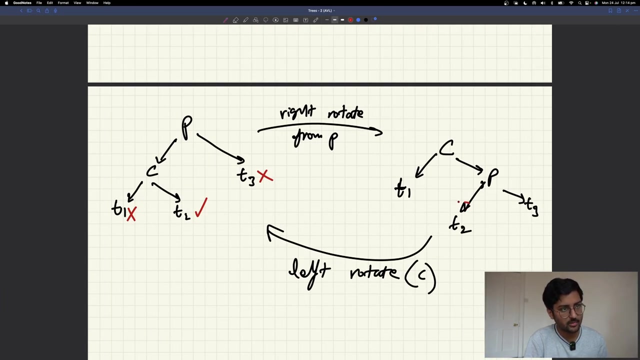 will become T. done, that's it. one last thing you have to do is update the heights now, because C was added above, P was coming down, so update the height. P dot height is equal to math dot max, so new height is going to be equal to maximum of left and right plus 1 for this. 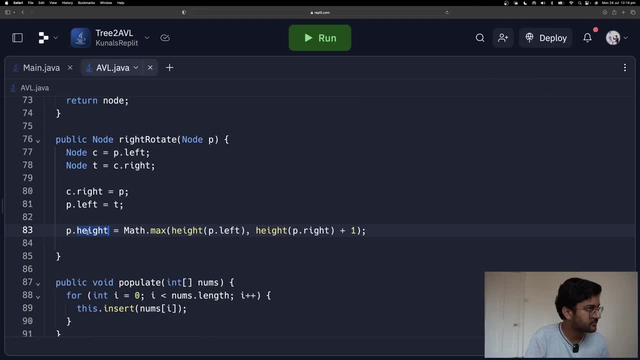 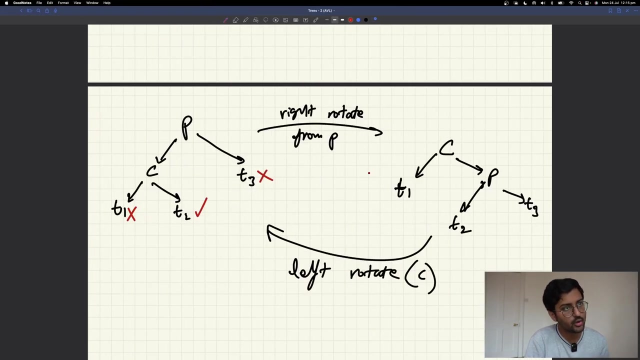 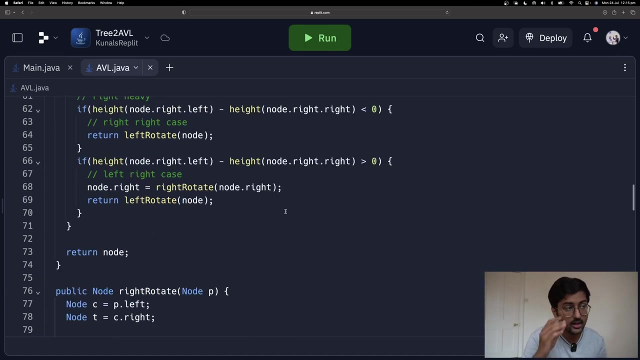 we have done the height formula before, so don't worry about that. similarly, C dot height will be equal to math dot max, C dot left, C dot right plus 1. now what is the new node? new node is C return C. I am telling it again and again: the only intuition problem that you are 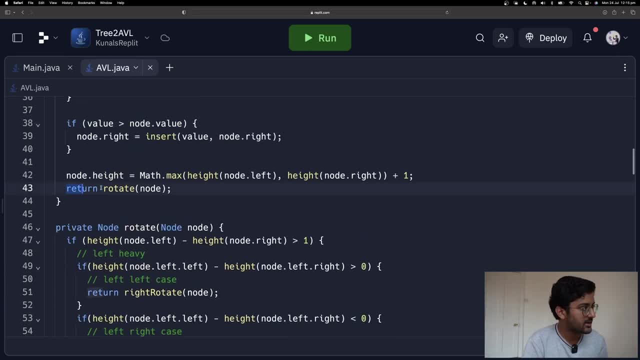 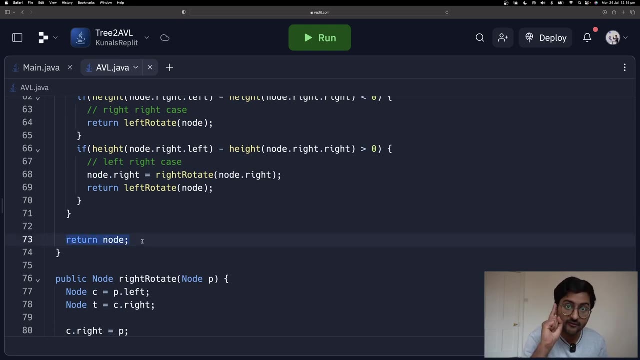 going to have. I know you were having this doubt is over in this line 43. please try to understand that. in original format it was return node. right now also it is return node only C. it is doing nothing but return node. but for that one case in which the sub-tree is unbalanced, it will balance in then return. the node. so new node will be returned. c again value is state transport. players of C and R can control T as shown by the techniques in the program chúng tafsir veo. it means that second node will be operating as a sub-tree. but when T left side isบ ask, tf is be always And it will import then C after T side. tf survey would not change k, that's it. 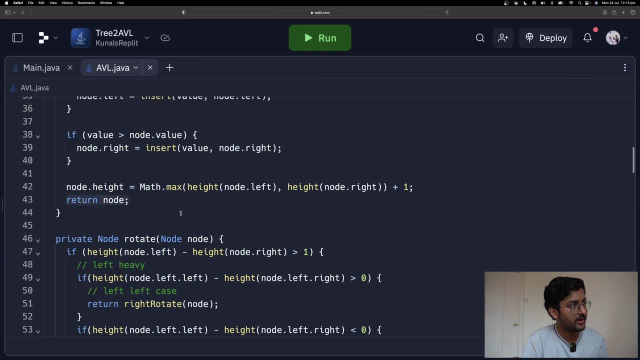 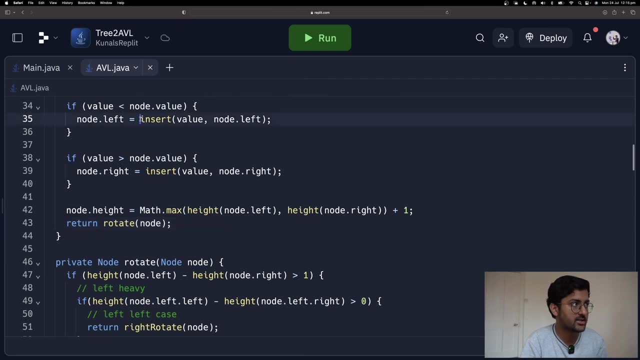 three more limitations. if from T sweep unit in P sii two-data would not change, we would not need the reían think counter like c, and that will be added over here, so it will return then where it will be returned from where it was called, which is somewhere over here, and then that new child will be equal to the node. 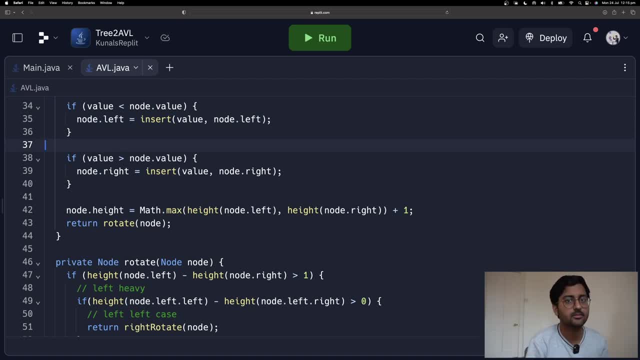 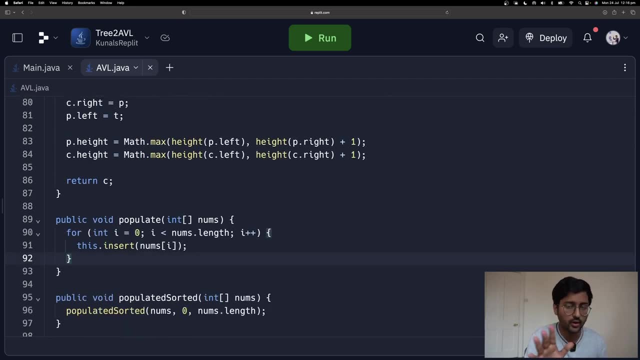 dot left of the above, the one above that one, as i showed you in the example right now when i was writing this code. okay, it was very simple, it is. don't overthink it, it's very simple. i shared it like three, four times. i won't share it again now because then it will get. 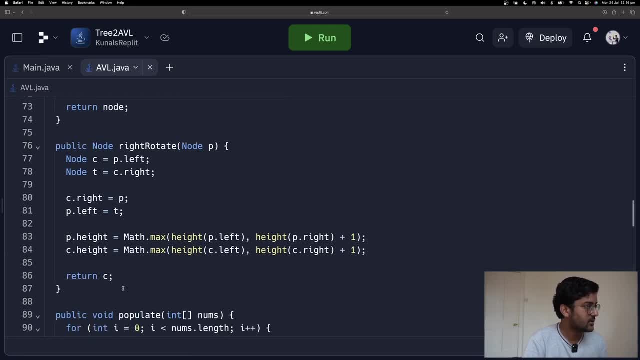 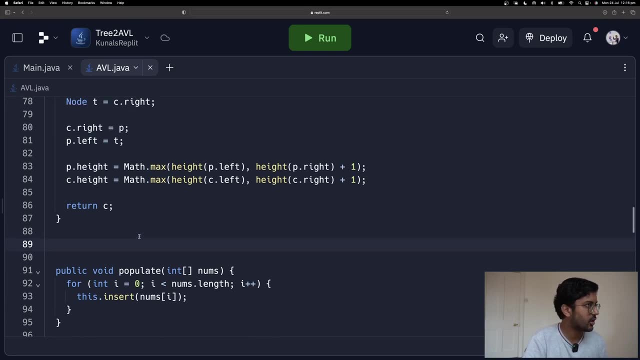 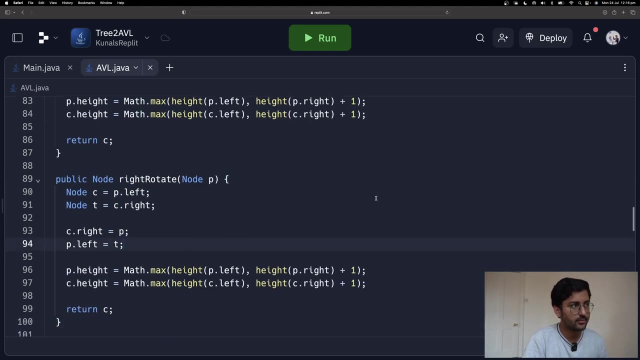 cringy anyway. so i told you where you might get doubt. i solved that doubt. now we can move forward. okay now, left rotate. left rotate is very simple: copy paste. you can still. you can just do the use, the you know um this thing over here. okay, so again, no need to think, i will take in this. 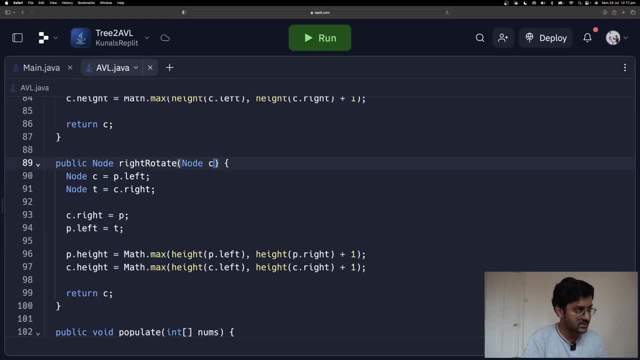 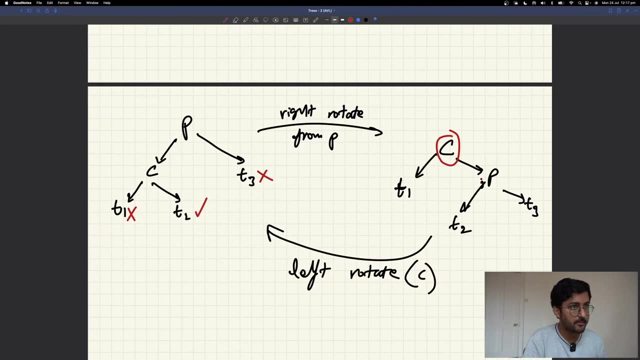 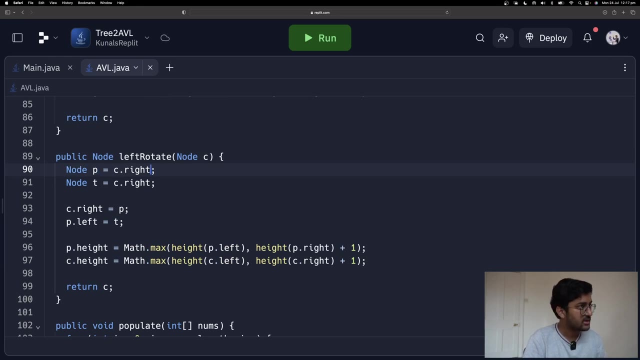 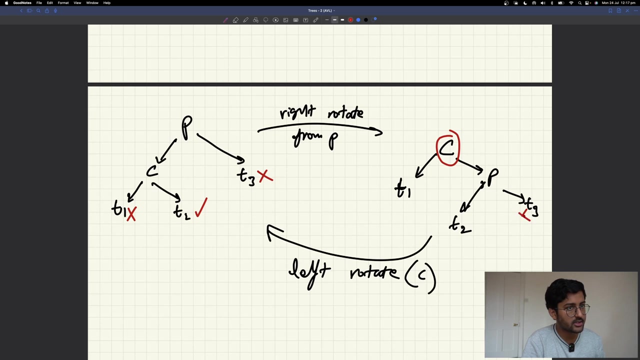 example. only it's saying c. i will have node c over here left rotate. so node p is going to be equal to c dot right. node p is going to be equal to c dot right. and what will remain unchanged? um, p, t3 will remain unchanged. uh, t1 will remain unchanged. t2 will be changed. so c dot right or p dot left. 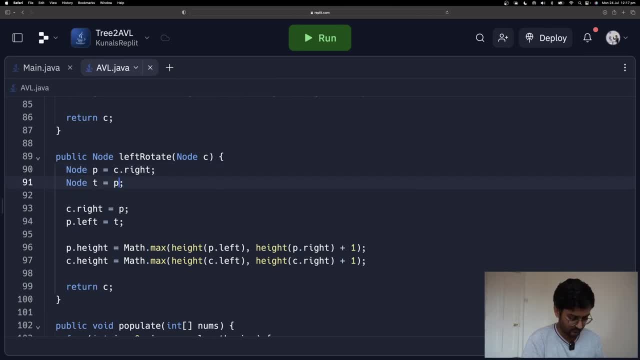 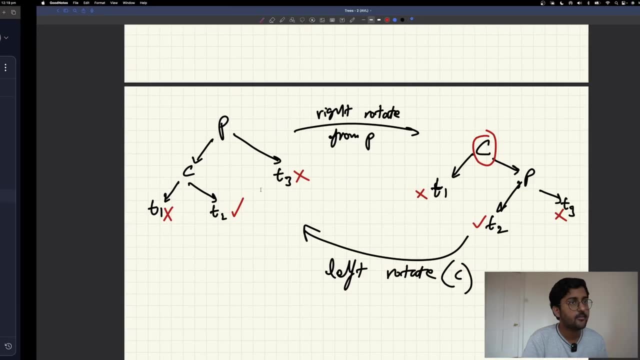 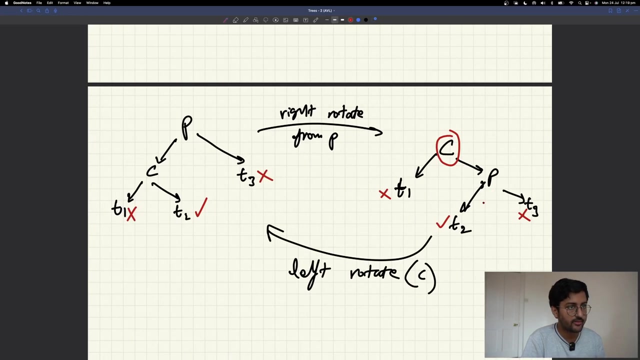 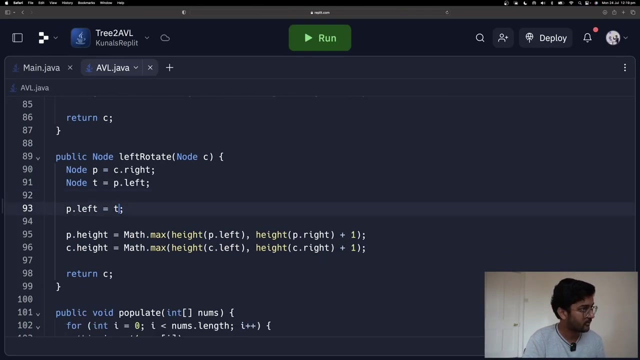 p dot left. okay, okay. so here we have: p dot left is equal my t. and now how to change it? so if i'm changing it left rotate, then p dot left becomes c, no problem at all, and c dot right becomes t, no problem. similarly, p dot height and c dot height. 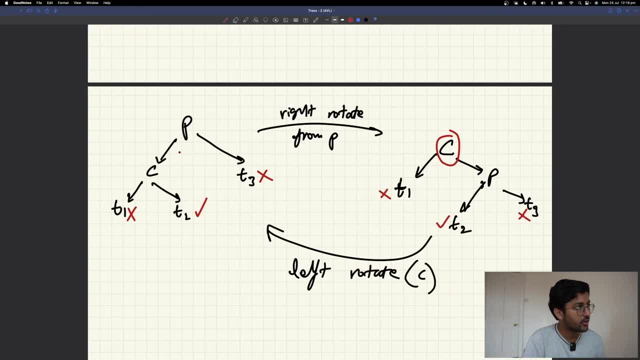 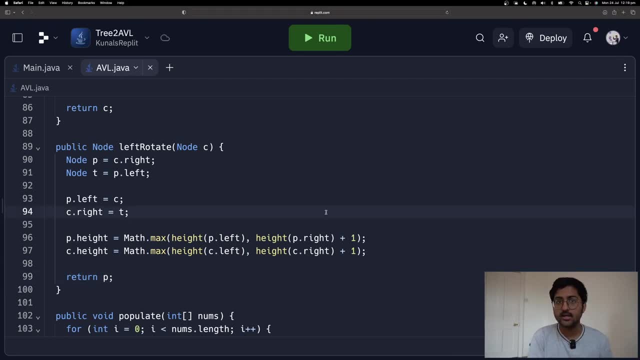 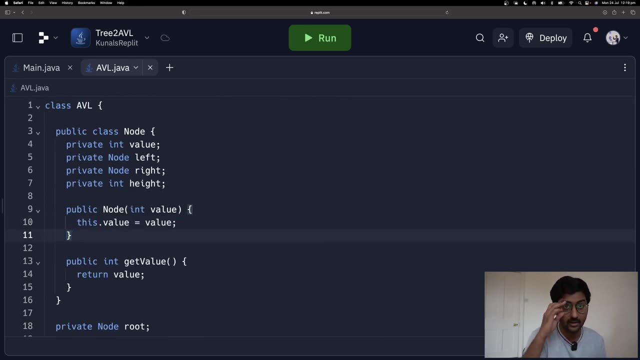 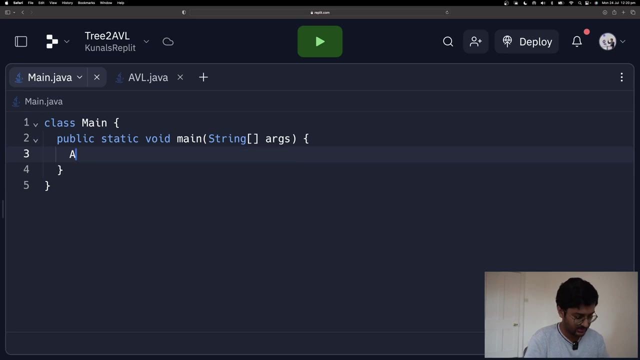 looks good. now new node is equal to p, so i will return p. that's it, avl tree done. um, very cool stuff, simple. right now you can run this. let's try running it. okay, so here in the main function i can write my code. i can say avl tree is equal to new avl tree and let's say i insert: we are trying. 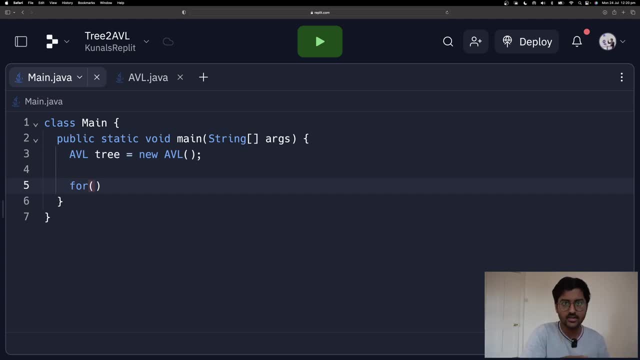 to insert, you know, ascending order. so in binary search state we'll just make a line like i showed in the previous one. uh, int. i is equal to zero, i is less than, let's say, 1000, and i plus plus. i'm going to say tree dot insert i. if i check the 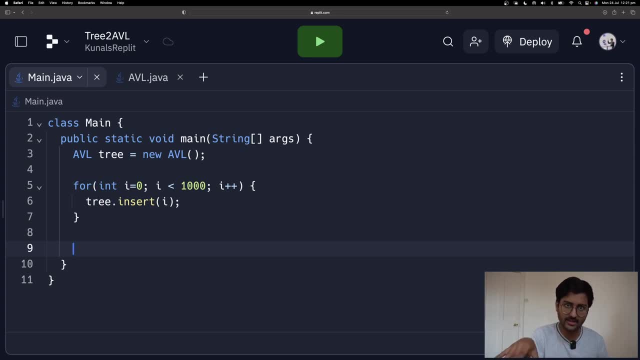 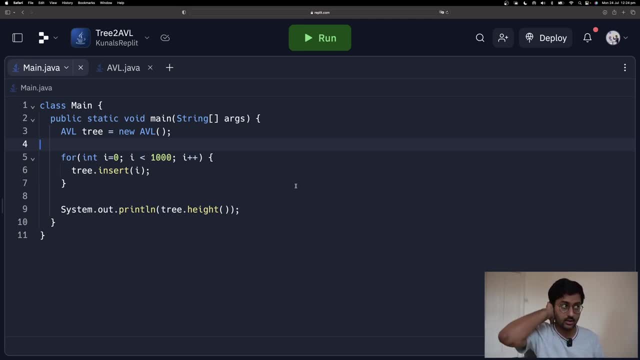 should give me one plus log thousand. so log thousand two plus one three. I inserted thousand elements in a tree in binary search. tree height would be 1 1 1 1. you know, just go right, right, right, right, right, right right, as I showed in. 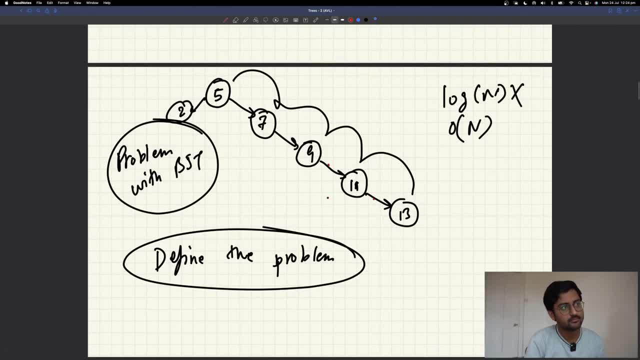 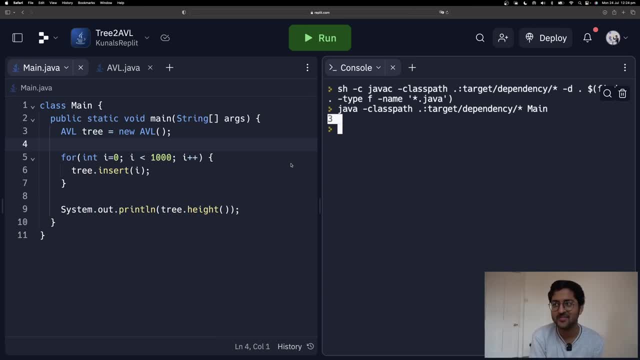 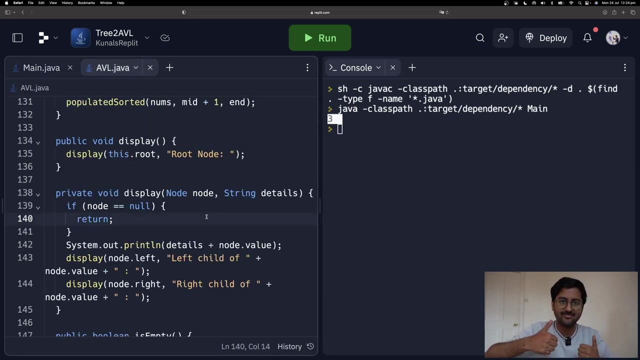 the previous example, this example, but now, no, it's balancing it. that is why always, height will be log of n. simple, very easy, very nice self balancing binary tree is a piece of cake done. okay, you can take a screenshot. share it on social media hashtag: DSA with Kunal. join the. 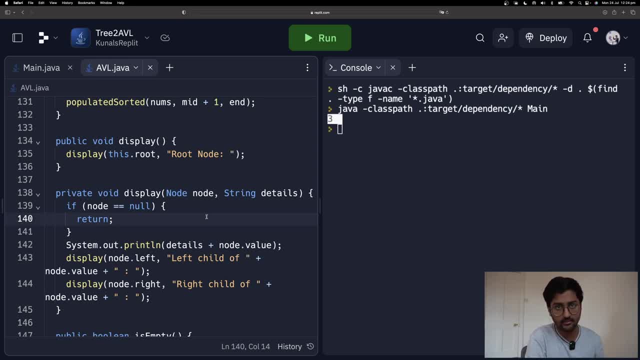 learning public initiative, I'll make tutorials much faster. at least four videos you can accept expect in a month and as the next ones recorded as well, I have to edit those. but I wanted to make sure we do this one first before jumping on to the questions, because these are some of the concepts that are being used.